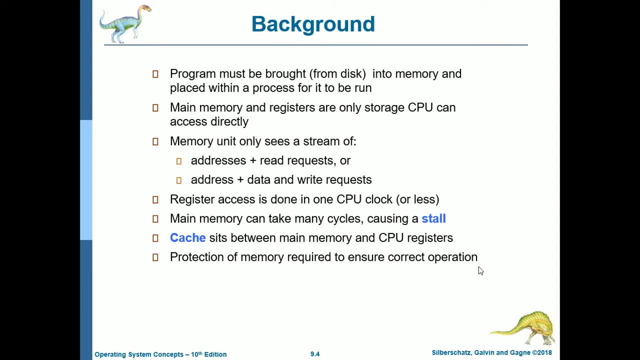 memory causes a stall Because, of course, in comparison with the speed of CPU and main memory, CPU is relatively faster than main memory. So the logic is like this: For example, if you have two people who are working together, then employee A finishes his or her task faster than employee. 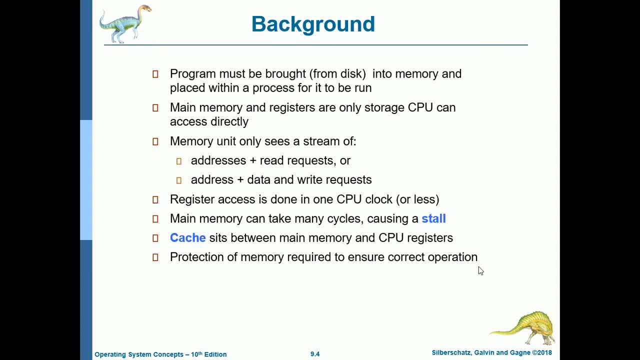 b, then his finished task will be passed to to employee b. so if employee b is slower, so it means that the tasks that are done by employee a will pile up uh to employee b. so that is why, so in in a real world application or for for computer application. so one solution to make your system: 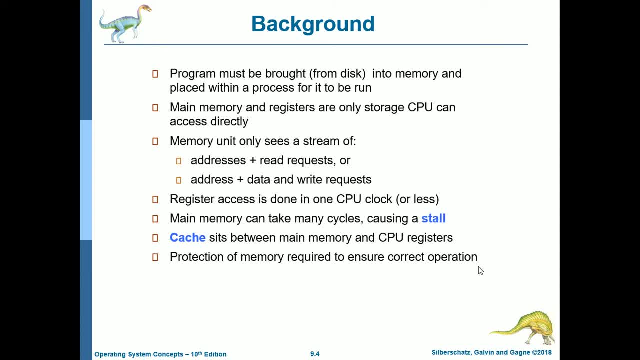 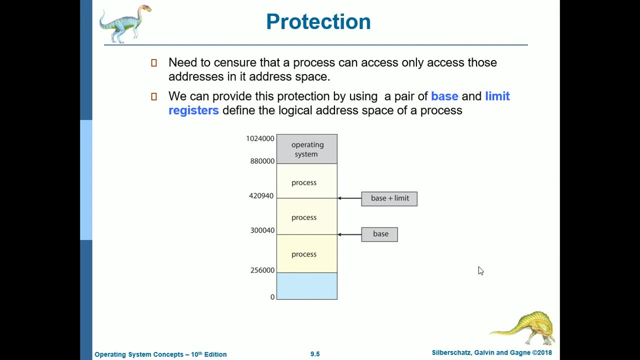 faster is you have to add additional ram or random access memory in your computer. so next is we have cache sits between main memory and cpu registers, and then protection of memory required to ensure correct operation. so this mentioned protection. so need to ensure that a process can access only those addresses in in its address space. so we can provide this protection. 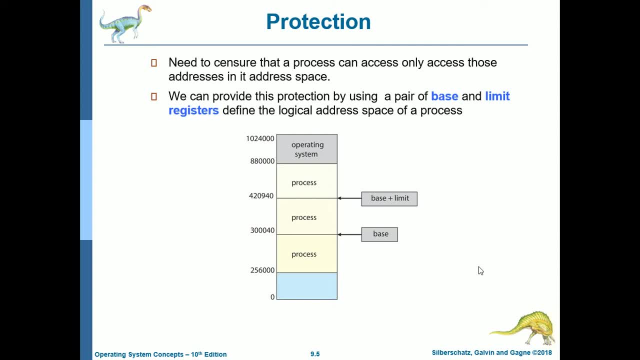 by using a pair of base and limit registers. this define the logical addresses, address space of a process. so, for example, we have this in the memory. so from this is we have the. this is where the operating system is located in memory. so, for example, we have three processes here. so for this, 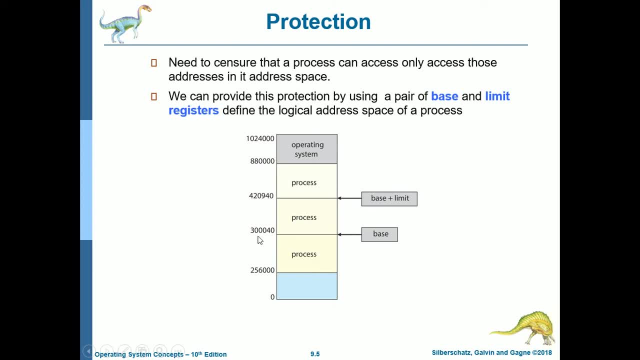 process. so this um three, zero, zero, zero, four, zero, it's it's base, um uh address, and then we have four, two zero nine forty, it's the base plus limit. so it means that the address here, that the base and limit registers defined for that process, is the logical address. 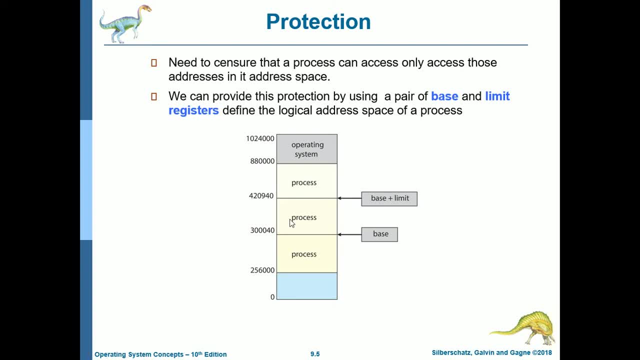 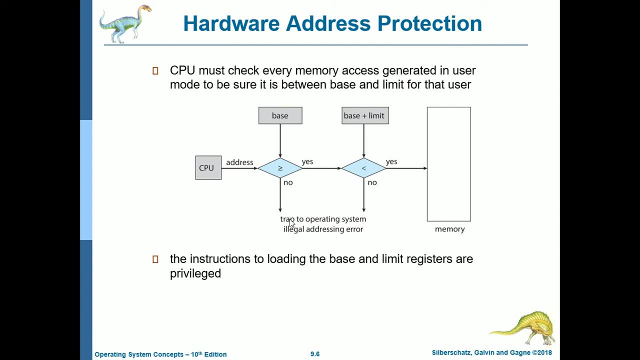 space of a process inside main memory. so next is we have the hardware address protection. so cpu must check every memory access generated in user mode to be sure it is between the base and for that user. so for example, so the cpu, so it will generate an address. so if it is greater than or 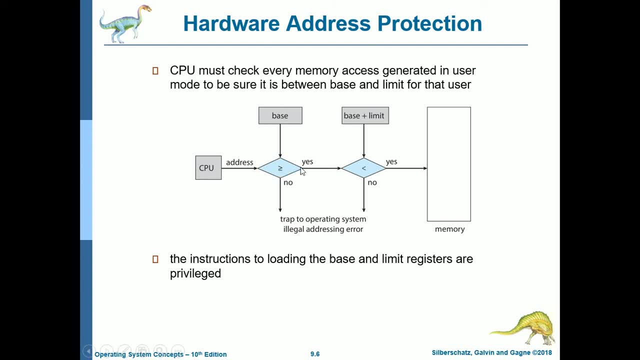 equal to base, so it will continue to add the base plus limit. okay, so let's go first with this one. so if the cpu, that is, um, produced or derived by this uh, the address, uh, derived by the cpu, is what if it is less than the base? so there is a trap to operating system which is illegal. 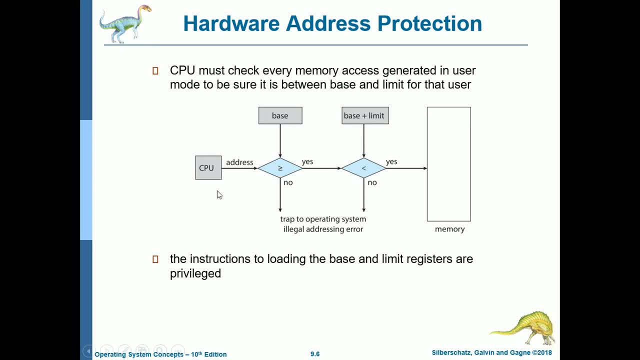 addressing error because, um, the address derived by the cpu is less than the base. but if it's greater than or equal to the base that is produced, so it will continue to add the base plus the limit if it is less than with the limit. so if it's, it's greater than the limit. so again, 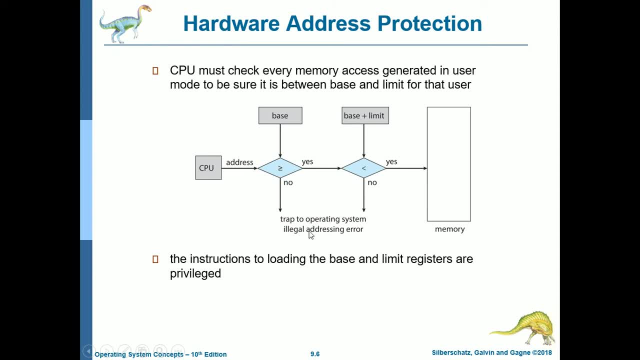 uh, this will have a trap to operating system illegal addressing error. so for it to be loaded to memory, the address should be greater than or equal than the base and less than the base plus limit. so it will be loaded into memory. so the instructions to loading the base and limit registers are privileged. so next is we. 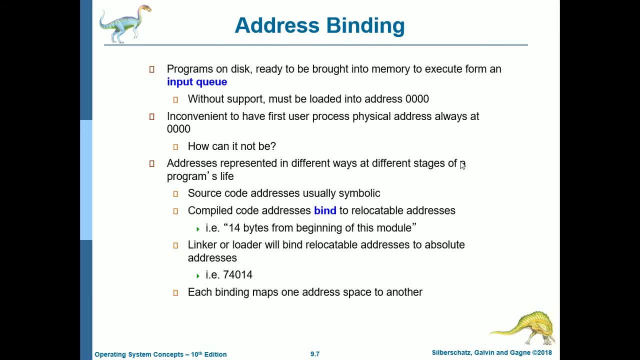 have the address binding. so programs on disk ready to be brought into memory to execute form and input queue, so without support, must be loaded into address zero, zero, zero, zero. okay, it's inconvenient to have first user process physical address always at zero zero. how can it not be because, um, for the addressing of main memory it's not always the same address? 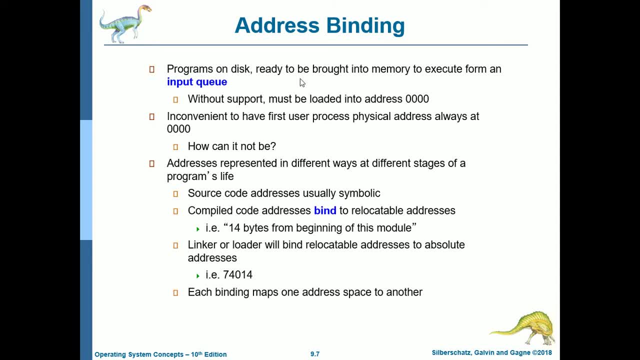 um, the address can be. it's not a really random. at least the free space in memory will be its address. so addresses represented in different ways at different stages of a program's life. so source code addresses, usually symbolic. compiled code addresses- bind to relocatable addresses, such as 14 bytes from beginning of this module, and then linker or loader will bind relocatable. 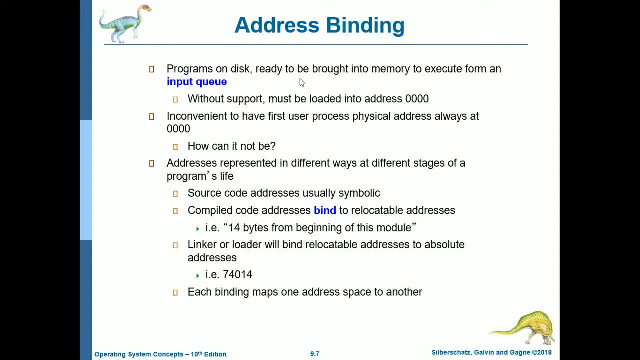 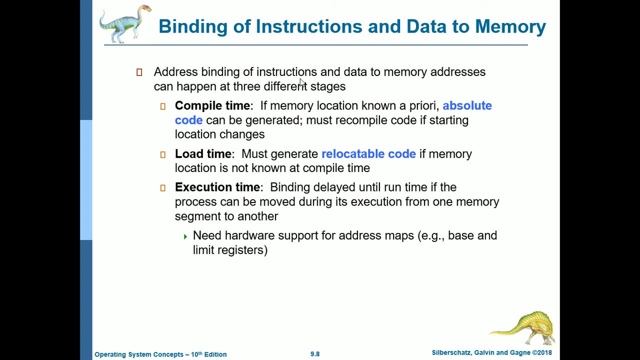 addresses to absolute addresses, so such as 74014, and then each binding maps one address space to another. so next is binding of instructions and data to memory. so address binding of instructions and data to memory addresses can happen at three different stages. so we have compile time if 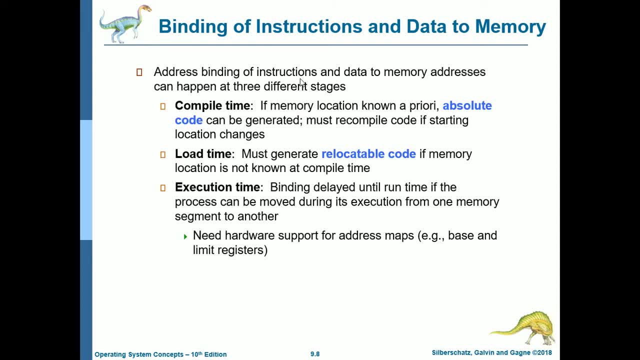 memory location known a priori, absolute code can be generated. must recompile code if starting location changes. so what is absolute code? so this code with bindings to absolute memory addresses. so next is we have load time. must be breadth dash. want generate relocatable code if memory location is not known at compile time. so relocatable code. 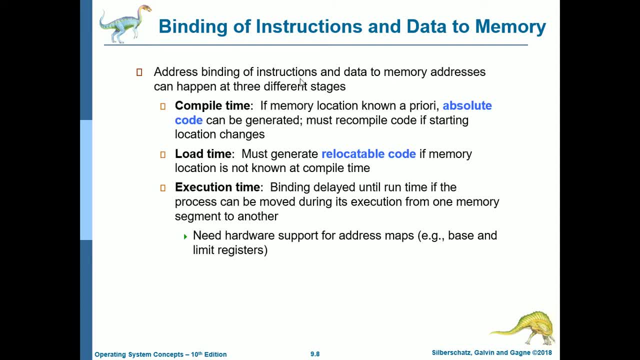 code with bindings to memory address that are changed at loading time to reflect where the code is located in main memory. so next is we have execution time binding delayed until run time if the process can be moved during its execution from one memory segment to another. so need hardware. 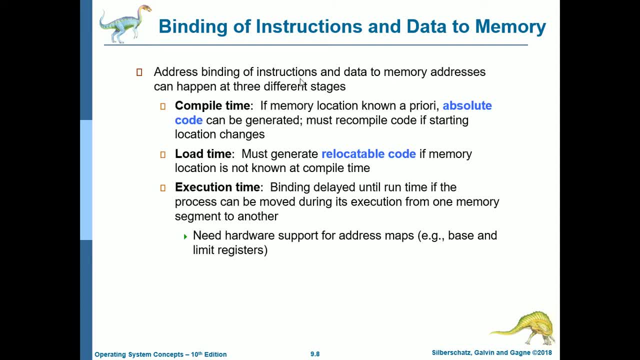 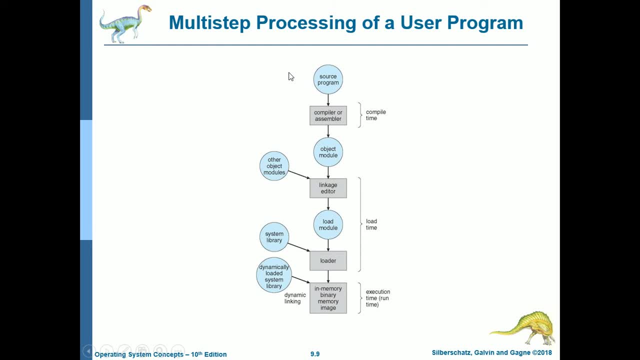 support for address maps such as base and limit registers. okay, as you can already see, this is already shown in the previous lessons, in cooperating systems. so again, our source program. so it will be compiled by the compiler or the assembler, so it is called compile time, the amount. 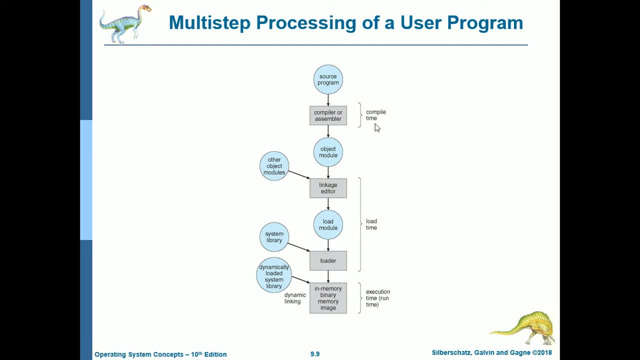 of time it took for the source program to be compiled or assembled, and then its product of the compiler or assembler will be compiled by the compiler or assembler. so it is called compile time, the object module, and then it will be combined to other object modules and there is a linkage editor. 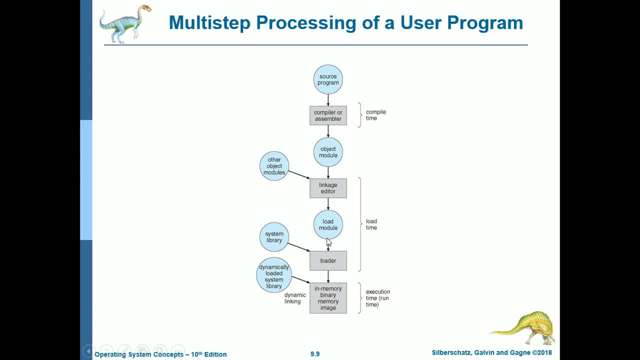 and then it will be the product of the linkage editor, will be the load module, and a load module will be combined with the system library and then it will be loaded in, of course, the loader. so from the linkage editor, the amount of time from the linkage editor to loader, that is the load time. 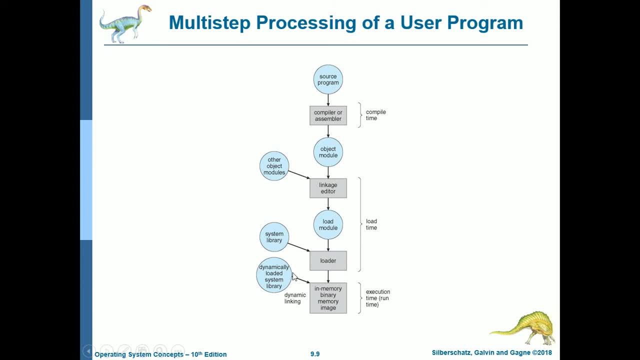 and then for the loader, so the loader will be combined with the system library, and then it will be so from here with in-memory binary memory image, so it will be combined with dynamically loaded system library. so at that that will be the execution or run time, so it uses dynamic linking for dynamically. 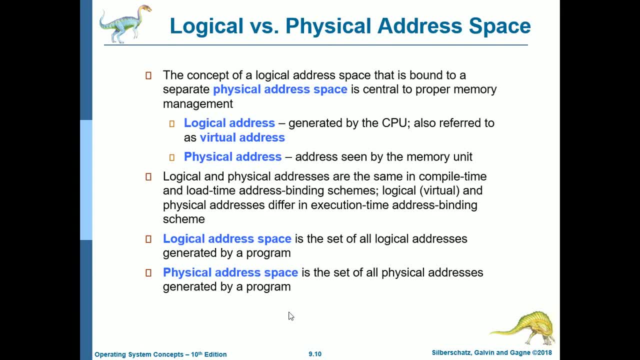 loaded system library. so next is we have logical versus physical address space. so the concept of a logical address space that is bound to a separate physical address space is central to proper memory management. so logical address generated by the cpu, also referred to as virtual address, and the 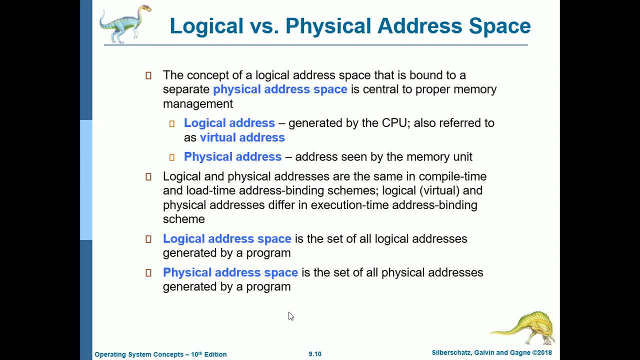 physical address, address seen by the memory unit. so for you to understand the logical and physical address in a real world scenario or analogy, um think of physical address, for example, your home, the house. okay, the physical address is the land where your house is located, the actual land. okay, so that will be the physical address. how about the logical address? the logical? 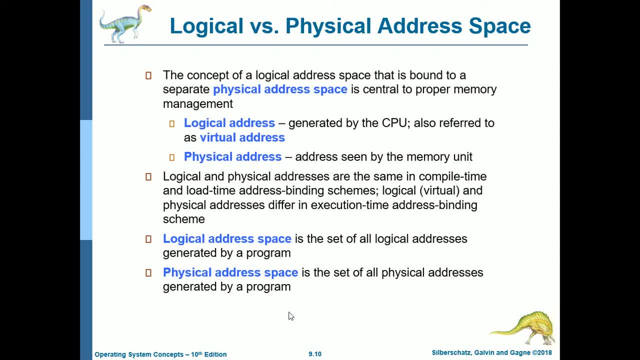 address is the address, for example: uh, if you, if you ordered something online and uh, and the online company or the logistics is asking for your address for for it to deliver at your home, so that address that is indicated um, in the, of course in the address, that is the logical address, so that's. 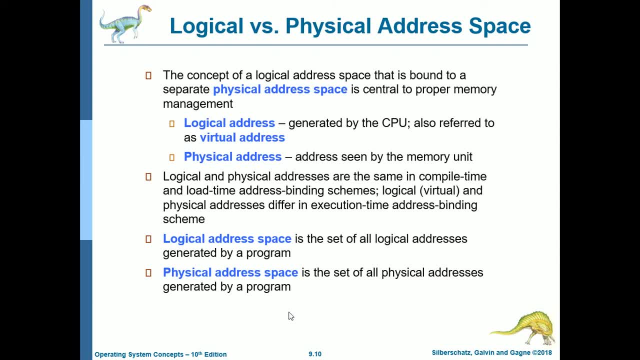 the difference between logical address and physical address. again, physical address, for example, in our house or in our homes, the actual land where our home is situated in the logical address is the, of course the assigned house number, and then what barangay you're in, what province you're in. so 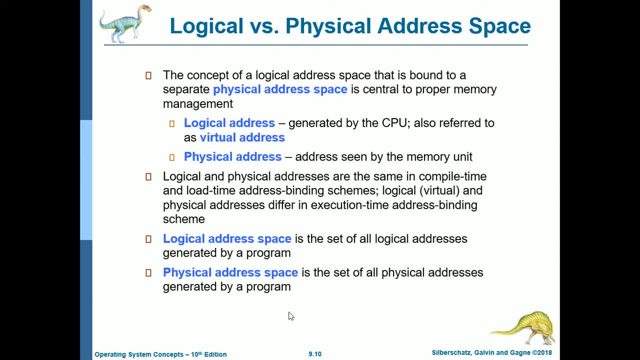 actually logical address can change. what if, for example, um, your barangay has a very prominent fig figure or persons, and then, after a long time, it can be changed, uh, the name of the barangay with the name of that prominent person? so that is all that is possible. so um logical address. 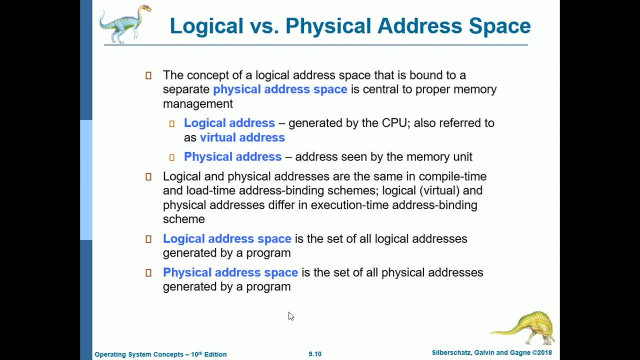 can change. physical address can change also if, for example, your home you will really um going to, um change your location or bring your house to another location. so that's that change of the address. so logical and physical addresses are the same in compiled time and load time address. 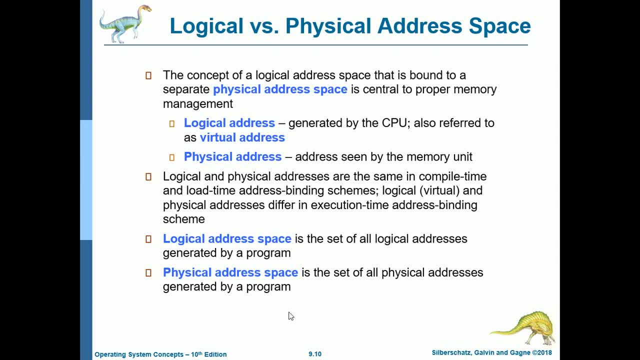 binding schemes. the logical, or virtual, and physical addresses differ in execution time address binding scheme. so logical address space is the set of all logical addresses generated by a program and physical address space is the set of all physical addresses generated by a program. so next is we the memory management unit, or the mmu. 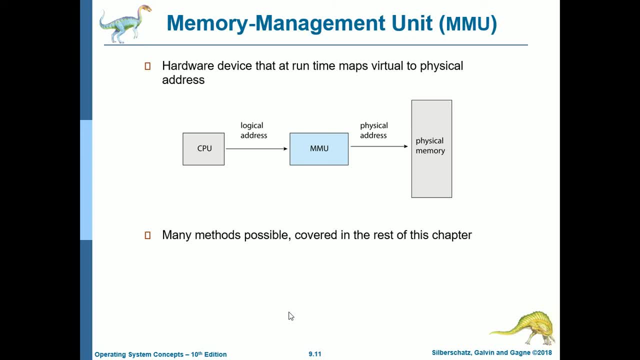 So hardware device that at runtime maps virtual to physical address. So the CPU produces a logical address And then of course, this memory management unit maps the virtual to physical address. It's its responsibility, So it will have its physical address And it will be. this physical address will be put for work. 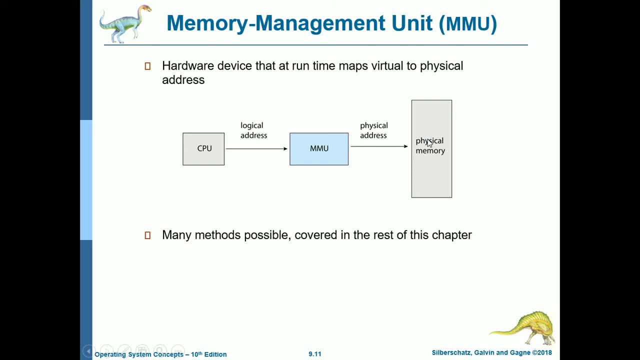 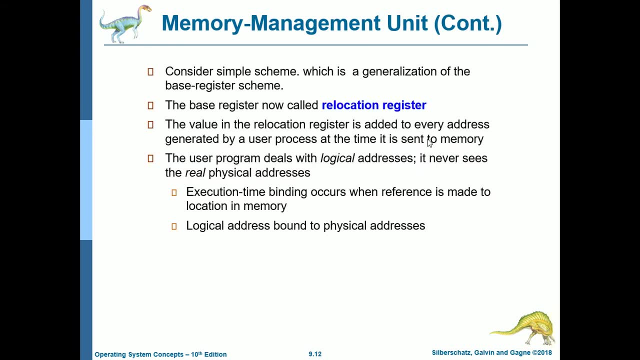 For example, the data will be put in the physical memory. So many methods possible covered in the rest of this chapter. So consider simple scheme which is a generalization of the base register scheme. So the base register now is called a relocation register. So relocation register it is a CPU register whose value is added. 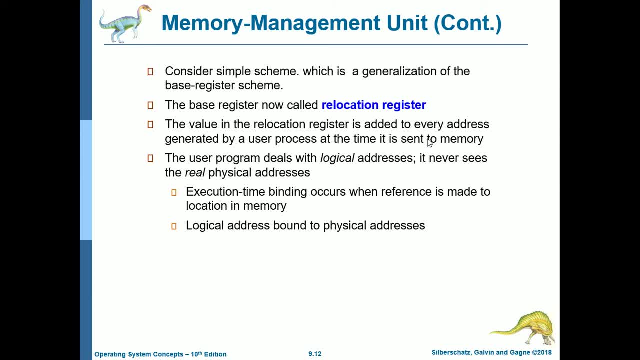 To the base register, To every logical address, to create a physical address, So for primitive memory management. So the value in the relocation register is added to every address Generated by a user process at the time it is sent to memory, And then the user program deals with logical addresses. 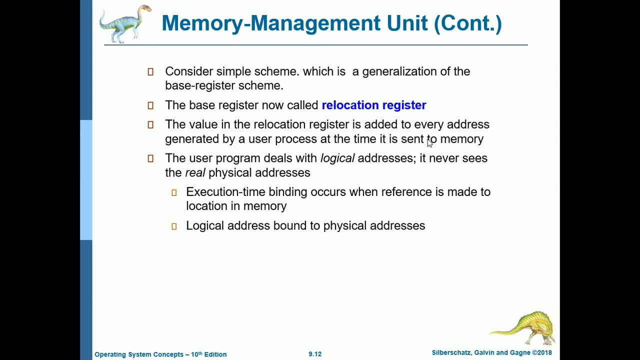 It never sees the real physical addresses. So execution time binding occurs when reference is made to location in memory And logical address bound to location in memory Bound to physical addresses. So we have this illustration of the using a relocation register. So for example, the CPU has a logical address of 346. 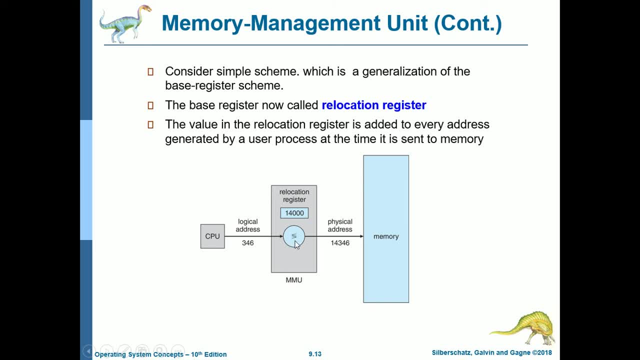 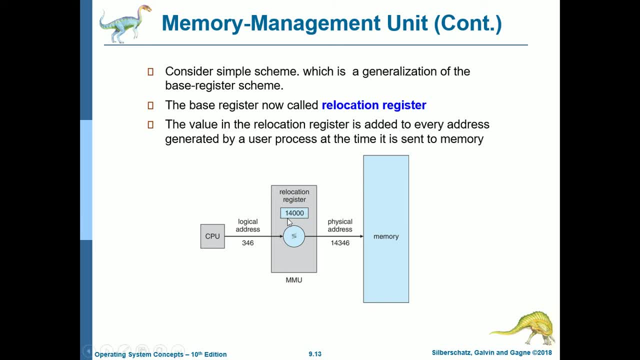 So the relocation address is a logical address. So the relocation address is a logical address. We have 14000, So what we're going to do Of the memory management unit. So the logical address is 346. It will just add the value of the relocation register. 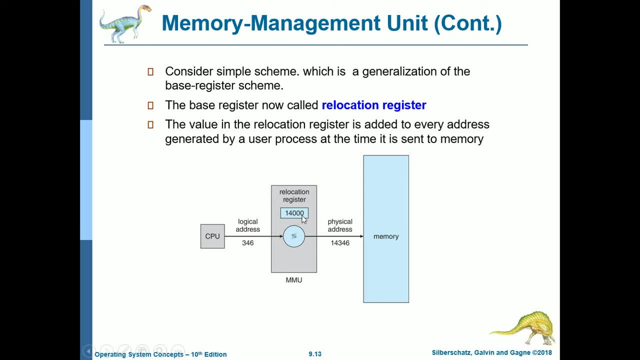 We have 1400, And then so we have 14346, And this will be the actual physical address in memory. So that is how the memory management unit. And then so we have 14346, And then so we have 14346. 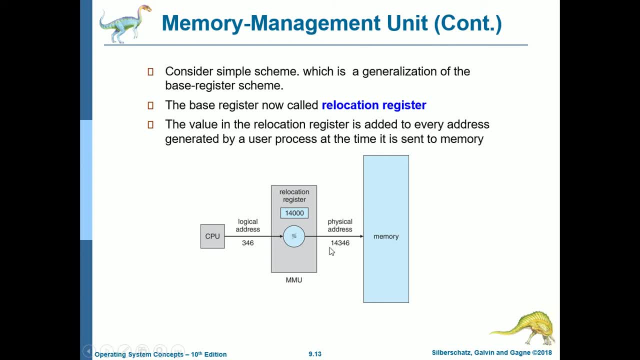 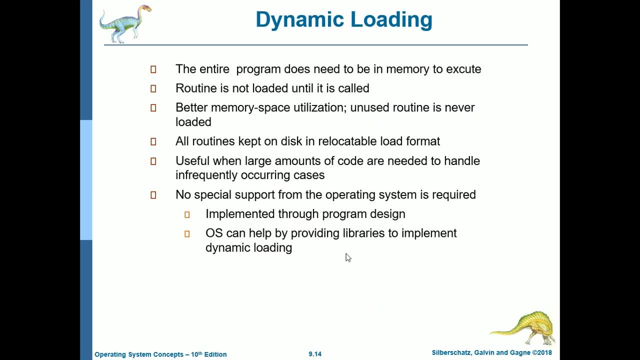 the logical address from the CPU and then and corresponding to its physical address in the main memory. so next is we have dynamic loading, so the entire program does not need to be in memory to execute to execute. so that's a good thing, because not, for example, what if your program is too big for it to 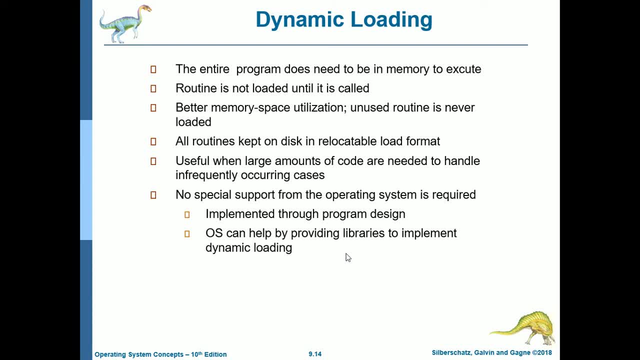 execute. it only needs parts of the program. so routine is not loaded until it is cold. so better memory space utilization. unused routine is never loaded. all routines kept on disk and relocatable load format, so useful when large amounts of codes are needed to handle infrequently occurring cases. so 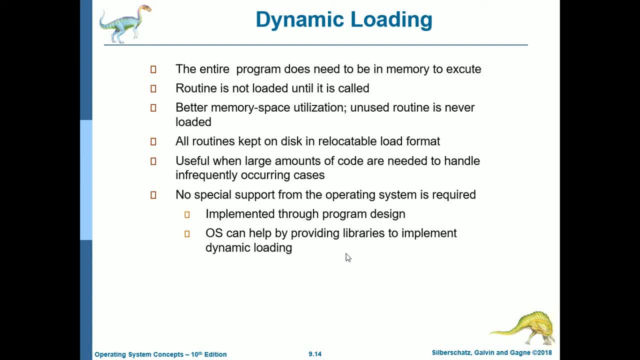 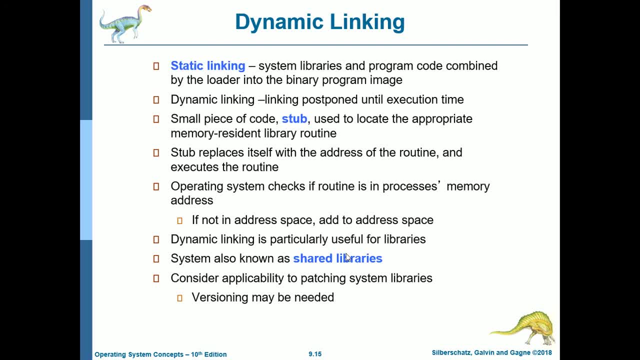 we have dynamic linking, so we have this term, static linking- system libraries and program code combined by the loader into the binary program image and then, if we have the static linking, we also have dynamic linking. linking postponed until execution time. so SME is a small piece of code or stub used to locate the 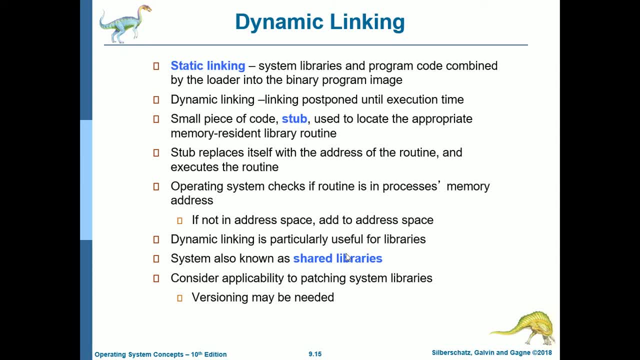 appropriate memory resident library routine. so the stub replaces itself with the address of the routine and it is then used to locate the appropriate memory resident library routine. so the stub replaces itself with the address of the routine and executes the routine and then the operating system checks if routine is in. 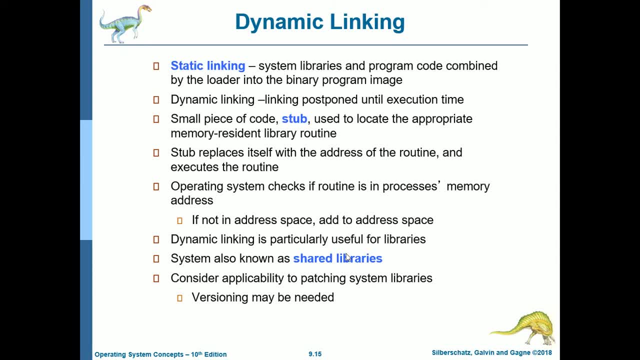 the processes memory address, so if not in address space, add to address space. dynamic linking is particularly useful for libraries, so system also known as the shared libraries for dynamic linking libraries. and then consider applicability to patching system libraries, so versioning may be needed. okay, next is we have the contiguous allocation, a. 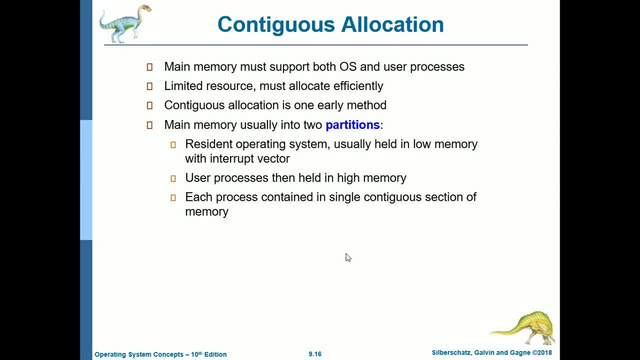 flexibility to patching system libraries, so versioning may be needed. Okay, next is we have the contiguous allocation, So main memory must support both OS and user processes. So of course limited resource must allocate efficiently because our memory is there is a fixed amount or a fixed capacity of main memory. 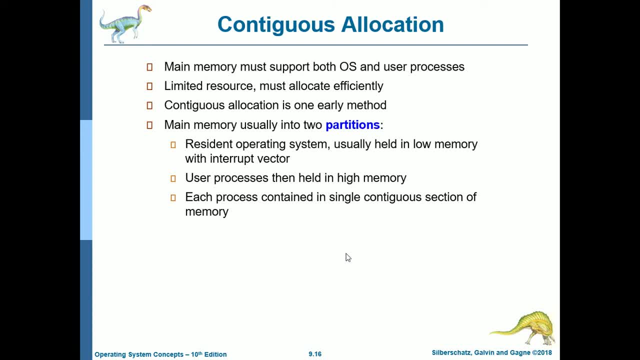 So it should allocate the data or the programs which will be using the space for the main memory must be allocated efficiently, And then contiguous allocation is one early method. So main memory usually into two partitions. We have the resident operating system, usually held in low memory with interrupt vector. 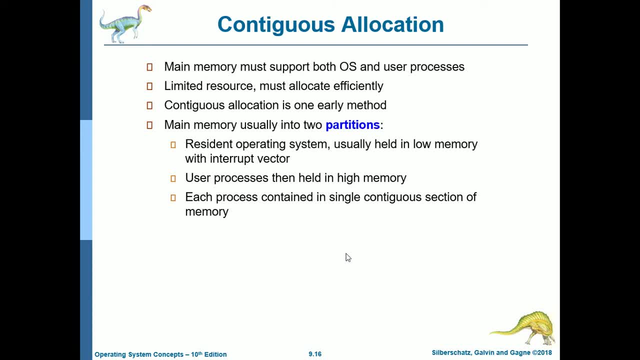 And the next user process is then held in high memory. So each process contained in single contiguous section of memory. So meaning of contiguous is they are in one place. Okay, they are adjacent to each other. That is what is mean with contiguous allocation. 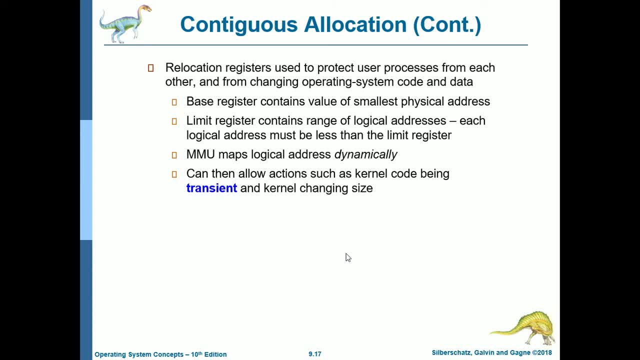 So relocation registers used to protect user processes from each other and from changing operating system code and data. So base register contains value of smallest physical address. So that's why base plus limit address And then limit register contains range of logical addresses. 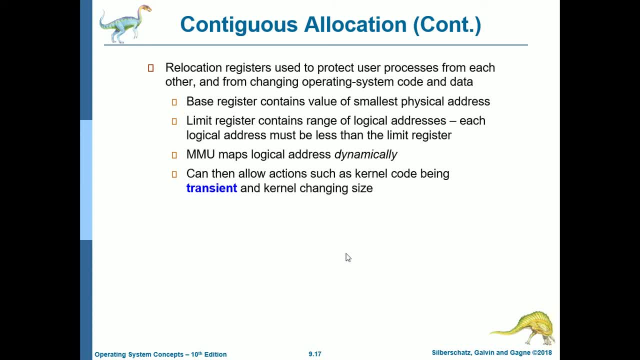 Each logical address must be less than the limit register. So, as a result, we have a limit register, As we already discussed in the previous slides. So base is the smallest physical address, while the limit- the logical address- must always be less than the limit register. 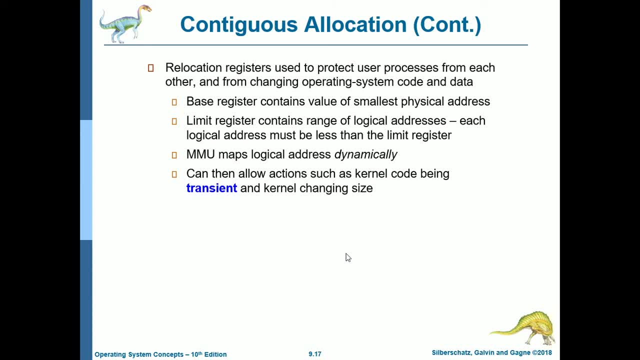 So the MMU maps logical address dynamically can then allow actions such as kernel code being transient and kernel changing size. So kernel being transient means it's temporary. So because kernel change its size, So kernel change its size over time. 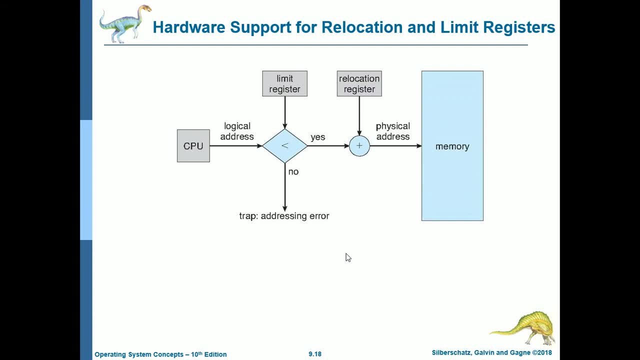 Okay, next is we have illustration of hardware support for relocation and limit registers. So again, this is using relocation registers, So the CPU will have or produce logical address. So if it's greater than the limit register, so it will have a trap and addressing error. 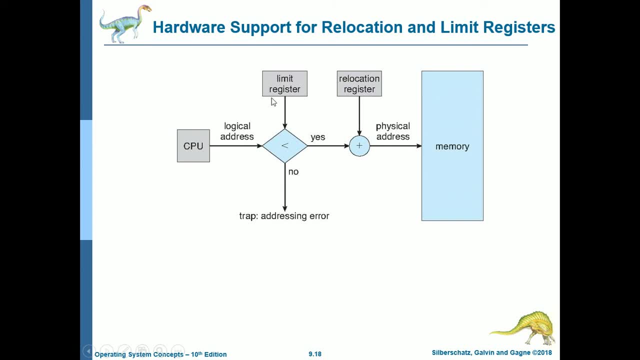 But if the logical address is less than the limit register, Then from the relocation register it will add the value of relocation register in the logical address and it will produce a physical address which corresponds to the physical address in the memory. Okay, next is we have variable partition. 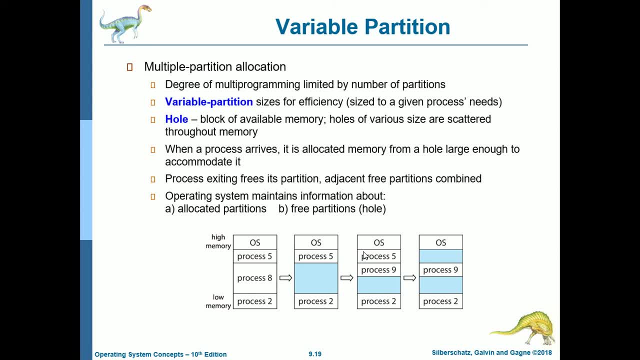 So multiple partition allocation, So degree of multi-programming limited by number of partitions, Variable partition sizes for efficiency Size to a given process needs. So what is a hole? Block of available memory. Holes of various sizes are scattered throughout memory. 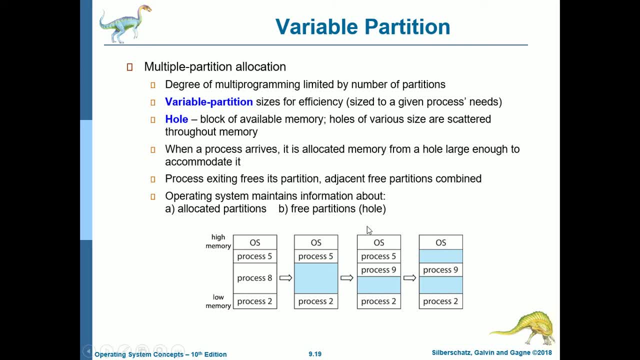 So this is a hole. this is a hole, So these are holes. When a process arrives, it is allocated memory from a hole large enough to accommodate it. Process exiting frees its partition adjacent free partitions combined So adjacent, So this will be combined to have a memory. 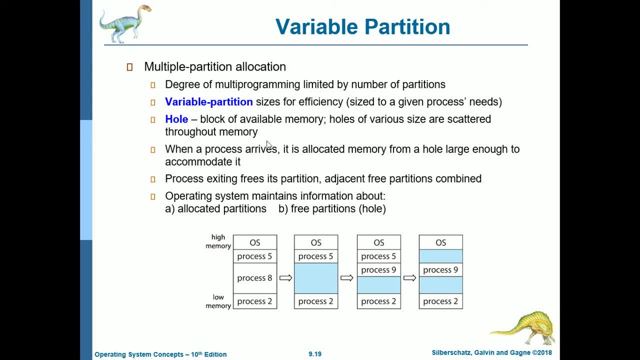 A free memory space, And then operating system maintains information about the allocated partitions, And then we also have free partitions, which are the holes, For example. so for memory we have three processes: 5,, 8, and 2.. 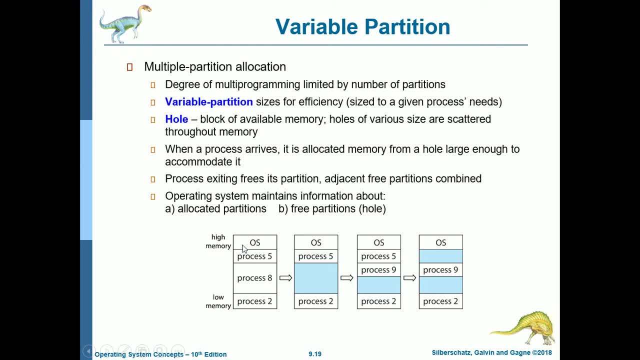 And then, of course, fixed memory location for OS. What if process 8 has already finished its execution? So it will be swapped out from the memory. So the space that process 8 leaves, that will be the hole. And then what if next is process will be executed. 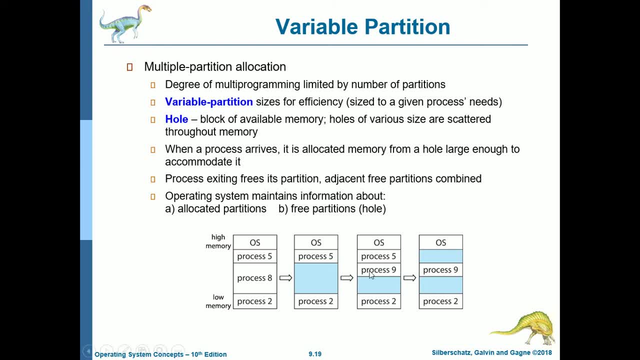 So it will be loaded in memory, So this will be put on the hole as we can see, But of course there's still additional or still a hole here, a space. And then what if process 5 has finished its execution? 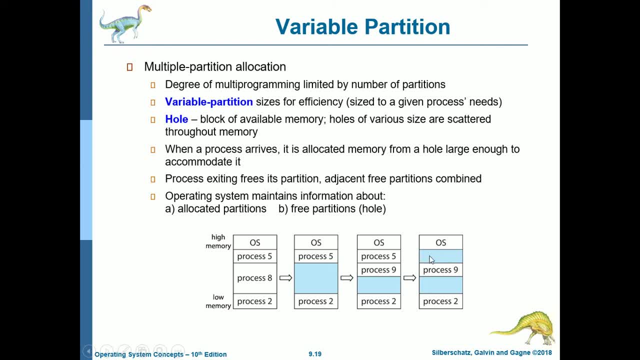 So we have. it will leave again another hole In which the process 5 has left, So we have two holes here. So that is what is the meaning is: there is always have a free partitions or hole after each processes finished its execution. 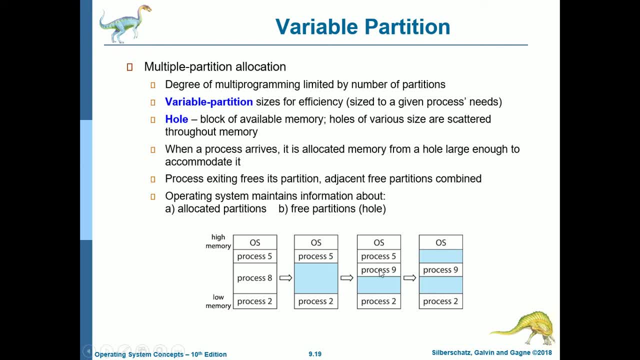 So, for example, what if process 9 has finished first and then process 5 is still here? So this it is. for example, this will be a hole. So it is said here that adjacent free partitions will be combined. 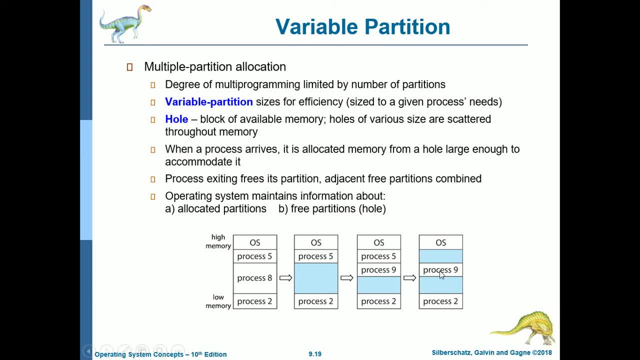 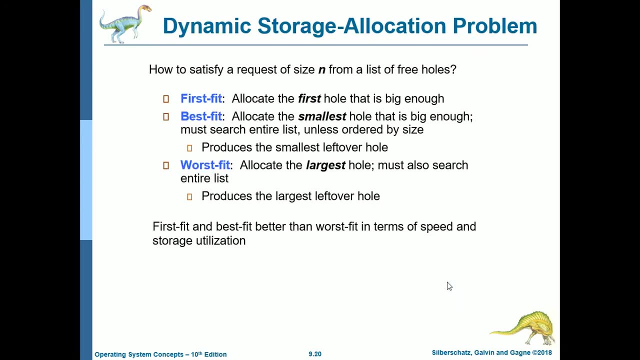 For this it cannot be combined because we have still process 9 here, that is, executing Once process 9 will be finished. So the three holes will be combined, since they are adjacent free partitions. Okay, next is we have the dynamic storage allocation problem. 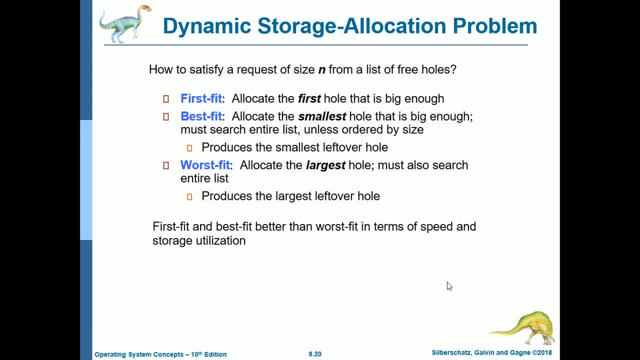 So how to satisfy a request of size n from a list of free holes. So we have three suggestions. So we have first fit allocate the first hole that is big enough, And then we also have the best fit Allocate the smallest hole that is big enough. 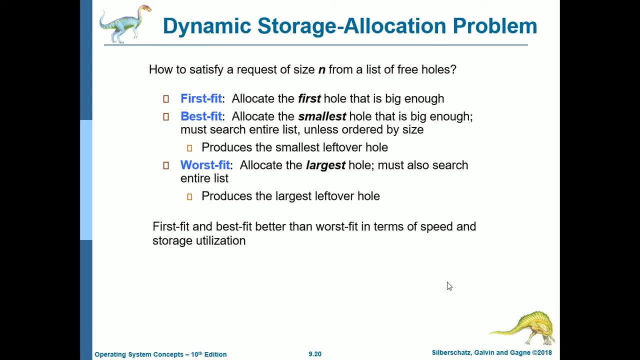 Must search entire list, unless ordered by size, And then produces the smallest left over hole And then we also have the worst fit. Allocate the largest hole Must also search the entire list. It produces the largest left over hole. So first fit and best fit. 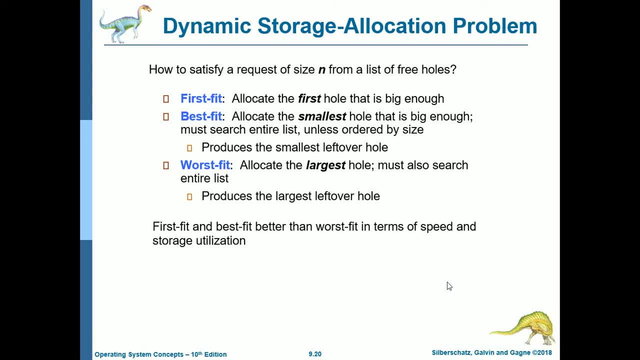 and best fit, better than worst fit in terms of speed and storage utilization. so, for example, let's have an example here. okay, for example, this is our memory. okay, example, let me allow me to draw okay example. this is already uh being uh occupied. and then, for example, we have 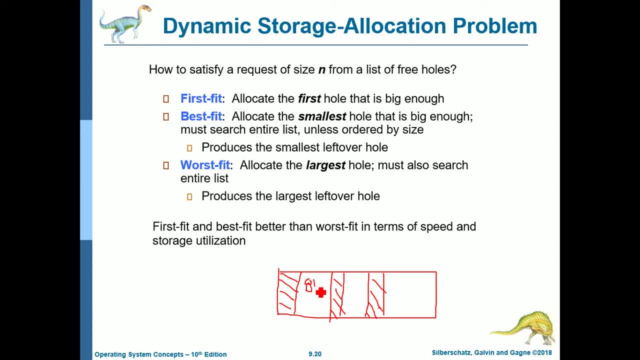 for example, right, just for example, 8 mb, just for, for our example, we have 8 mb, we have 6 mb- okay, sorry for the handwriting- and then we have 10 megabyte free space, for example, and then, for example, we have a chunk. for example, this is 5. 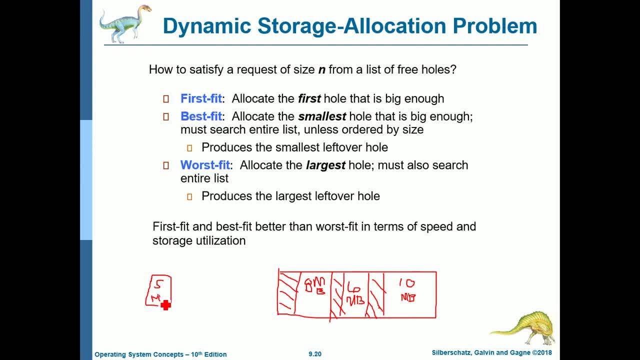 mb. okay, so let's have an example. assuming our block here is is equally. uh, it's a square, okay, so, uh, i'm sorry for my good drawing. uh, my first is we have, uh, let's use the best fit of first fit, best fit and worst fit, for example, 5 mb. if we're going to use first fit, 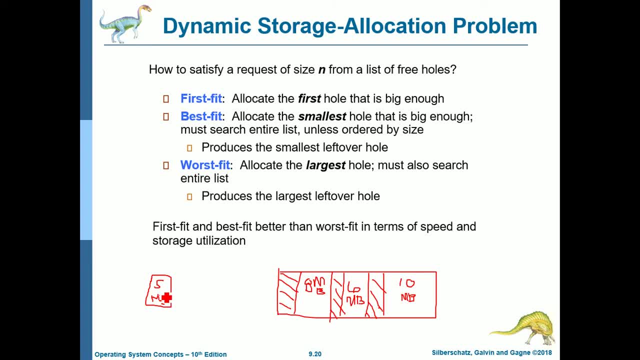 we where it will be. uh, where will our 5 mbb process be located or be situated? if you're talking about first fit again, allocate the first hole, this is that is big enough. since 5mb, it will first encounter 8 mb. so since this is the first hole, that is big enough for 5 mb. 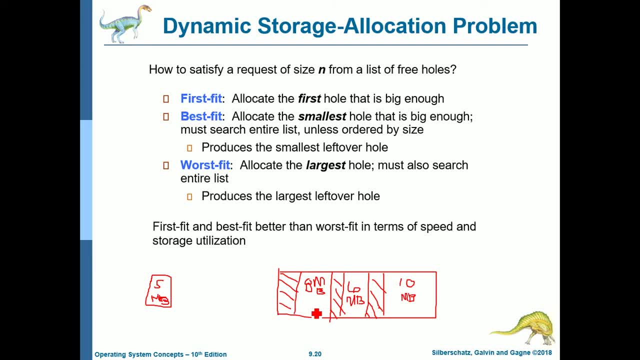 so 5 mb will be put inside this space for uh, which is 8 megabytes for first fit, okay, next, if best fit, so allocate the smallest hole that is big enough. must search entire list unless ordered by size, since this is not ordered by size, so it will check all the holes. 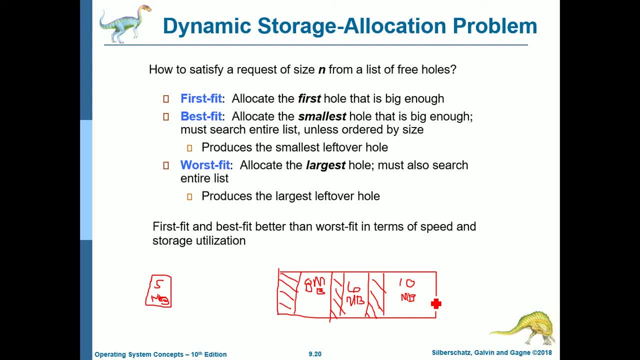 that is available. so we have 8, 6 and 10.. which of them has the smallest leftover hole? if 5 mb will be put inside that free partition, so actually the best using, best fit, it will be 6 mb, because if you're going to put it in 8 mb, you still have 3 megabyte. 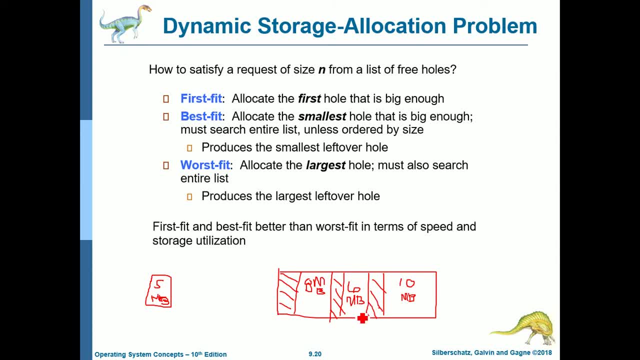 um left over hole for six, it's only one, and then for 10 we have five. okay, so for best fit, so five mb will be situated inside the six megabyte free partition. so last but not the least is we have the worst fit, so allocate the largest hole. 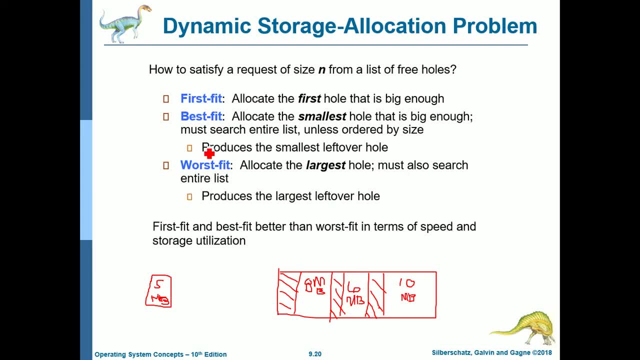 must also search the entire list. so, just like best fit, it will check all the available free partitions. then after that, of course, it will allocate the largest hole. so, um again, the left over here is g, this is one and this is five. so since for worst fit, it will always allocate the 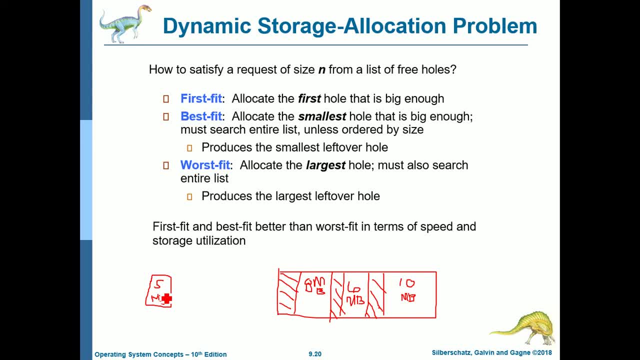 largest hole. so this 5mb for worst fit will be put inside the 10 megabyte free partition. so that is the difference between first fit, best fit and worst fit. so is there a case that uh, for for this fit, that uh, it will choose the, it will choose the um the same, um the same free partition. 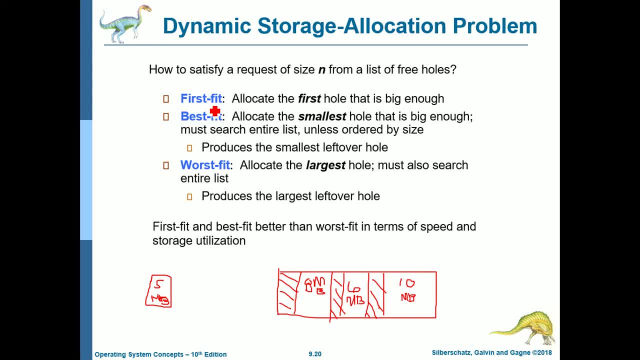 uh for uh for first fit and best fit. that's always possible. so what if, for example, 6mb will be uh put here and they, for example, they interchange the space? what if the, the location has changed? so first fit and best fit will have the same um free partitions that they will choose from, because worst fit will always. 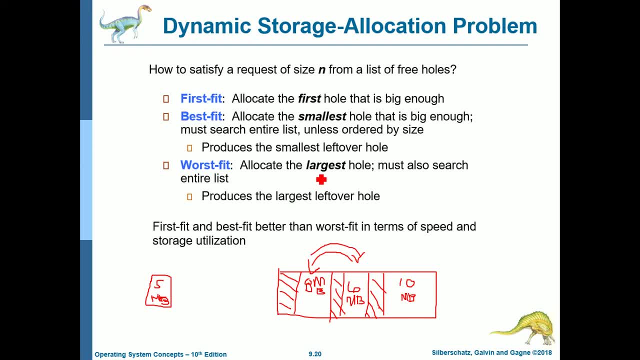 choose the- uh, the largest hole that it will fit. it has the largest left over hole if you're going to put the process inside. so this is an explanation of how to um, how to deal with the first fit, best fit and best fit. so this is an explanation of how to um, how to deal with the first fit, best fit, and. 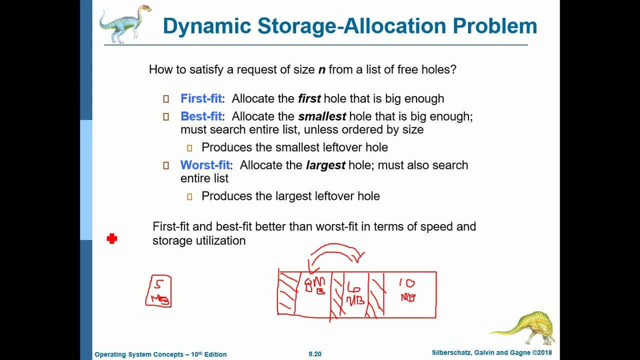 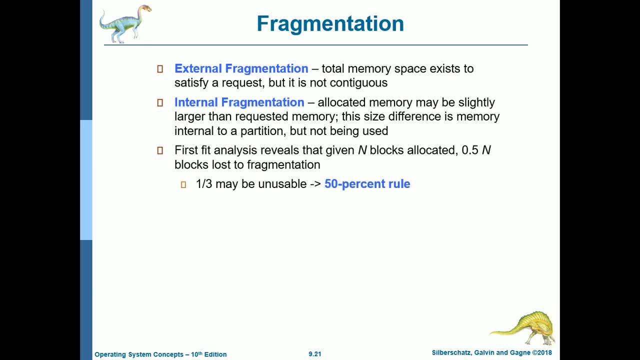 worst fit for the dynamic storage allocation problem. okay, next is we have fragmentation. so external fragmentation: total memory space exists to satisfy a request, but it is not contiguous. and then we have internal fragmentation. allocated memory may be slightly larger than requested memory. this size difference is memory internal to a partition but not being used. 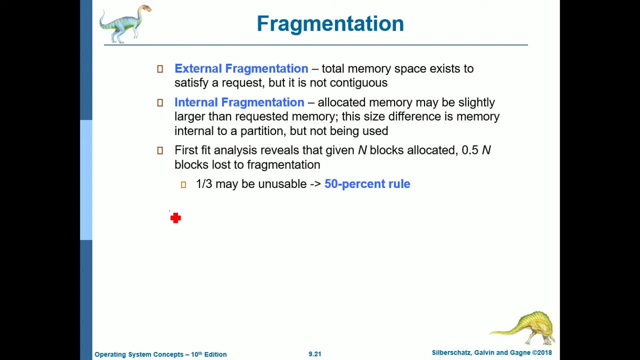 okay, so let's have another example. okay, so again, let me draw again a memory. okay, let's assume that this is already occupied. um, okay, for example, we have 4mb, for example. okay, and then i have another 4mb free space or hole. okay, what if your memory or the process that you have is: we have an 8mb? 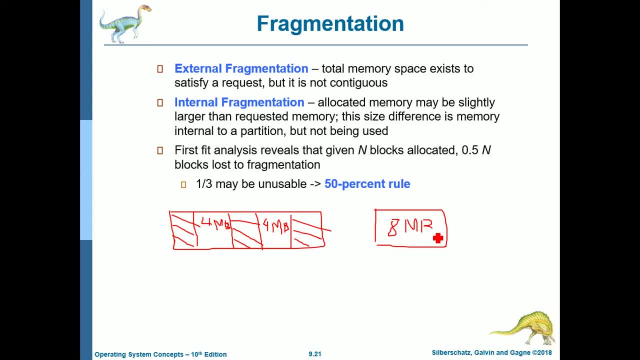 the size of your process is 8mb, it needs 8 megabyte um space. okay for external fragmentation. so this example is internal fragmentation. why? because if you're going to add 4 megabyte plus 4 megabyte is equal to 8 megabytes, but because, since they are, 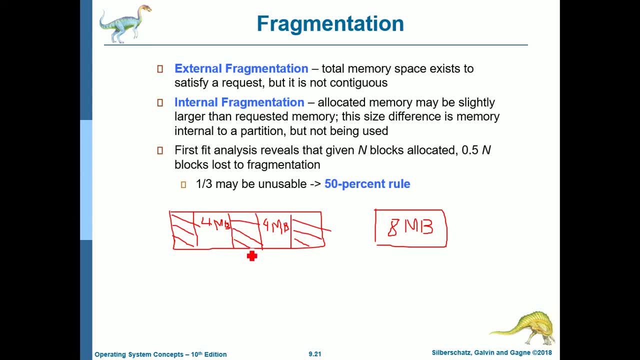 not adjacent to each other and there is, uh, this um portion which is occupied by another process. so this, this, so this is so called the internal fragmentation because, uh, again, the definition is: total memory exists to satisfy a request, exactly as 8mb, but it's not contiguous. 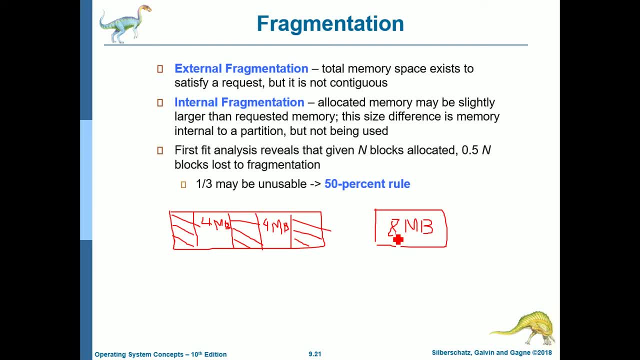 so still, this 8mb cannot be accommodated inside memory because the free space here are not contiguous. so what about internal fragmentation? so allocated memory may be slightly larger than requested memory. so this size difference is memory internal to appropriate memory. so this size difference is memory internal to. 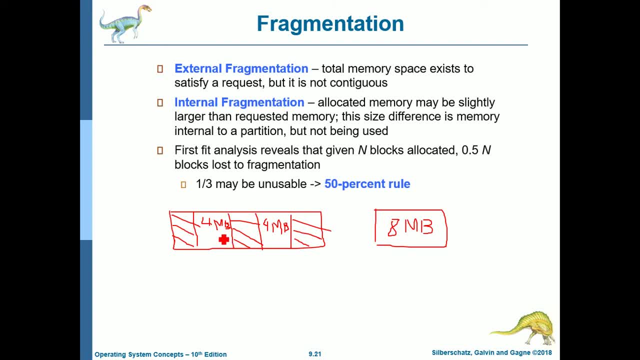 partition, but not being used. so, for example, we have 4mb and then we have we, we have a process that needs 3mb. okay, so actually 3mb will fit, 4mb. okay, this memory, uh, this will fit. so, but it will leave a hole, which is one. 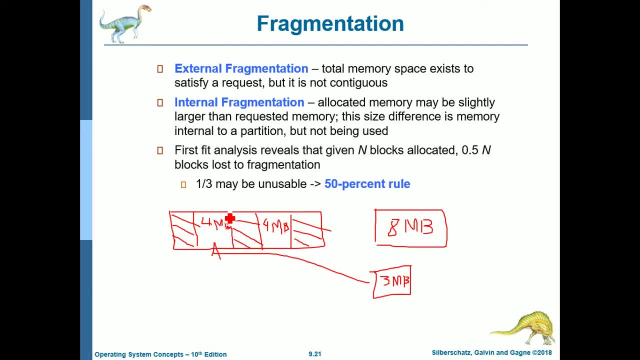 megabyte, so actually that one hole or one megabyte. there is called already the internal fragmentation, because the space here is four megabytes but because the- uh, the process that has arrived needs three megabytes. and then if you're going to put here, and then there is still. 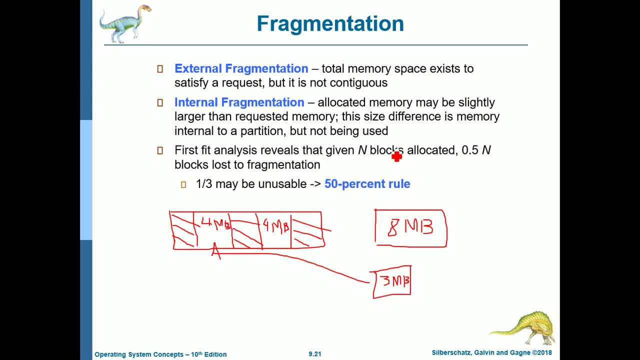 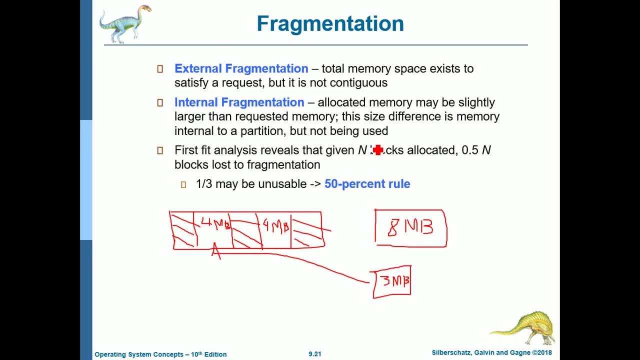 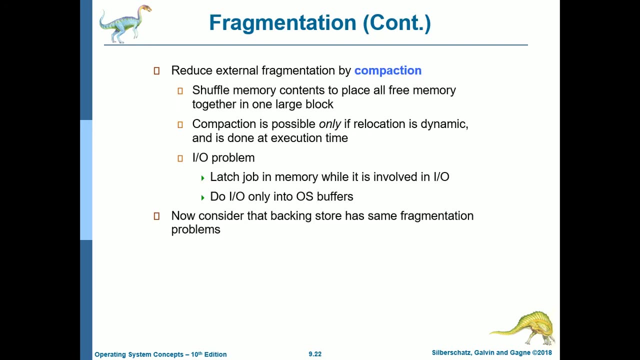 one third may be unusable, so we go i. so it means that they have to use the 50 rule, so that's why it's 50. we have 0.5 endblocks loss, loss to fragmentation. okay. what's the solution for that? so reduce external fragmentation by 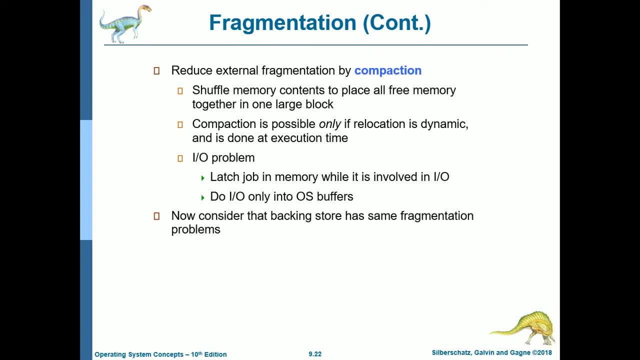 compaction. so shuffle memory contents to place all free memory together in one, in one large block. so compaction is possible only if relocation is dynamic and is done at execution time. so we have the io problem. so latch job in memory while it is involved in io. so that is the problem. 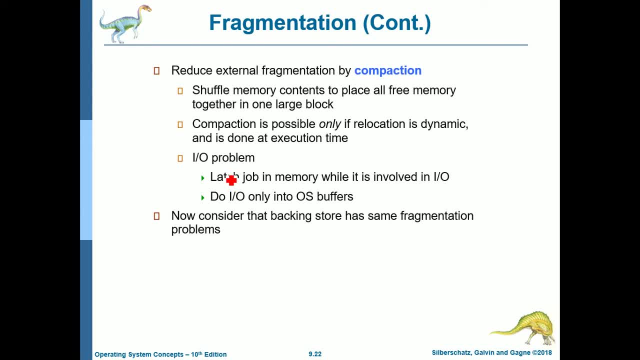 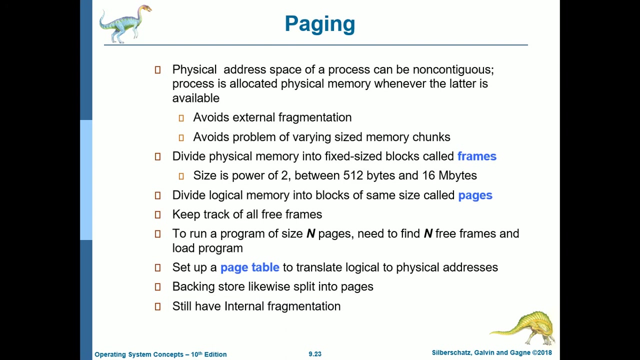 with compaction if the relocation is dynamic, because of course for io the address is fixed, so do io only into os buffer. so that's the solution. so now consider that backing store has some fragmentation, has the same rather fragmentation problems. so next is we have paging. so physical address space of a process can be non-contiguous. process is allocated. 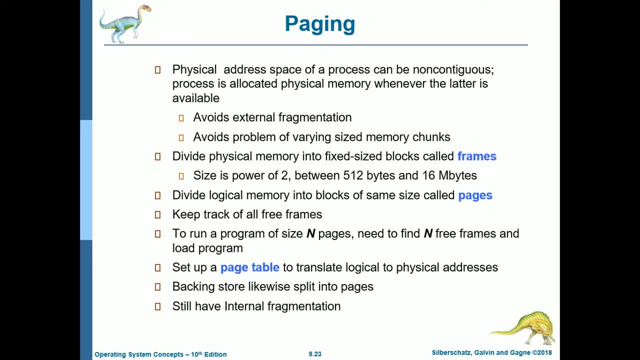 physical memory whenever the latter is available, so paging, uh. this avoids external fragmentation, avoids problem of varying size memory chunks. so divide physical memory into fixed size blocks called frames, so size is a power of two, between 512 bytes and 16 megabytes. so also divide logical memory into blocks of same size called pages, and then keep track of all. 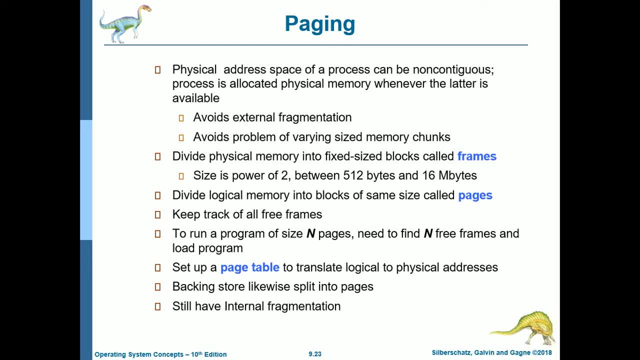 free frames. so to run a program of size n pages need to find n free frames and load program. then set up a page table to translate logical to physical addresses and backing store. likewise split into pages and though it avoids external fragmentation, they still have an internal fragmentation for 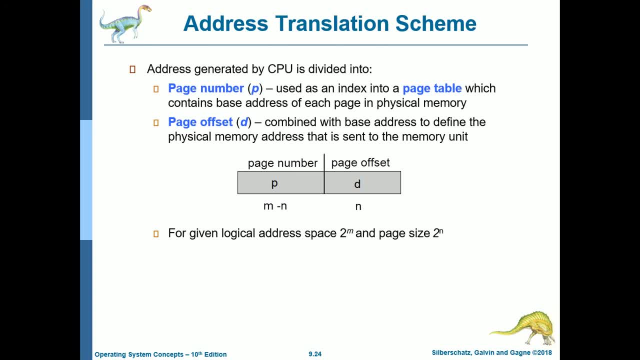 this setup. so we have the address translation scheme. so so address generated by cpu is divided into. for using the paging is: we have the page number, or p uses an index into a page table which contains base address of each page in physical memory. and then we also have this page offset, or d, combined the with base address to define the. 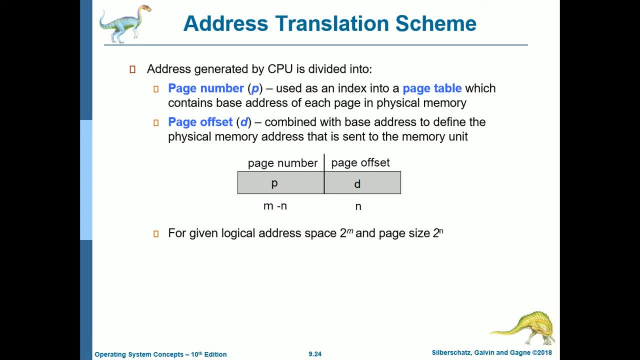 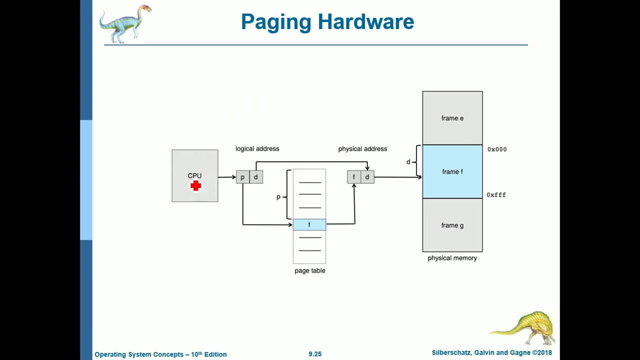 physical memory address that is sent to the memory unit. so we have this page number and then page offset. so for given logical address, space two raised to m and page size of two raised to n. so this addresses are powers of two. okay, so how does the paging hardware work? so, for example, so the cpu, so the cpu's logical. 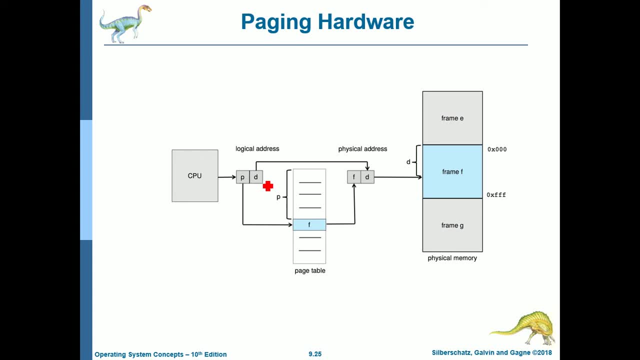 address will be composed of the page number and the page offset, so as already indicated here, and then the page number points to the page table the corresponding uh values of the for the logical address space, and then we have this offset will be added with the physical address once the value of page number is already is located in the page table. so for 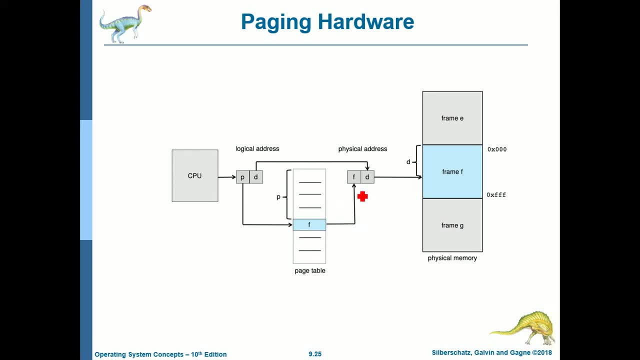 example, this is f, so our example here is f. then combined with the physical uh, rather with the offset of a page offset, and then this will be uh. the physical address will be the page number, so to will be used so that it will be situated inside the main memory or in the physical memory. 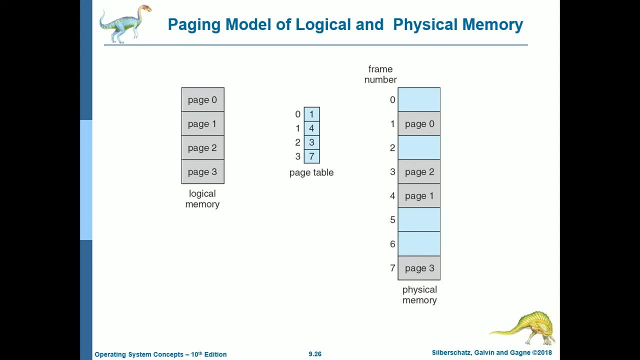 okay, next is paging model of logical and physical memory. so we have logical memory- page 0, page 1, page 2 and page 3, and then we have a corresponding page table. so page 0 will be situated in physical memory frame number 1, so that's why it's here. so so our page 0 is in frame number 1. 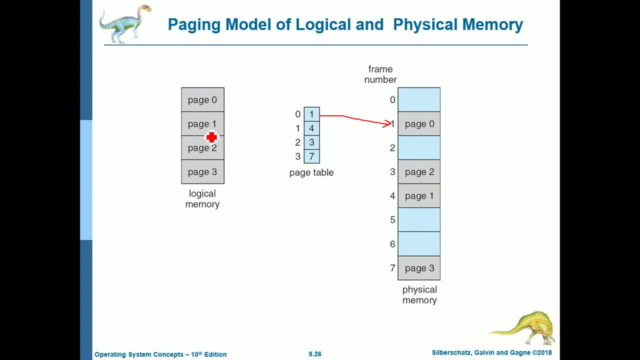 because in the page table it is indicated here. so our page 1 will be will be located in frame number 4 of the physical memory, and then page 2 will be located in frame number 4, 3 in the physical memory and, last but not the least, page number 3 will be situated in page. 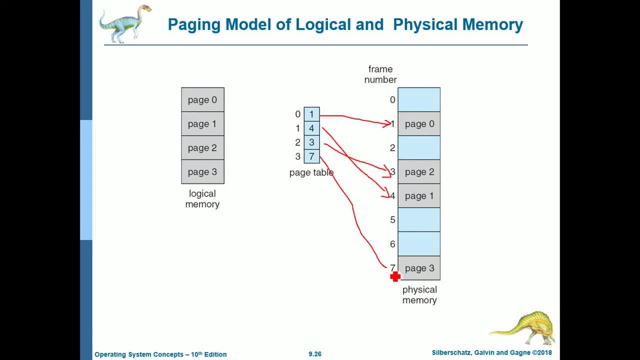 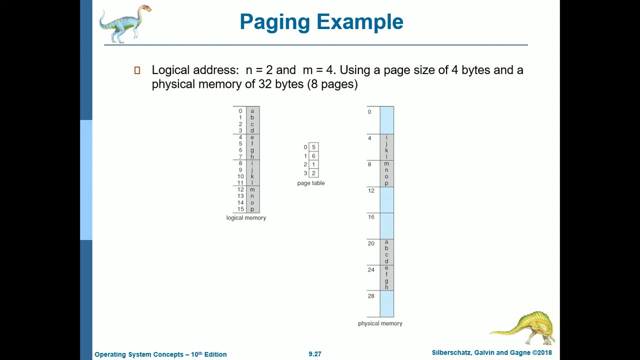 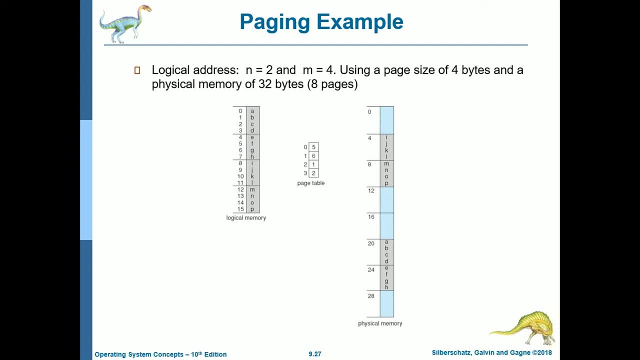 4 equal to 4, so use a page size of 4 bytes and a physical memory of 32 bytes or 8 pages. okay, so we have m is equal to. we have my at. the page size is 4 bytes. okay, so we have our page table. okay. since xs is equal to 5 and p is equal to 5 and p is equal to xs is equal to area, political income, example. so our paging table is its original page size, because this paging table is composed of pages. possessive cost this, the fact that, uh, there's no time limit and that one doesn't actually. uh, yeah, but 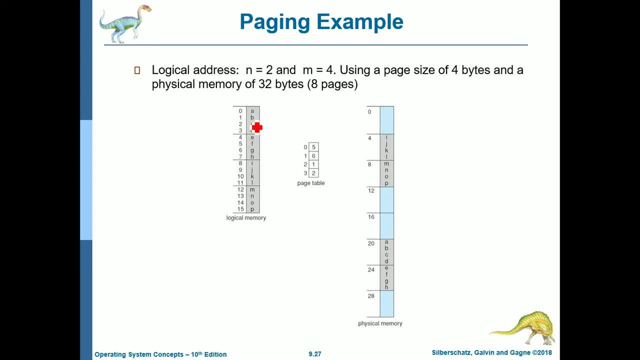 uh, there's a requirement. uh, something about that is that there's some requirement here, because in the So our logical memory here is A, B, C and D, So it will be located at 5, since we have to multiply it by 4.. 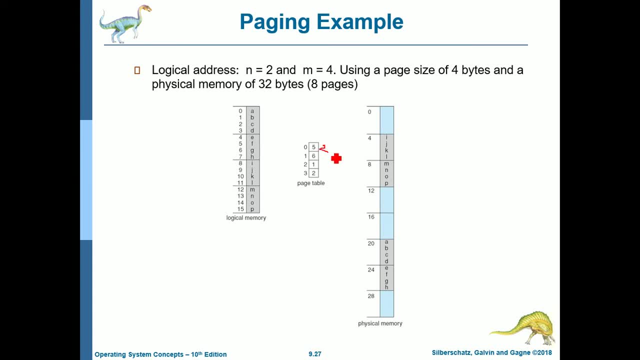 So 5 times 4 will be equal to 20.. So that's why our A, B, C and D is located in number 20.. Okay, next, This is our next data. Okay, so this will be located in 6 in the physical memory. 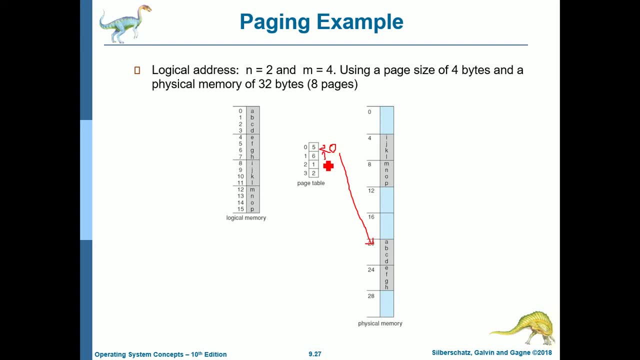 So times 4, we have 24.. So that's why this is located here. Then for I, J, K and L. So this will be located in: In 1 times 4 is we have 4.. 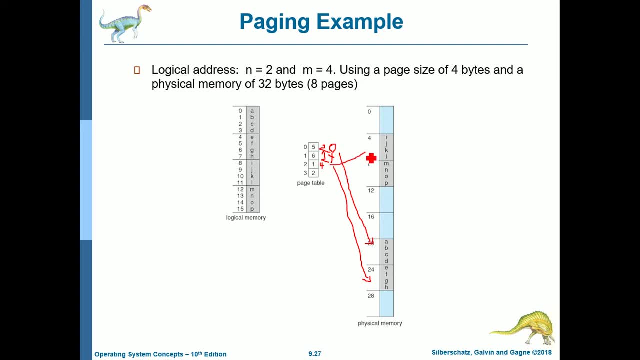 So that's why we have here in the frame number of 4, page size is 4 bytes. Okay, so in total the physical memory is equal to 32 bytes. And then, last but not the least, are M and OP will be in page 2.. 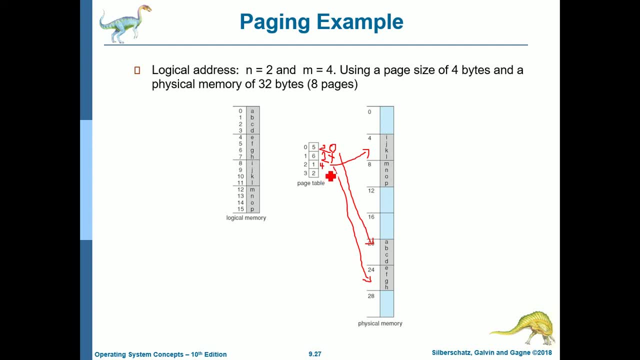 So for the page table, 2 times 4 is we have. So that's why M N O P is here in the frame 8,, 9,, 10,, 11.. Okay, so this is used with bytes. 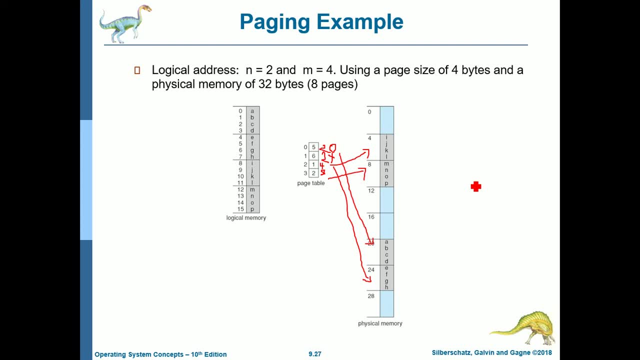 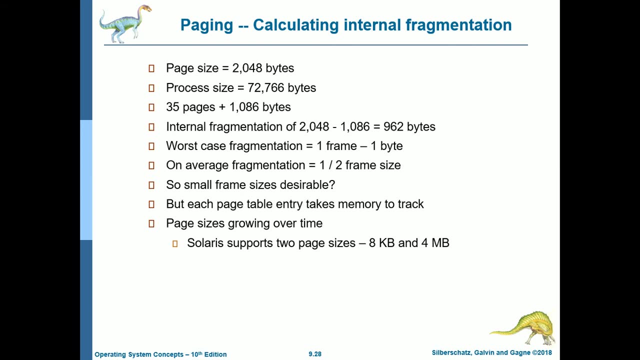 So that's why it is larger compared with the other example. Okay, next is we have paging, calculating internal fragmentation. So we have page size. Page size is 2,048 bytes And the process size is 72,766 bytes. 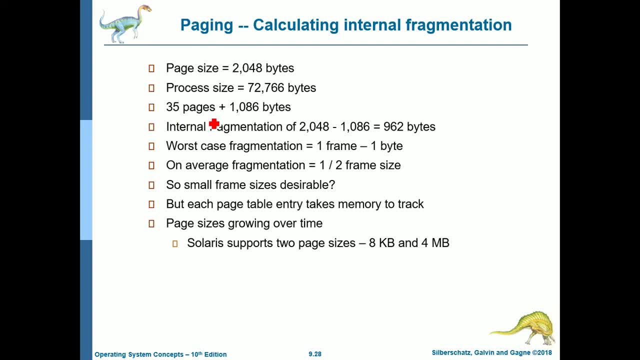 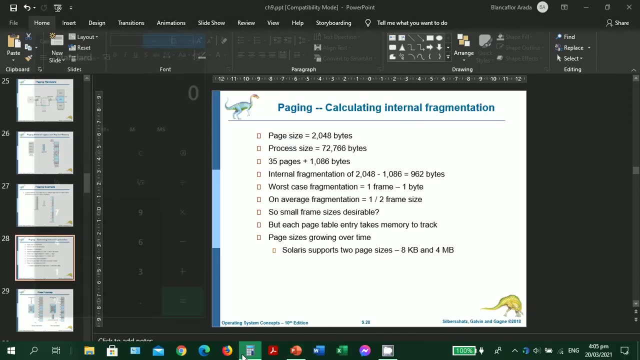 So we have 35 pages plus 1,086 pages. Okay so let's access our calculator. Okay so, let's just see the computation. So okay, our page size- This is 2,048 bytes- and process size: 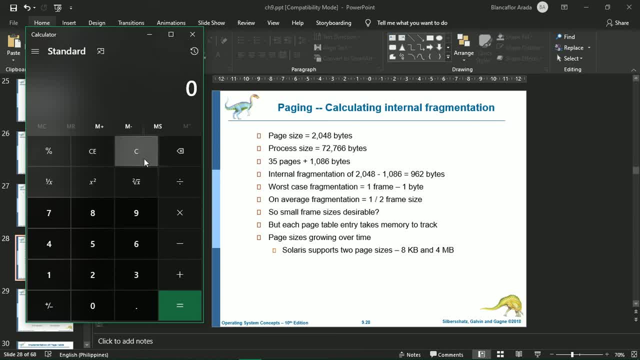 So how many pages will we need? So we have 72,766.. So we have divided by 2,048.. So that's why it's 35 pages And this decimal part with the decimal point. this is the remainder, the 1,086 bytes. 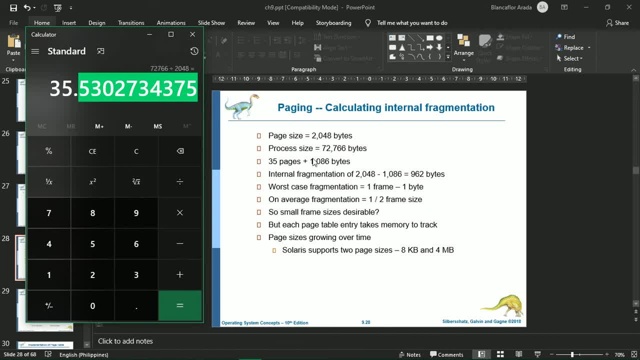 So 1,086.. So 1,086 in the powers of 2, where it will be, where will it fit? Okay, so we have it will fit. so powers of 2,, 2,, 4,, 8,, 16,, 32,, 64,, 1,, 2,, 8,, 2,, 5,, 6,, 5,, 12,, 5, 12,, 1,000,, 5,, 12,, 1,024, and then 2,048. 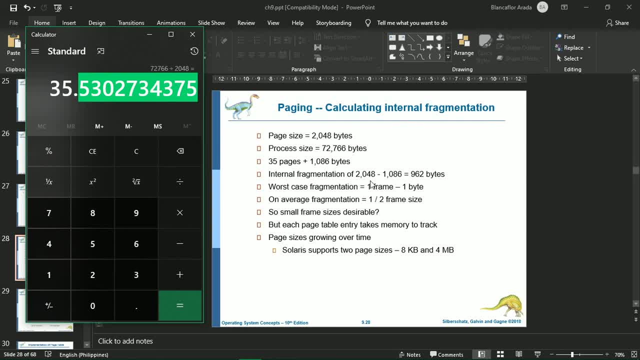 So 1,086 bytes will fit the 2,048.. So subtract, So internal fragmentation of 2,048 minus 1,086.. So we have 962 bytes. So worst case fragmentation is equal to 1 frame, which is almost 1 frame 1 byte. 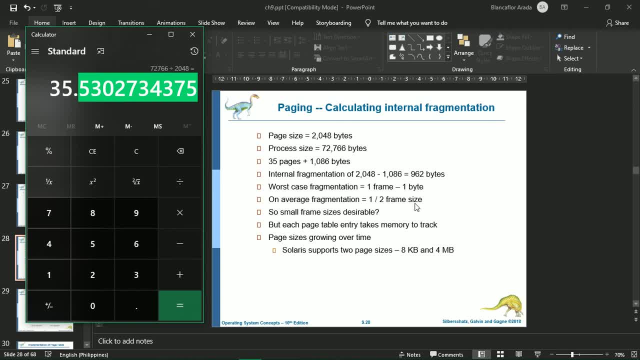 So on average, fragmentation is equal to 1 half frame size. So our small frames size is desirable, rather So. but each page, So each table entry takes memory to track. So page size is growing over time. 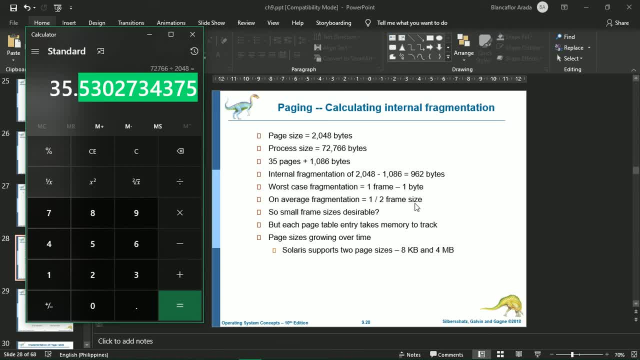 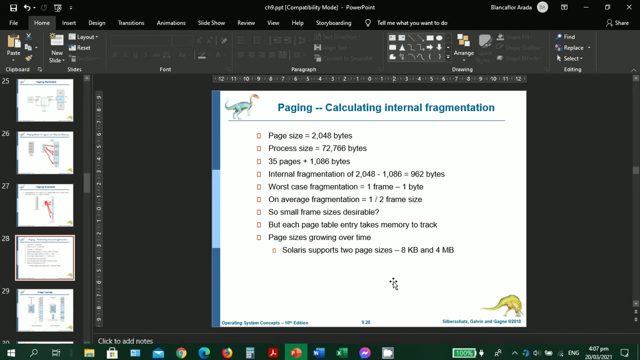 So, as much as possible, it is very convenient to have frame sizes that are big enough to accommodate other processes with big sizes for pages. So we have this. For example, we have Solari supports. So let's go back with our presentation. 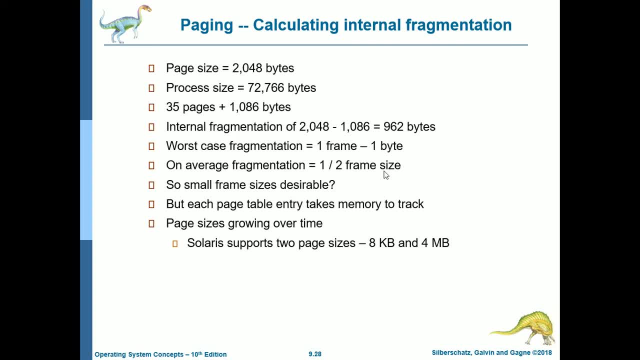 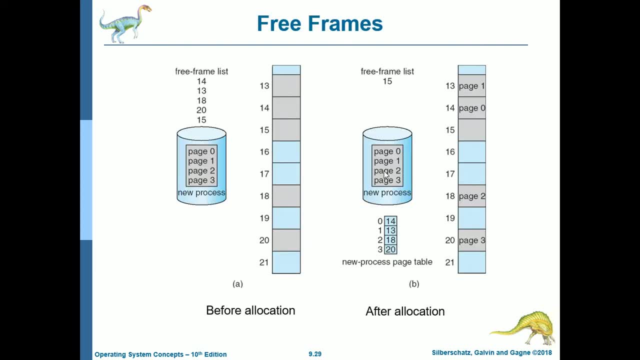 Solari supports 2. Page sizes, which is 8 kilobyte and 4 megabyte page sizes. Okay, Next is, we have free frames. So of course. So there are also free frames. So we have the free frame list. 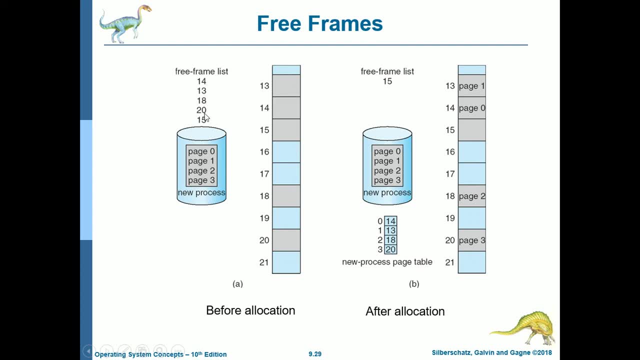 For example, we have the 14,, 13,, 18,, 20, and 15.. So this is our frame list, And then we have this in the backing store, the pages Page 0,, 1,, 2,, 3.. 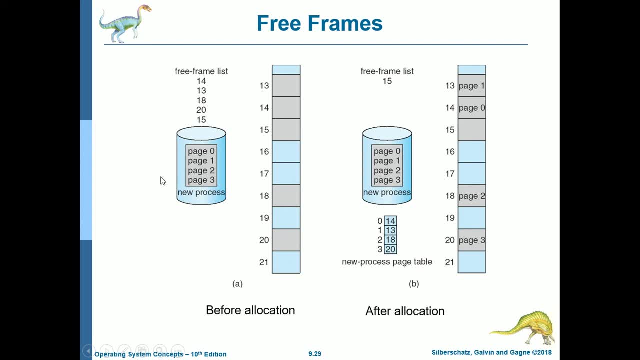 And then, of course, this is the backing store for new process. And then what happens here? since we have free frame list, then we need frames for these pages. So these pages will be assigned to, for example, page 0, will assign to frame number 14.. 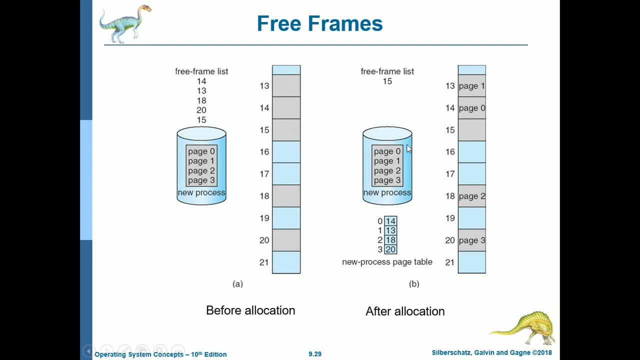 So that's why 0 is in frame number 14.. So page 0 is frame number 14.. And then page 1 is in frame number 13. So that's why page 1 is here, And then we have the page 2 will be located in frame number 18.. 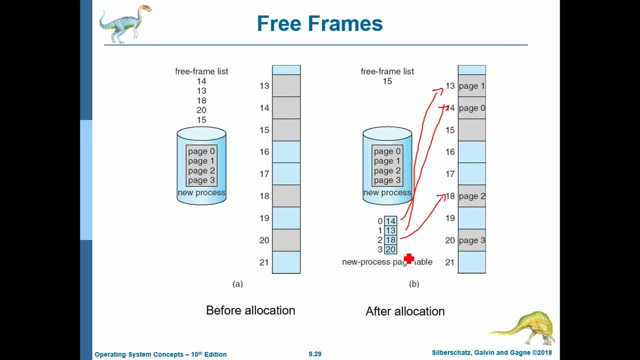 And then, last but not the least, we have the page 3 will be located in frame number 20.. So this is before allocation and after Allocation. So the allocation of pages will be: these pages will use the frames that are free. 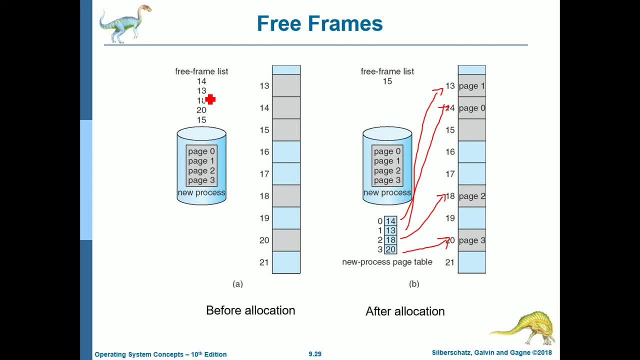 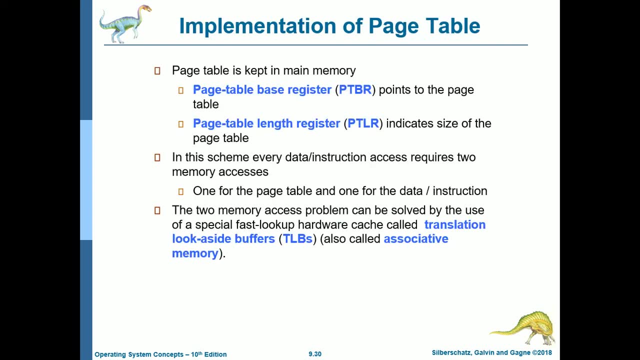 Or these are actually no process that's still been using these frames. Okay, next is we have implementation of page table. So page table is kept in main memory. So we have this so-called page table register, Or P-T-B-R points to the page table. 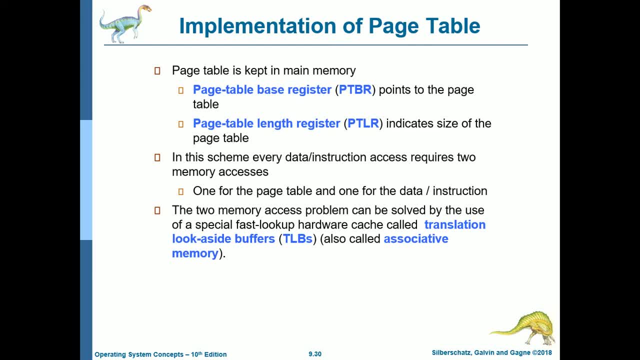 We also have the page table length register, or P-T-L-R indicates size of the page table, So base and length register. So in this scheme every data or instruction access requires two memory accesses, So one for the page table and one for the data or instruction. 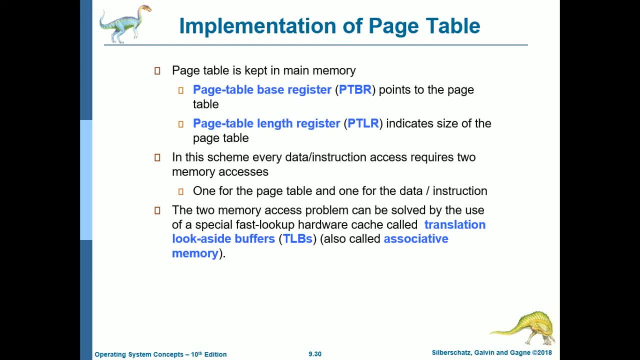 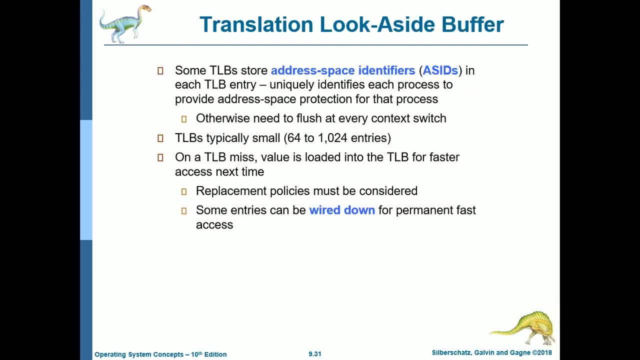 So that's why two memory accesses. So the two memory access problem can be solved by the use of special fast lookup hardware cache called the translation look-aside buffers, Or TLBs are also called associative memory. So what is TLB or translation look-aside buffer? 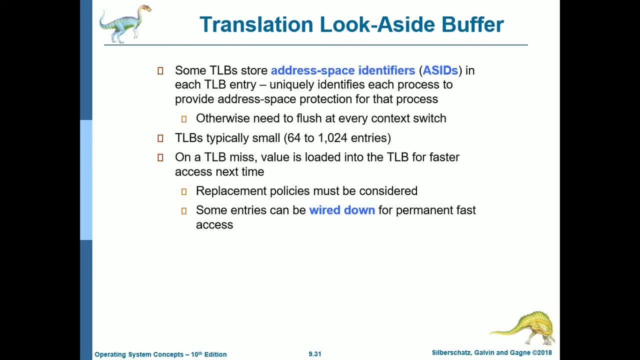 So some TLBs store address space identifiers in each TLB entry. So this uniquely identifies each process to provide address space protection for that process. So that's why it's called address space identifiers. Otherwise need to flush at every context switch. 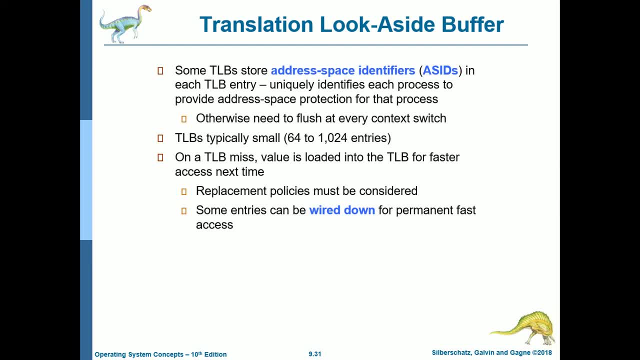 So flush means erase, So typically TLBs sizes are small, from 64 to 1024 entries. So on a TLB miss, so we have the TLB hit, If there's a TLB hit, meaning that the address is there on the TLB. 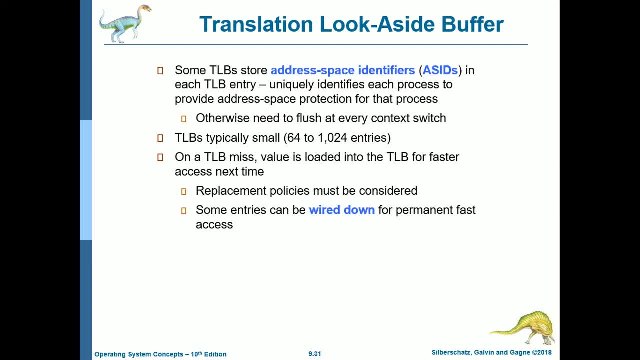 But if not, so it's a TLB miss. So value is loaded into the TLB For faster access time. So replacement policies must be considered And then some entries can be wired down for permanent fast access. Wired down meaning the values will not change inside the TLB. 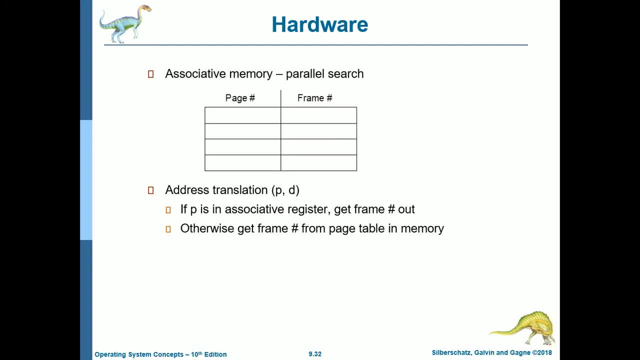 So hardware. So associative memory uses parallel search. So we have page number and frame number, So address translation is also the page number and office number. So if P is in associative register get frame number out. Otherwise get frame number from page table in memory. 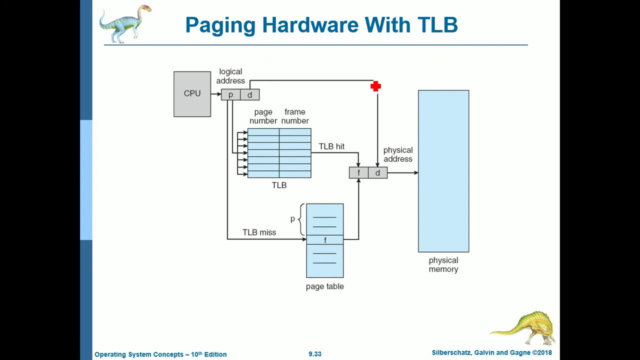 So this is what happens for paging hardware with TLB. So instead of only a page table we have TLB or translation look-aside buffer. So again, our CPU produces logical address P, And So we have a page number and a page offset. 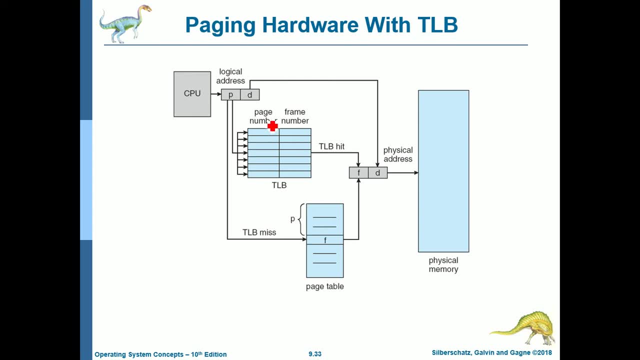 And then this page number has a corresponding value for the TLB, which is composed of page number and frame number. So if the value is inside this TLB, then we have a TLB hit. So this will be loaded faster in the physical address. 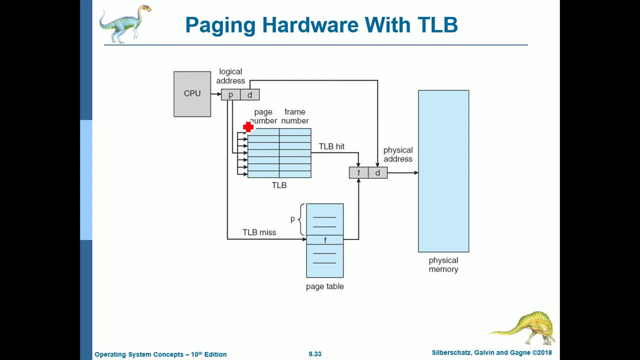 So what if the value is not here? So it's not in the TLB, So it's a TLB miss. So this is a TLB hit, So this is a TLB miss. The page number will be acquired from the page table and this will be loaded here. 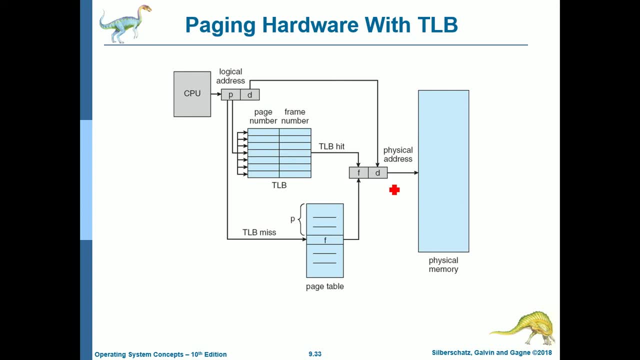 And then after the physical address. so you have to add for the physical address the offset and combining of course again the value. It's either from the TLB or from the page table. From the TLB if the value is already in the TLB. 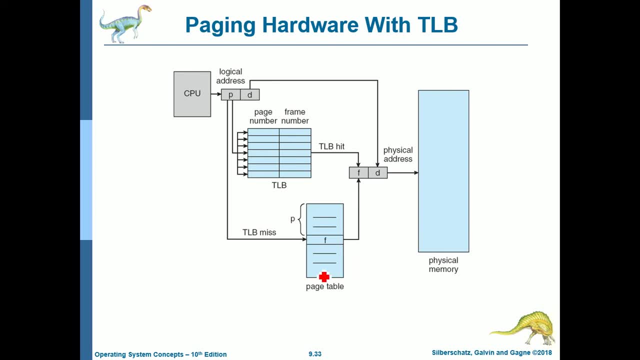 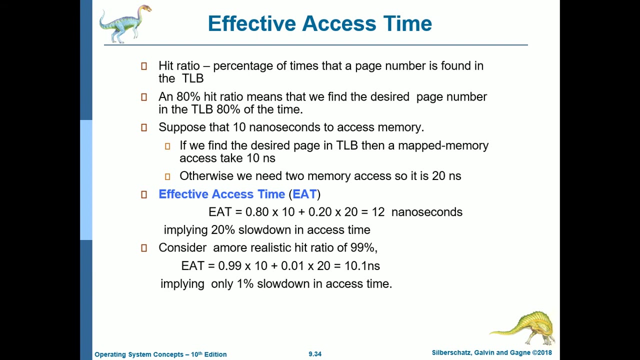 if it is located in the page table, meaning the value is not yet in the TLB. So this will be combined so that this will be the address in the physical memory. So we also have this so-called effective access time or EAT. 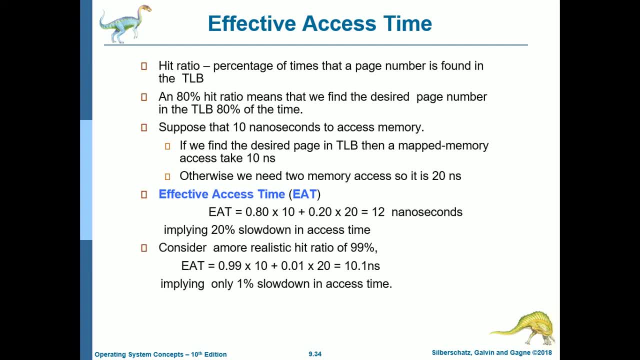 So we have hit ratio percentage of times that the page number is found in the TLB. So this is actually desirable. that the page number is already found in the TLB, So it will. The execution will be faster. but if the page number is not found in the TLB, 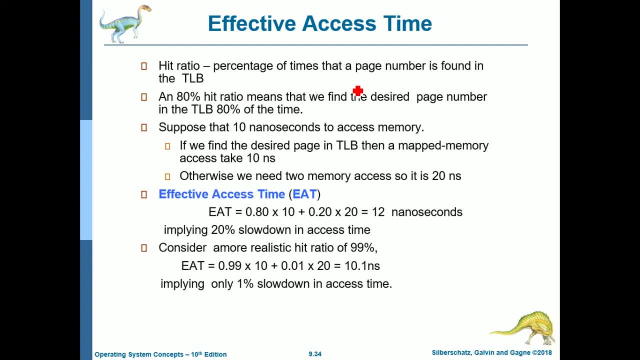 then it will be acquired from the page table. So an 80% hit ratio means that we find the desired page number in the TLB 80% of the time. So we have this example. So suppose that 10 nanoseconds to access memory. 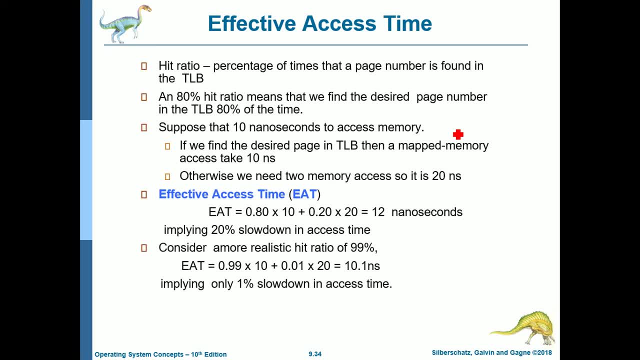 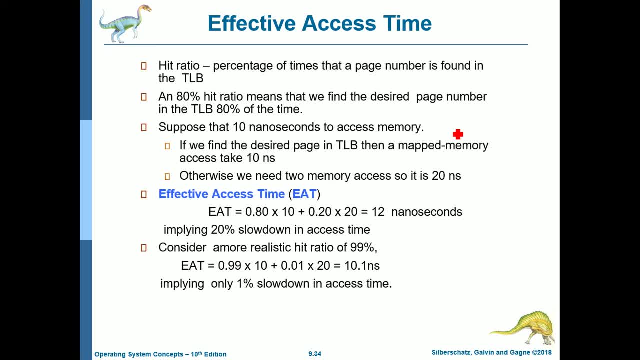 So if we find the desired page in TLB, then a map memory access takes 10 nanoseconds, So otherwise, so what if it's a TLB miss? We need two memory access, so it is 20 nanoseconds. 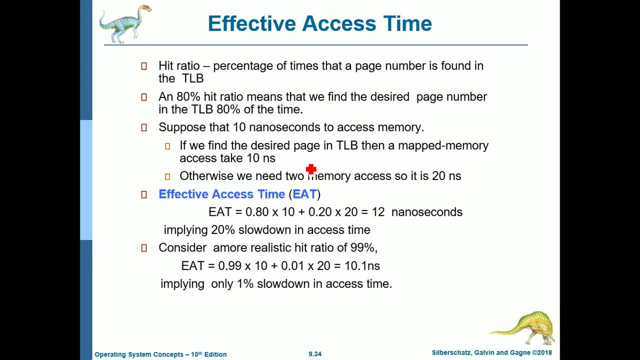 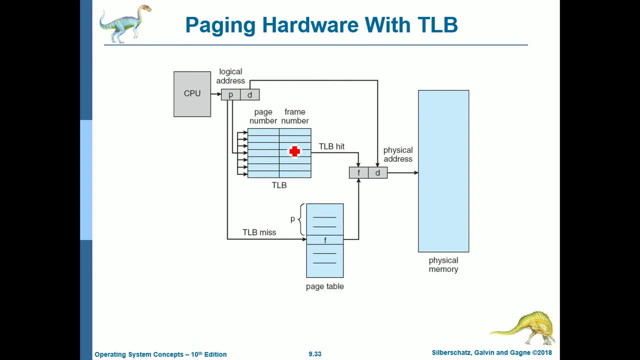 So why is it two memory access? As we can remember, let's go back with the figure. So for the page number it will always search first for inside the TLB. If the page number is already available, so that will be a TLB hit. so it's only one access. 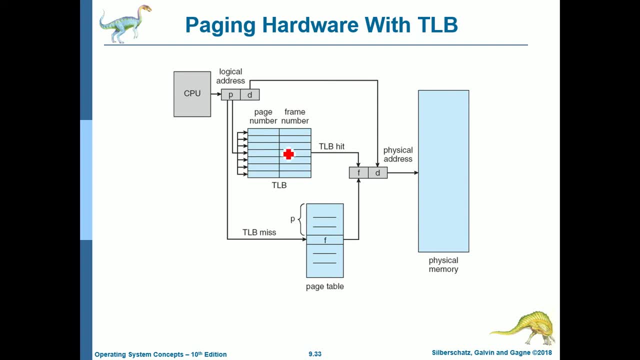 But once the page number is not available in TLB, so first it is accessed in TLB and then it will also access the page table. So that's why the memory access is times two, because you need to look first at the TLB. 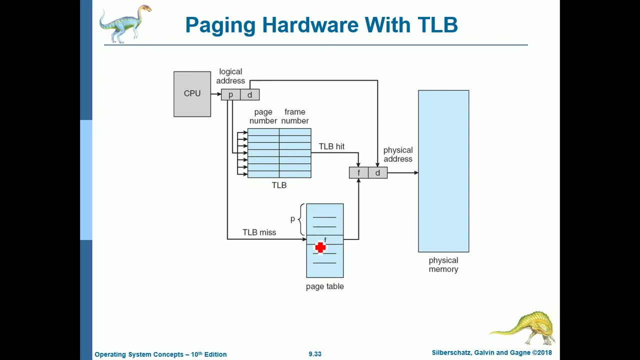 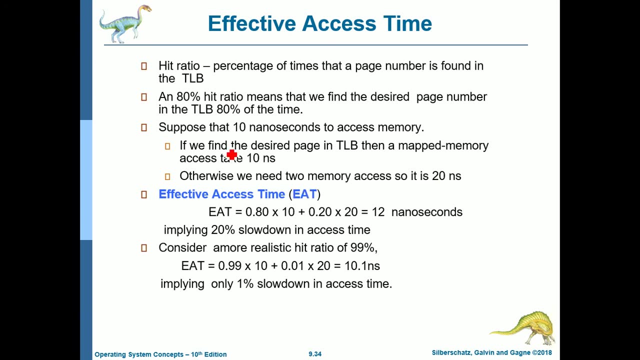 and if it's a miss then you need to look at the page table. So for TLB miss it will be 20 nanoseconds, 10 times two. So what is the effective access time? So the effective 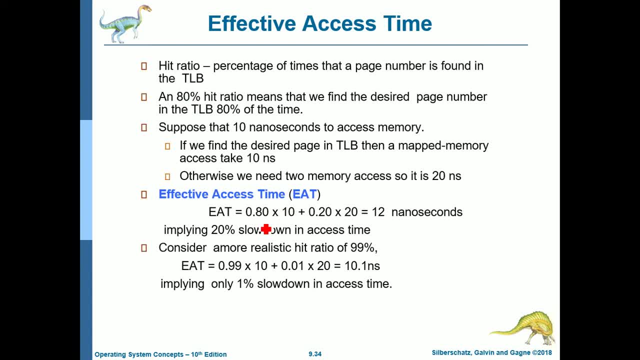 So the effective access time is what? So 80%, so we have 0.80, then the access is 10 nanoseconds. So this will be for the TLB hit and then this part is the TLB miss. 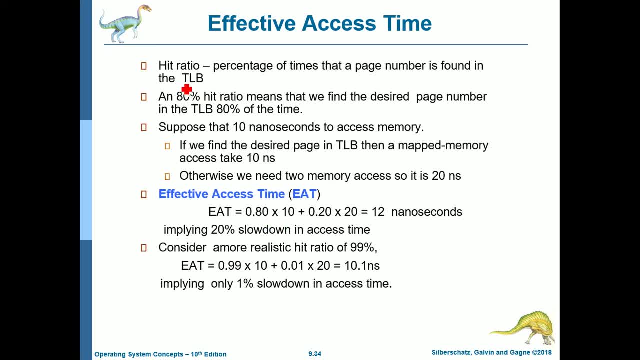 So we have 100 minus 80,, which is 20%, or 0.20 times 20,, since if it's a TLB miss, it accesses the memory. So that's why 2 times 10, so we have 20, is equal to 12 nanoseconds. 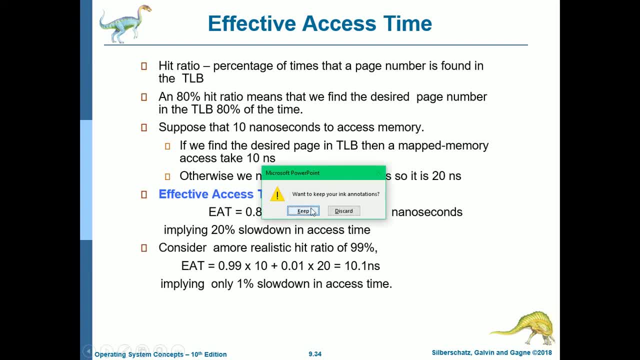 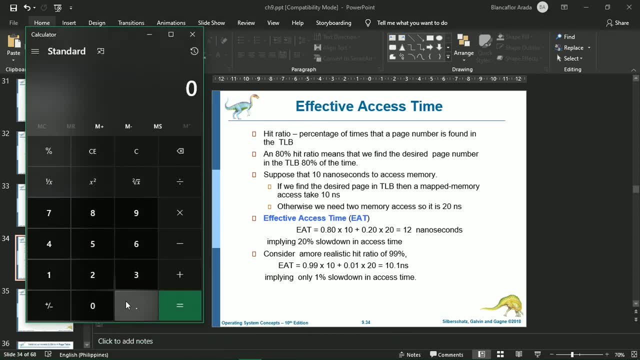 So we can also again have our calculator. okay, So again our calculator here. So just to make sure: 0.80 times 10,, okay, So we have 8, and then 0.2 times 20,, 4 plus 8,, so of course we have 12,. 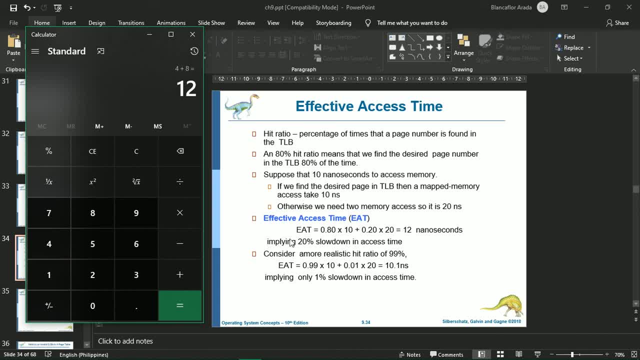 implying 20% slowdown in access time. So what is this 20%? Okay, since our access time to access the memory is 10 nanoseconds, then we have 12 nanoseconds, meaning it adds 2 seconds to access memory. 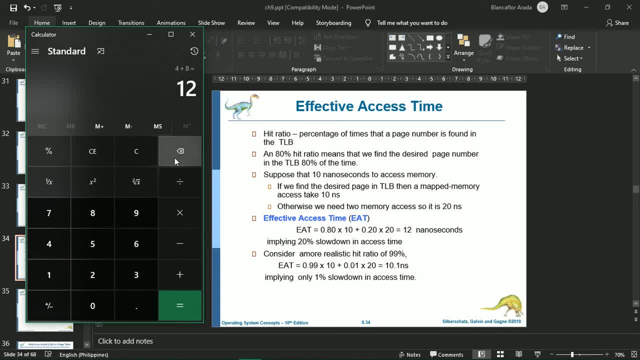 Because of the TLB miss. So what we're going to do here is: 12 minus 10 is equal to 2, and then this 2 will be divided by 10, because that is the time it takes to access the memory, the ideal. 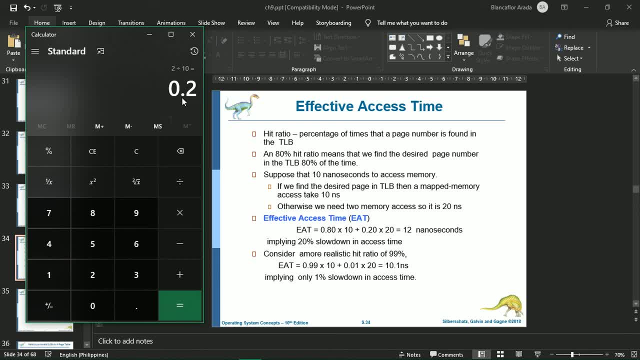 Okay, so 2 divided by 10 is equal to 0.2, or, if you're going to do it in a percentage, so it means 20.. That is Why There is a 20% slowdown in access time. 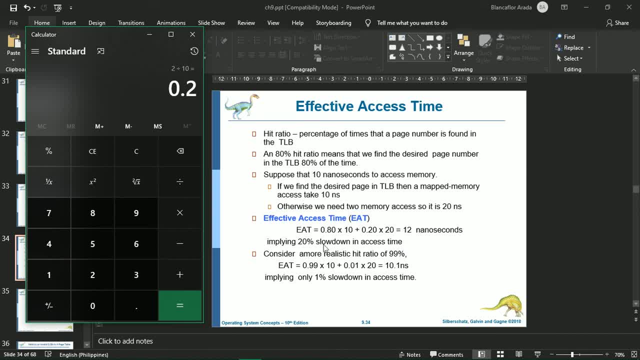 So that 2 seconds here is the 20% slowdown in access time. Okay, so what if we have consider a more realistic hit ratio of 99%? So we have 99, so it means that. so our TLB hit ratio here is 0.99, since 99%. 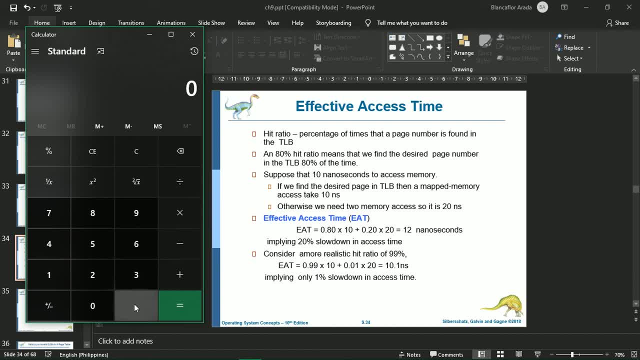 So our effective access time, of course again. So we have 0.99 plus, or rather- okay, let's repeat it again- 0.99 times 10, so we have 9.9, and of course this is the TLB hit. the TLB miss is of course 100 minus 99,, which 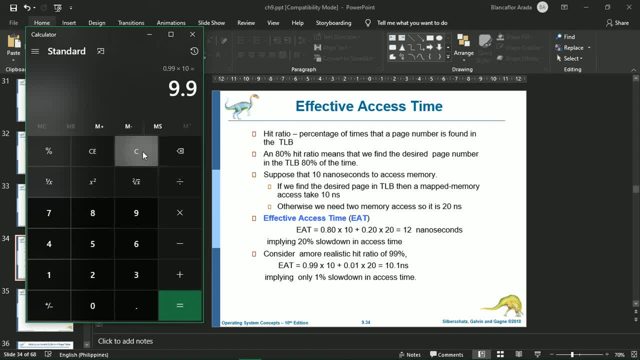 is 1,, which is 1%. so that's why 0.1, 0.01 times again. because 20, because of you know this is a TLB miss. it needs to access memory twice, so times 20 is equals to 0.2. 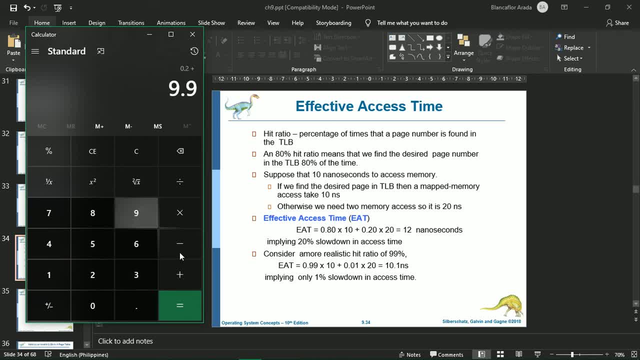 plus 9.9 for the previous for the TLB hit. okay, we have 10.1 nanoseconds, so implying only 1% slowdown in access time. so how do we get again this percentage with the same with? here? with the 20% is we have 10.1,, of course, again, our access time is 10 nanoseconds. 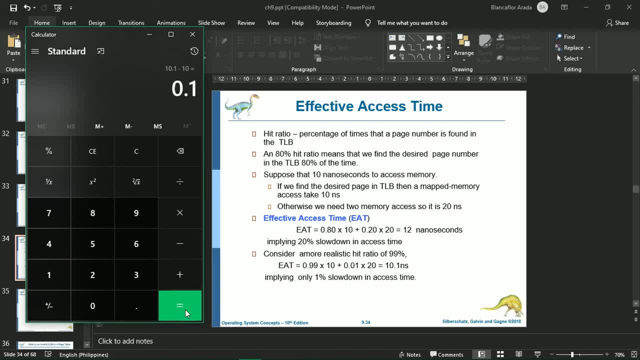 as indicated in the problem, minus 10,, so we have 0.1, then again divided by 10 nanoseconds, so we have 0.01,. so if we're going to convert it into percentage, so this will be the 1%. 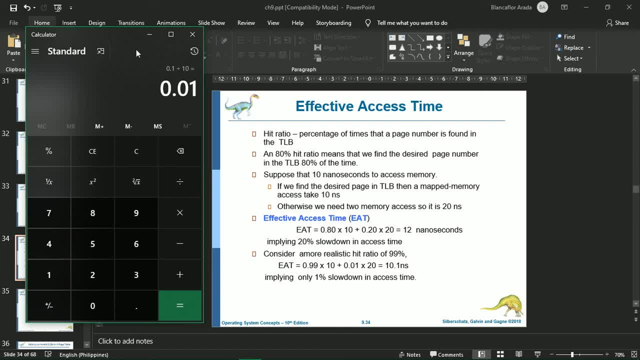 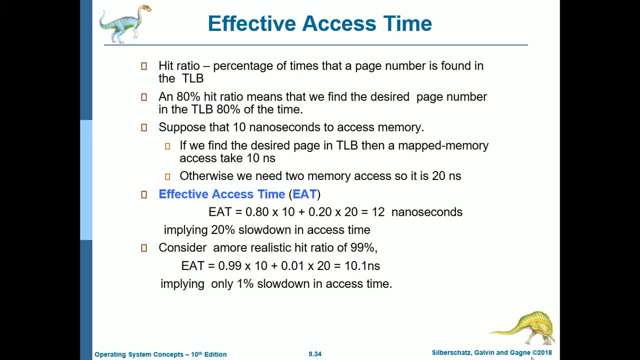 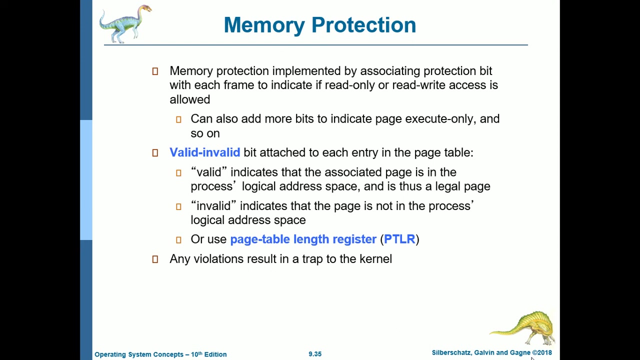 slowdown in access time. So I hope you understand How to compute the effective access time by in use by when using translation look-aside buffer. Okay, so let's continue. Next is we have memory protection. So memory protection implemented by associating protection bit with each frame to indicate. 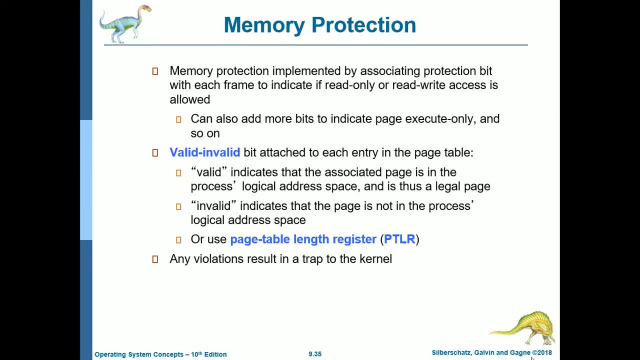 if read-only or read-write access is allowed, Can also add more bits to indicate page execute-only and so on. So we have the valid-invalid bit attached to each entry in the page table. So valid indicates that the associated page is in the process. logical address space and. 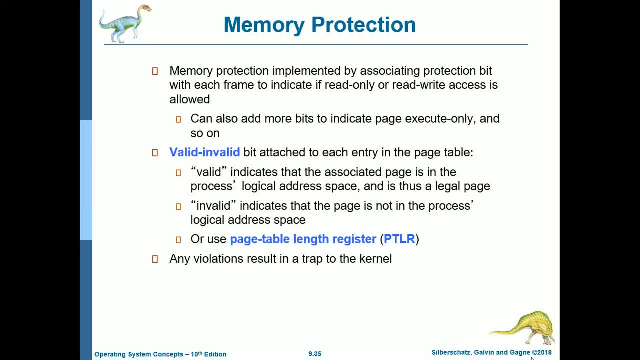 is thus a legal page. And then we also have invalid indicates that the page is not in the process, logical address space, or we could also use the page table length register or the PTLR. So any violations result in a trap to the kernel. 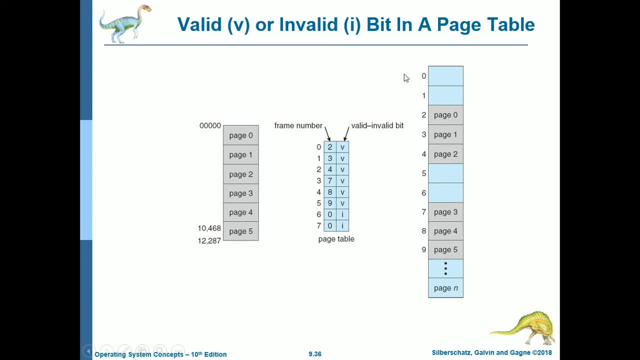 So we can see, for example, how does the valid or invalid bit in a page table is applied. So for we have 1,, 2,, 3,, 4,, 5, 6. So we have six pages for logical memory or address. 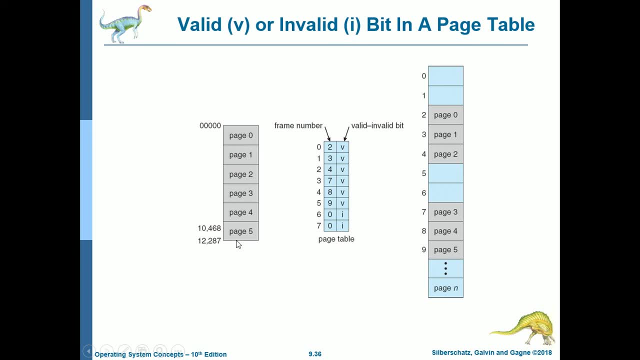 So this six pages is loaded here, So zero will be located. Then page two. So page one will be located in page three. So page Okay, Let's return again, Okay, Okay, So again, page zero will be located in page two. 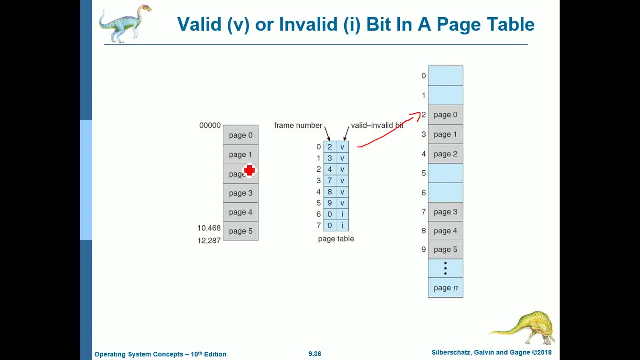 Or rather frame number two of the physical memory. Then page one will be in frame number three, So that's why it's in frame number three- And then page two will be in frame number four, And then, And then we have page three will be in frame number seven. 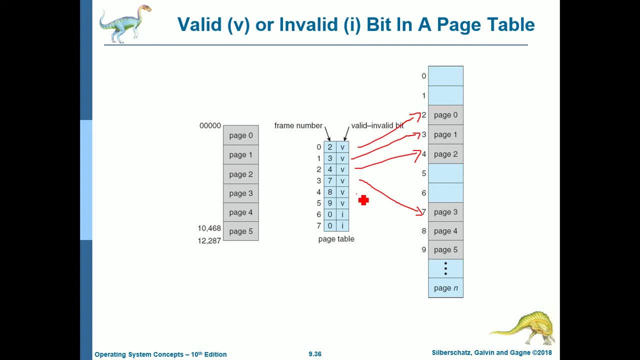 And then page four will be in frame number eight And we have page five will be in frame number nine. Okay, So this six pages. So by using valid or invalid bit, they're all V. They're all valid because they're all existing as logical address. 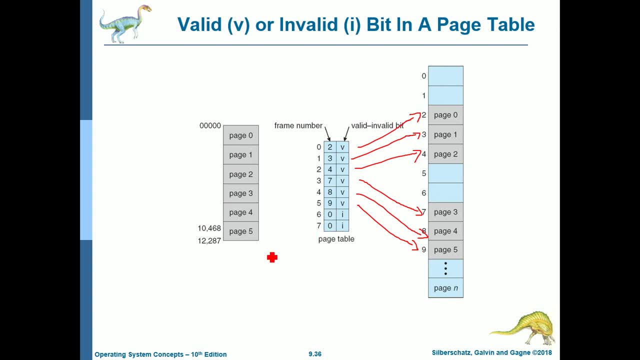 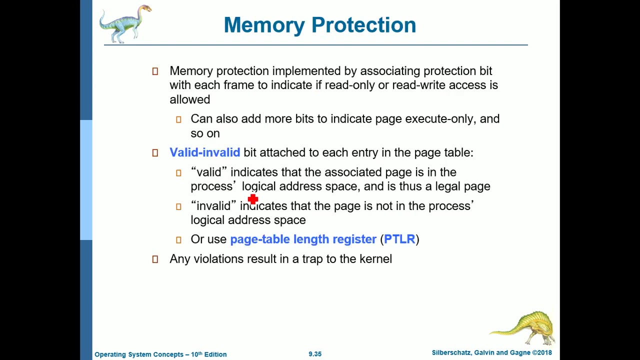 So we have six and seven. Since It does not exist here, the logical address, So the valid invalid bit here is: we have I So, as you can remember, here valid if the associated page is in the process: logical address space. 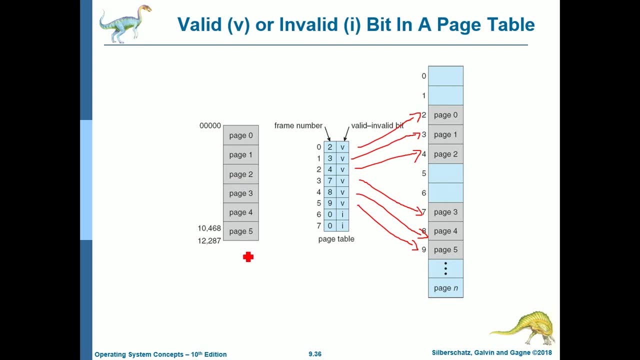 So invalid, since we do not have for page six or page seven, we only have six pages, And here is we have eight, Since We don't have for the seventh and eighth page for it. So that's why these are all invalid. 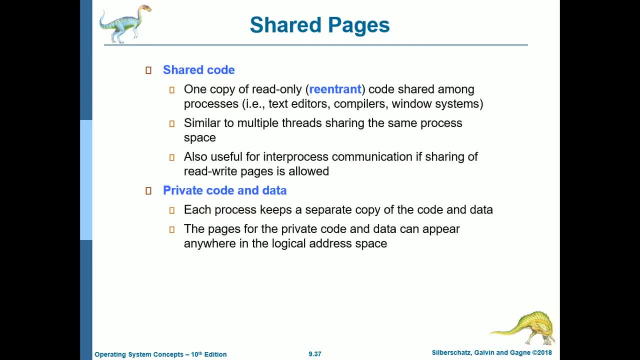 These two Okay. Next is: we have shared pages, So we have shared code: One copy of read-only or re-entrant code shared among processes such as text editors, compilers and Windows system. What is re-entrant? So re-entrant is a non-modifying code. 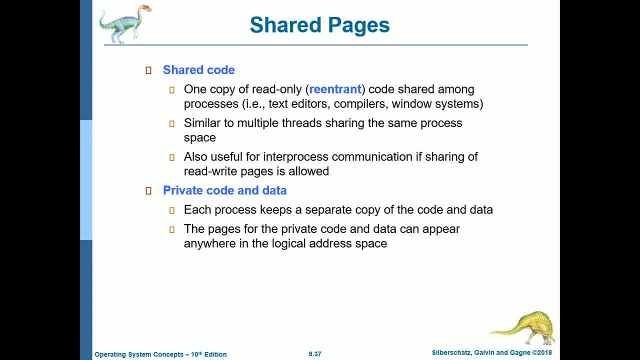 It never changes during execution. So similar to multiple threads sharing the same process space. So this is useful. the shared code for inter-process communication. if sharing of read-write pages is allowed, Then we also have the private code and data. 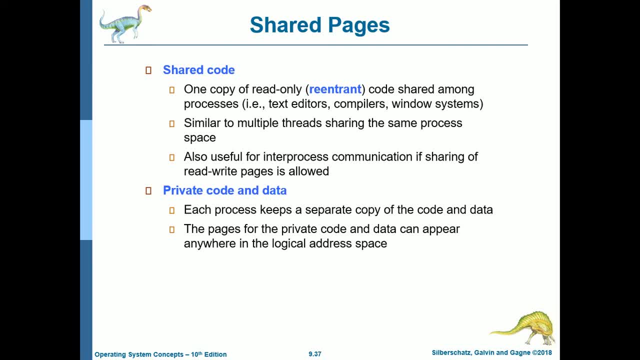 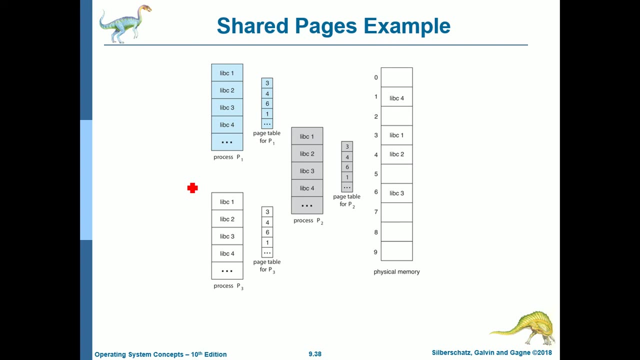 So each process keeps a separate copy of the code and data. The pages for the private code and data can appear anywhere in the logical address space. So we have shared, So we have shared pages, example here. So we have this for process P sub 1 and process P sub 3.. 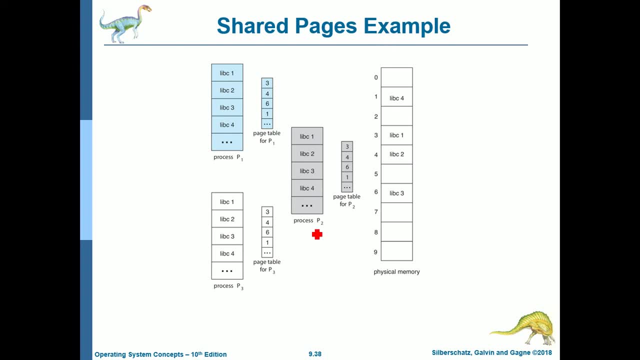 So we also have process P sub 2 and then they have their corresponding page table for P sub 1,, P sub 3, and P sub 2.. But since they are using the same libraries and page table, So it should be located all at the same. 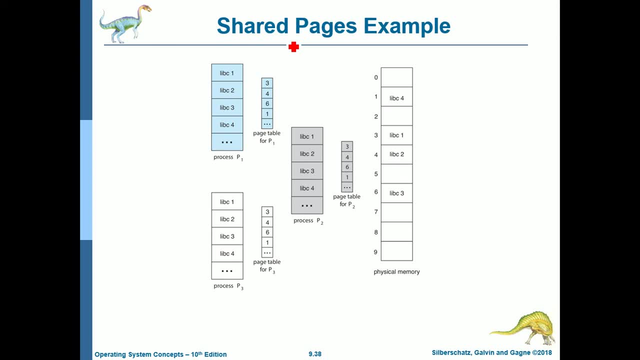 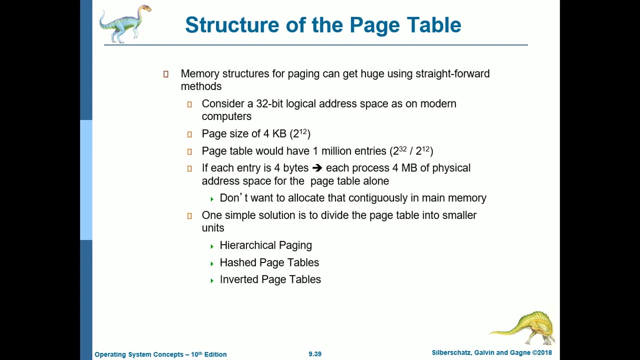 Location. That's the mechanism of shared pages, So that because they are sharing these pages, the address in the physical memory must all be the same. Okay, next is we have the structure of the page table, So memory structures for paging can get huge using straightforward methods. 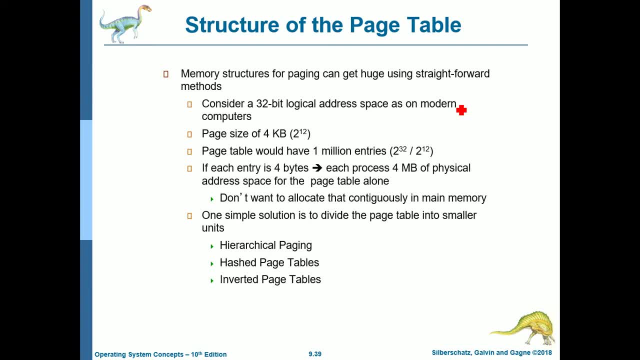 So consider a 32-bit logical address space, As on modern computers. So page size of 4 kilobytes, 2 raised to 12.. So for this page table would have 1 million entries. So we have 2 raised to 32 for the page number and 2 raised to 12 for the page offset. 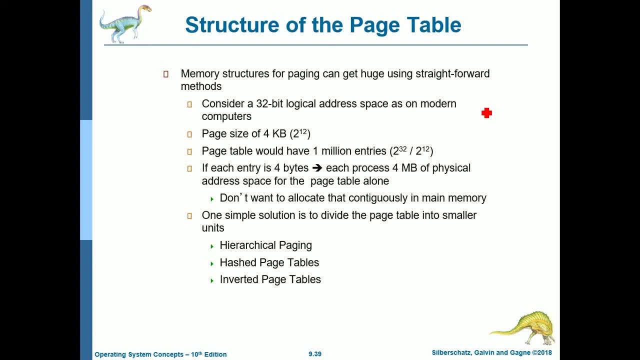 So if each entry is 4 bytes, each process 4 megabytes of physical address space for the page table alone. So don't want to allocate that contiguously in main memory because I think main memory will not be enough for other processes. 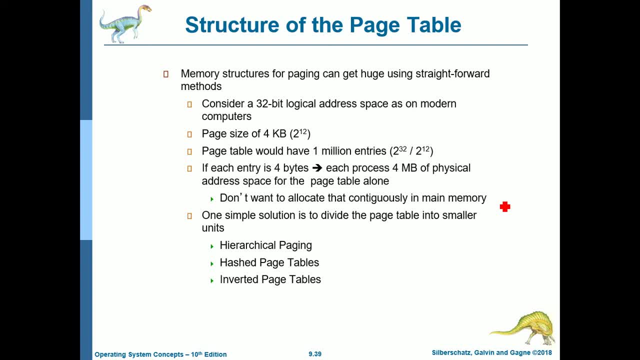 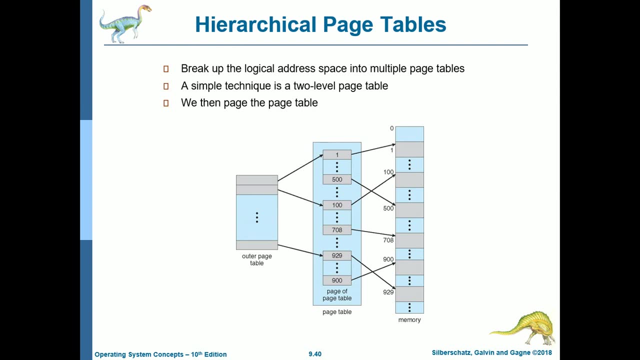 So one simple solution is to divide the page table into smaller units. So how we're going to divide that is by using hierarchical paging has page tables and inverted page tables. So first is we have hierarchical page tables, So break up the logical address space into multiple page tables. 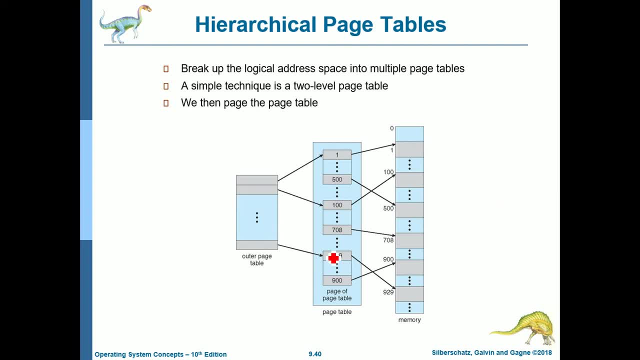 So a simple technique: a two level page table. so we have this one. so this table- outer page table- is, uh, divided, so we have three here, for an example, and then this will also be divided. so this is a two level page table. so so this one will have its own address, physical address, in memory. so we then page the. 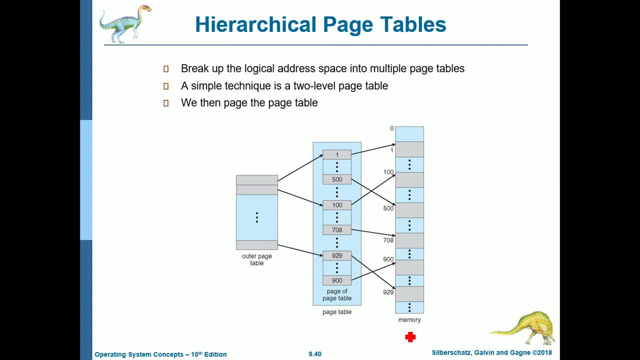 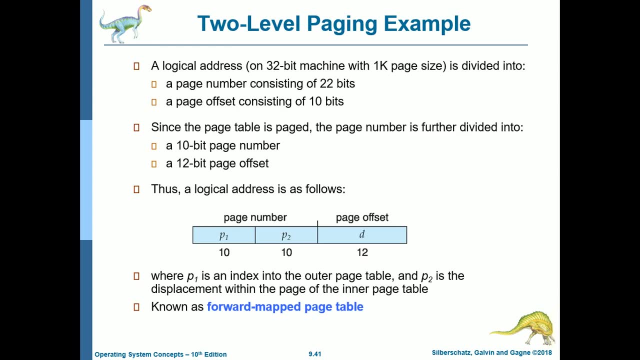 page table. so that's the hierarchical page table. this is a two level page table, so two level paging. example so a logical address on a 32-bit machine with one kilobyte page size is divided in two. okay, it can be a page consisting of 22 bits and a page offset consisting of 10 bits. so 22 plus 10. 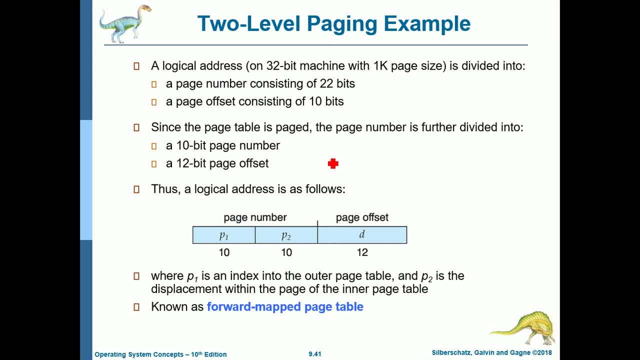 is equal to 32.. so since the table page table is page, the page number is further divided in two. so we have the 22 here is divided with 10 bit page number and we have a 12 bit page offset. so the logical address is as follows: for page number we have p sub 1 and then p sub 2. 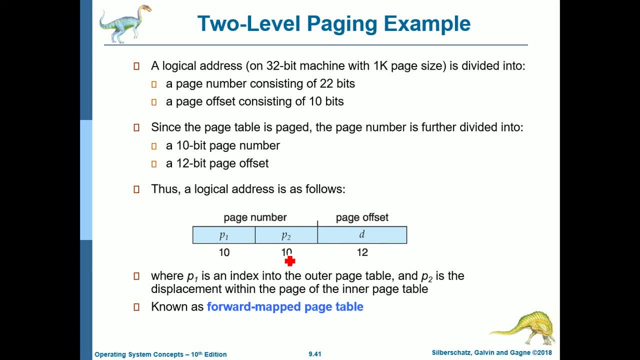 and then we have the page offset of 12.. so 10 plus 10 is equals to, is equals to. 20 plus 12 is equals. so where p sub i is an index into the outer page table, p sub 1 and then p sub 2 is the displacement. 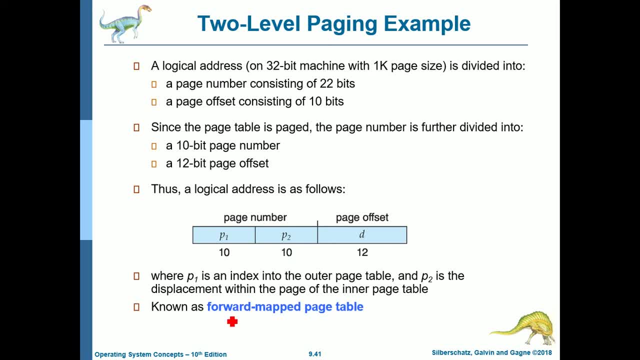 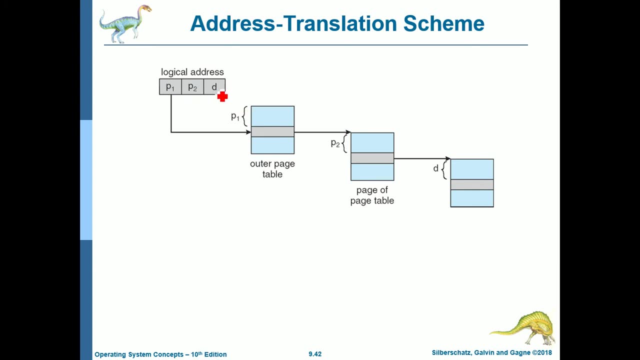 within the page of the inner page table, so this is known as the forward map page table. so this is the addressing for two level paging. so example for the address translation scheme: so we have p sub 1, p sub 2 as the page number and then d is for the page offset, so piece of one is said that it will access. 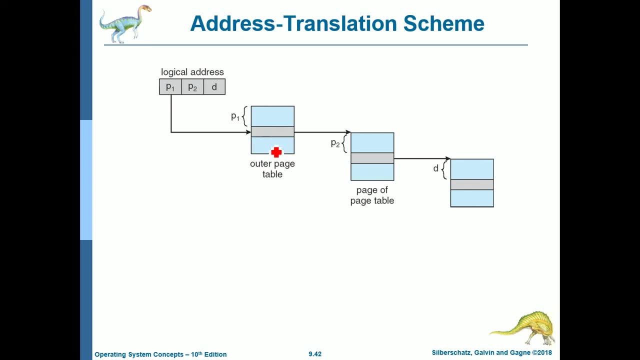 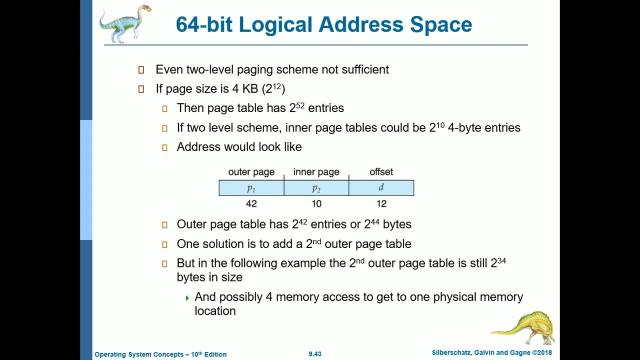 the outer page table. so after accessing the outer page table, then use p sub 2 to get the page of the page table, and then we are going to add the offset, okay. next is we have 64-bit logical address space, so even two level paging scheme is not sufficient. 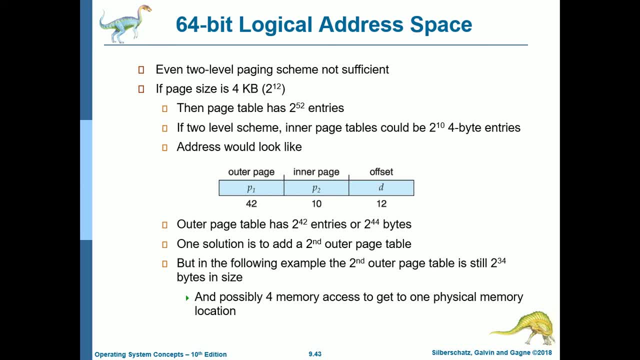 of course. so if page size is 4 kilobytes or 2 raised to 12, and page table has 2 raised to 52 entries, it's actually too much. so if two level scheme inner page tables could be 2 raised to 10, 4 byte entries, so the address would look like it's. 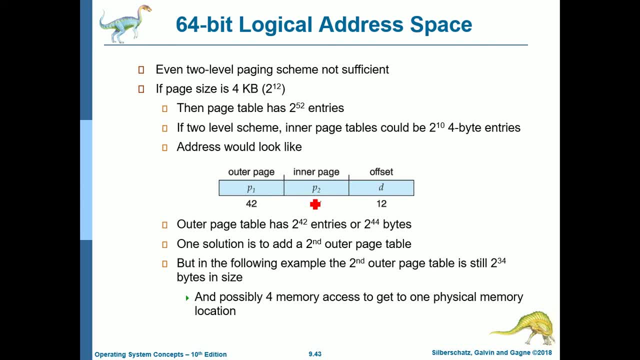 still actually big for the outer page for p, sub 1 is 42, inner page is 10 and then offset is 12. so 42 plus 10 we have 52. plus 12 is we have 64. so the outer page table has 2 raised to. 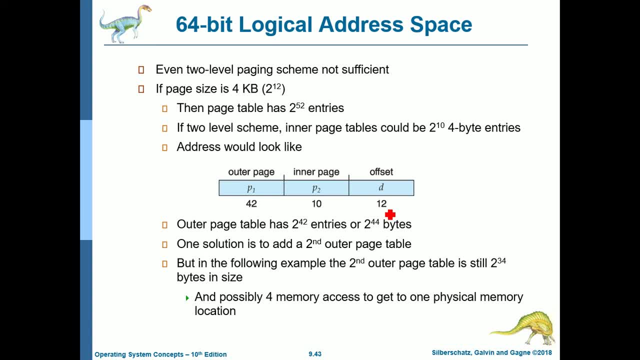 42 entries or 2 raised to 44 bytes. it's too big. so one solution is to add a second outer page table. but in the following example the second outer page table is still 2 raised to 34 bytes in size and possibly for memory access to get one physical memory location. 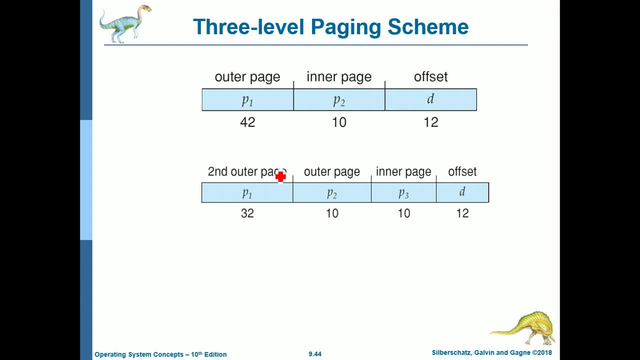 so this is the example. as it is said is, we have outer pages 42, then 10 and then 12 for 64-bit. so create another um for the second outer page table, but it's still big. for p sub 1 we have 32. 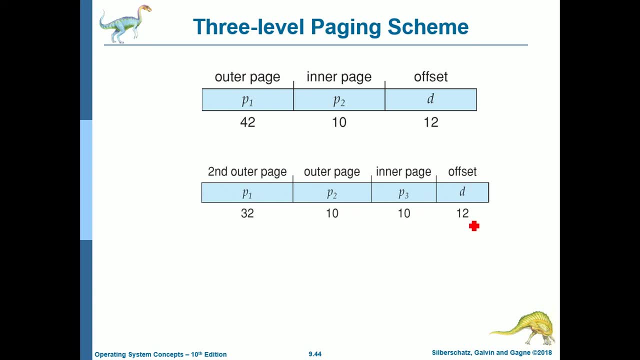 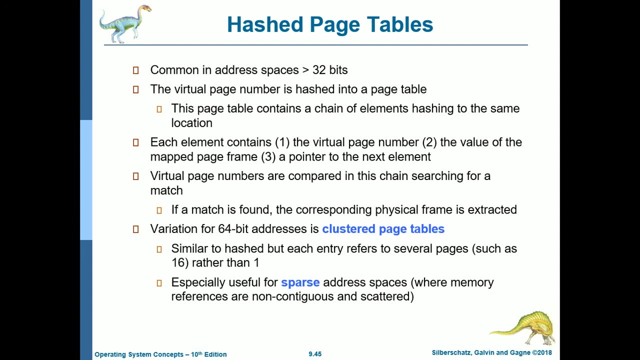 and then outer and inner page is just the same as 10, and then the offset is 12, so this will also be equivalent to 64-bit. so to solve that problem. so we are going to use hashed page tables. so common in address space is greater than 32 bits. so common in address space is greater than 32 bits. so common in address space is greater than 32 bits. 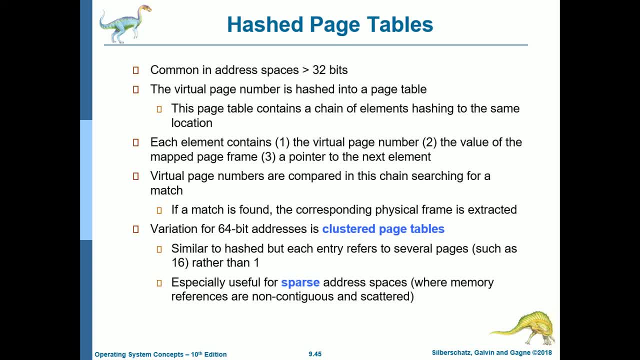 so the virtual page number is hashed into a page table. so this page table contains a chain of elements hashing to the same location. so each element contains number 1, the virtual page number, number 2, the value of the map page frame, and number 3, a pointer to the next element. so virtual page. 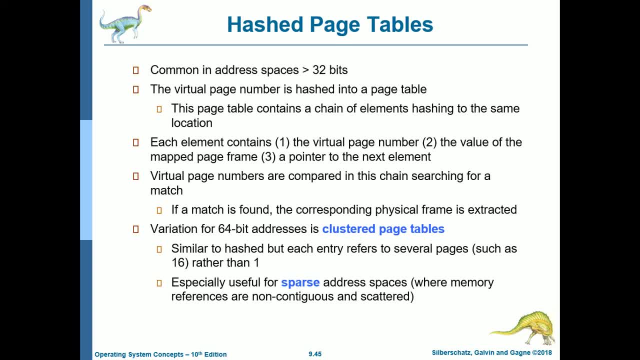 numbers are compared in this chain, searching for a match. if a match is found, the corresponding physical frame is extracted. so variation for select individual overall frame within a provided line are being found by cruelórrämer, case-emie and down value from the right hand side of useful and the left hand side of useful and smooth-Brown image. prepared text, go to front page, select neural data with animation, ar, suffer videos and dashboardality, and use the toolcaème to adapt the pace over to at least six examples. so this is all based on needs, as our Judge, jenny давайте easy to see, is written in table 7. 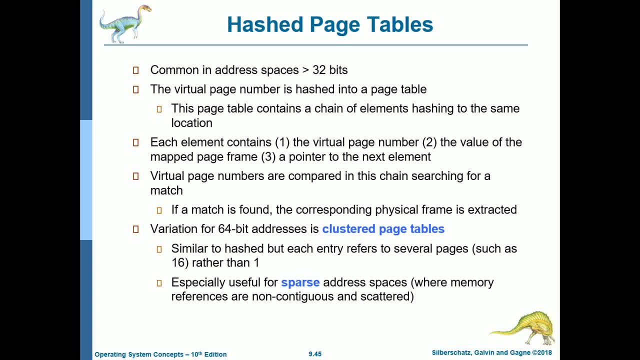 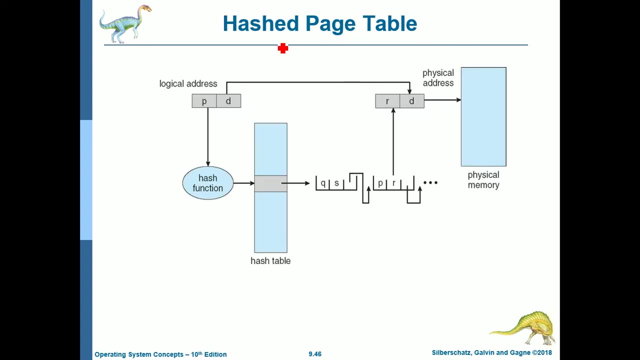 64-bit addresses is clustered page tables, so similar to the hashed, but each entry refers to several pages, such as 16 rather than one, and especially useful for sparse address spaces, or sparse meaning distributed address spaces where memory references are non-contiguous and scattered. so this is an example of a hashed page table, the illustration how it is done. 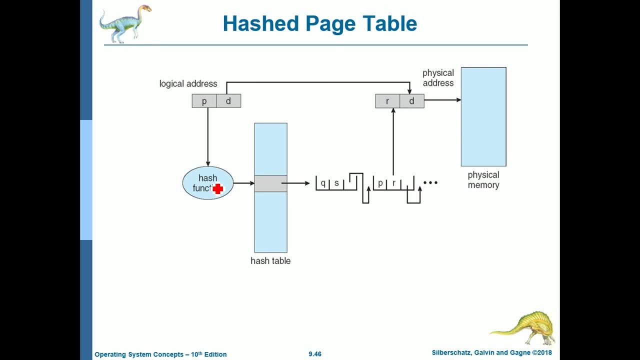 we have a logical address for the page number. it will access the. it has the hash function. it will access the hash table. so the hash table consists of values in linked list and if the value is found then it will be extracted from the hash table and then the page offset will be combined to get the. 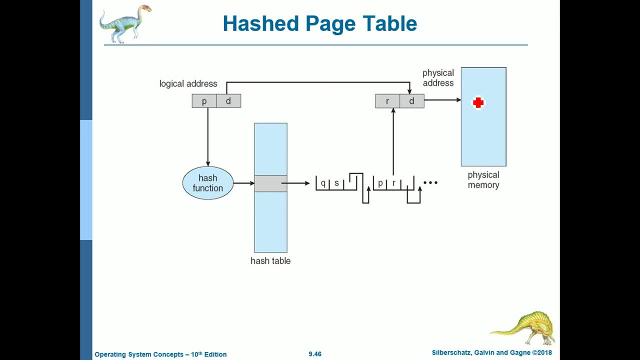 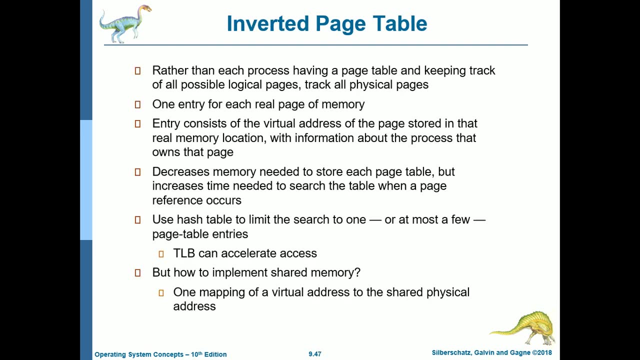 physical address corresponds to the physical memory. okay, next is we have another one. aside from hashed page table is we have the inverted page table. rather than each process having a page table and keeping track of all possible logical pages, track all physical pages. so one entry for each real page of memory. so entry consists of the: 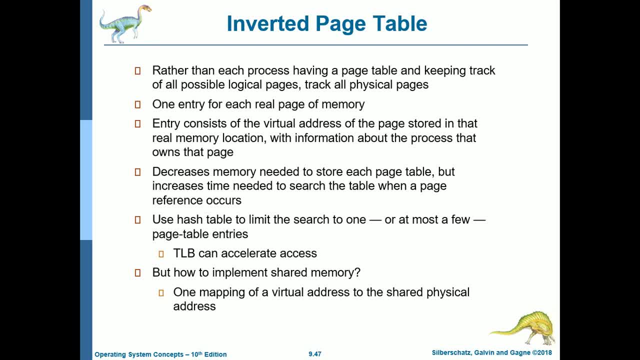 virtual address of the page stored in that real memory location with information about the process that owns that page. so this the advantage is: it decreases memory needed to store each page table but increases time needed to search the table when a page reference occurs. so use hash table to limit. 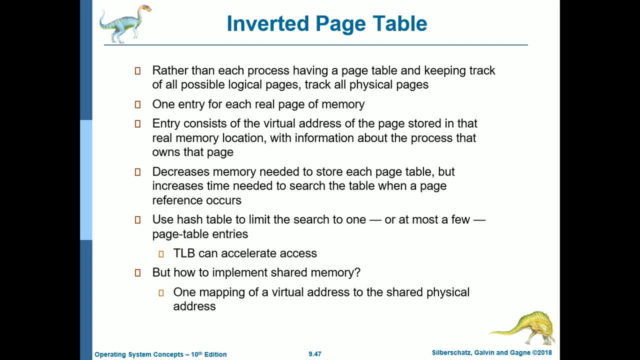 the search to one or at most a few page table entries, so tlbs can accelerate the access. so the question here now is: but how to implement shared memory? so the solution here is one mapping of a three entry using half route. Briefly, this video will show you how the pathetic 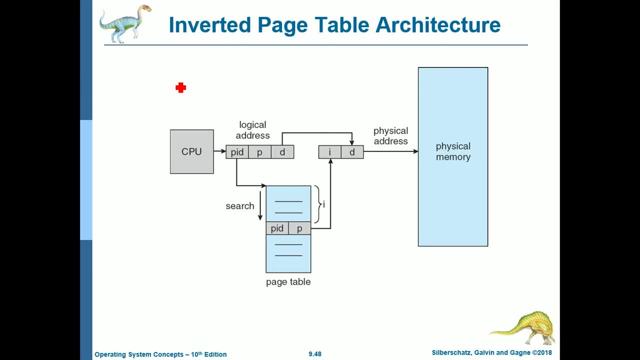 such as this video. so this is the, the illustration of the inverted page table architecture. you can also So the CPU, the logical address, so we have the PID 、 and then we also have the page number and the offset, so it will search the page table with the sen ID and the page number. 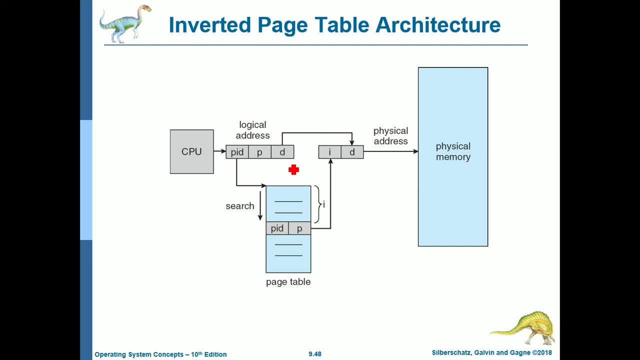 So if the value is located, so it will be extracted and then offset. the operation will be performed from this如果你 dia will arrive 있�, Sheriff is recordedня, But it'll managuh press and pull drugs E ". so the copy ". 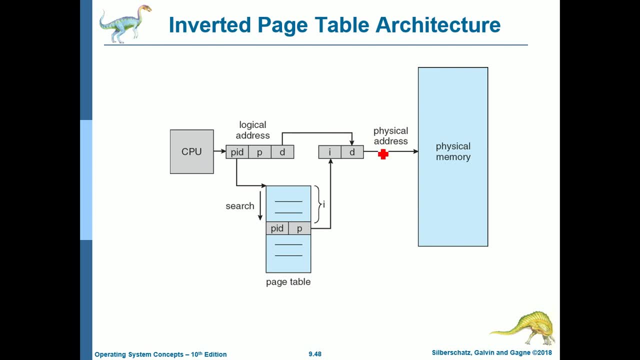 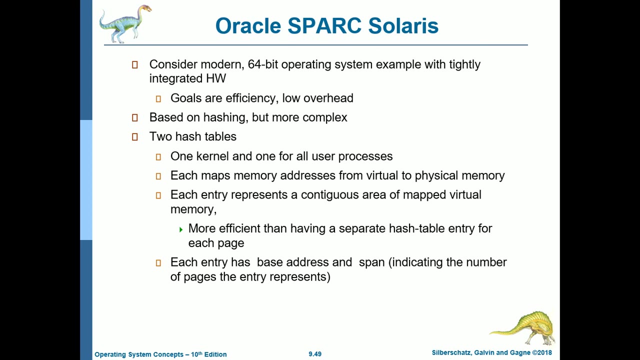 " page offset will be added, so it will produce the physical address corresponds to the actual address in the physical memory. okay, next is we have oracle, spark, solaris. so we have an example of an operating system here. how does the memory access or paging is happening in this operating system? so consider modern 64-bit. 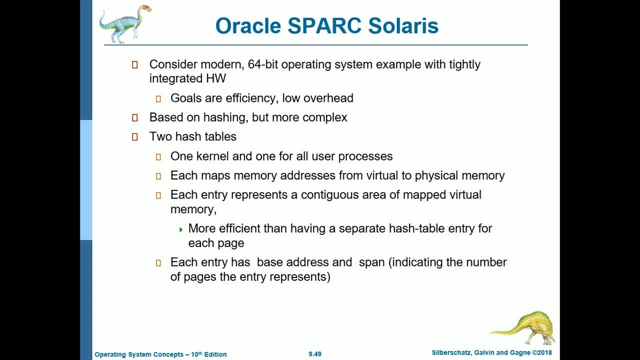 operating system example with tightly integrated hardware. so goals are efficiency and low overhead. so this is based on hashing, but more complex because it uses two hash tables, so one kernel and one for all user processes. each maps memory addresses from virtual to physical memory. each entry represents a contiguous area of mapped virtual memory, so more efficient than having a 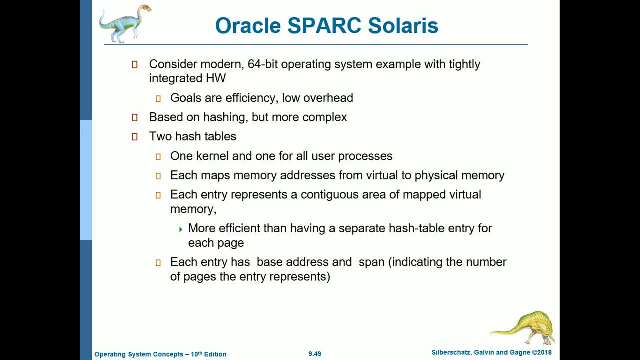 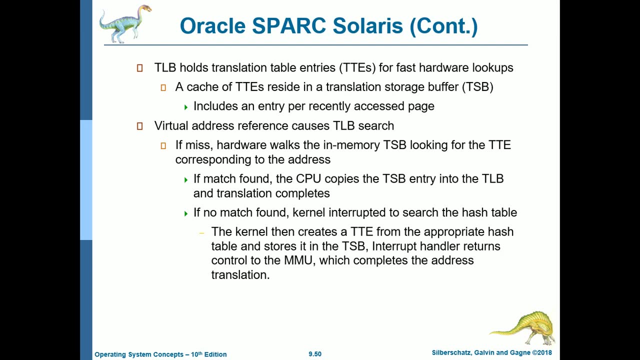 separate hash table entry for each page and then each entry has base address and span, or this indicates the number of pages the entry represents. so for oracle spark solaris it has a tlb that holds translation table entries, or ttes, for fast hardware lookups. so a cache of tte is resigned in a translation storage buffer or tsb. 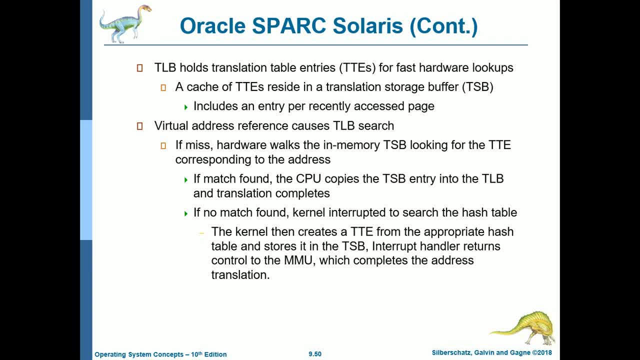 includes an entry per recently accessed page and then the tlb has a tlb that holds translation table entries. for fast hardware lookups and virtual address reference causes: tlb search: if it's a tlb miss, so hardware walks the in-memory tsb looking for the tte corresponding to the address. if match is found, the cpu copies the. 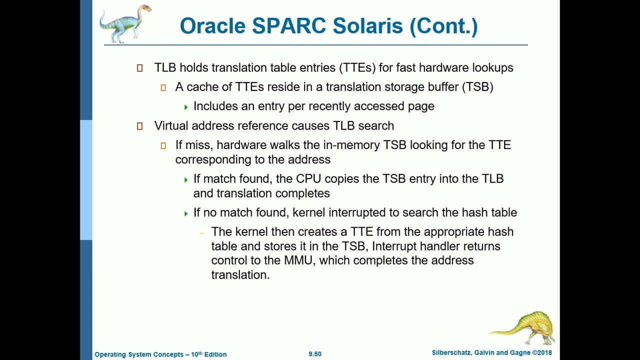 tsb entry into the tlb and translation completes. if no match is found, kernel interrupted to search the hash table. the kernel then creates a tte from the appropriate hash table and stores it in the tsb interrupt handler. handler returns the tte to the hash table and stores it in the tsb. 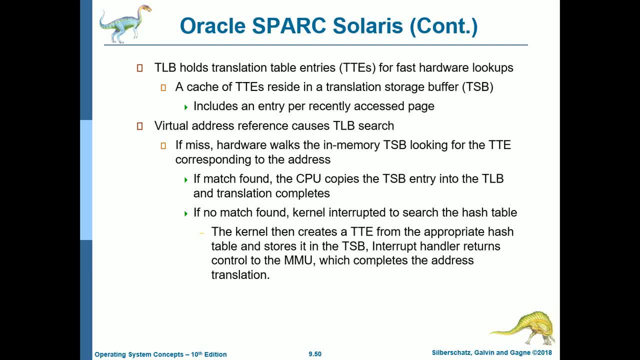 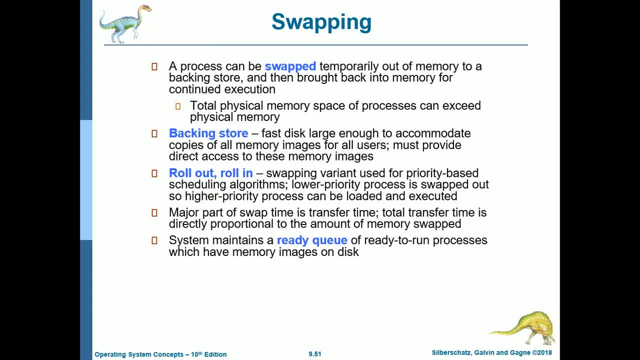 turns control to the mmu or the memory management unit, which completes the address translation. so that is for oracle, spark, solaris, okay. next is we have swapping, so a process can be swapped temporarily out of memory to a backing store and then brought back into memory for continued. 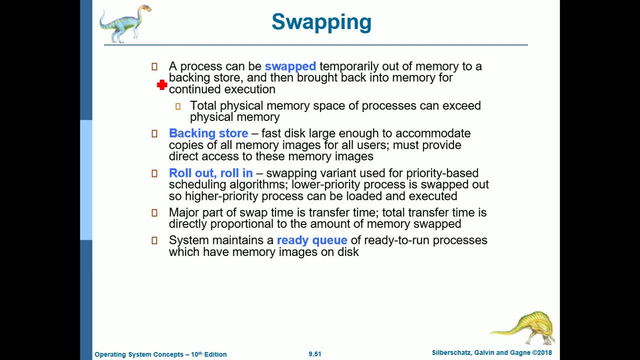 execution. so backing store- here is example- a hard drive. so total physical memory space of processes can exit physical memories. so that's why it needs to be swapped, because sometimes the physical memory space needed by the processes is bigger than the physical memory itself. so backing store, as i've said, can be a 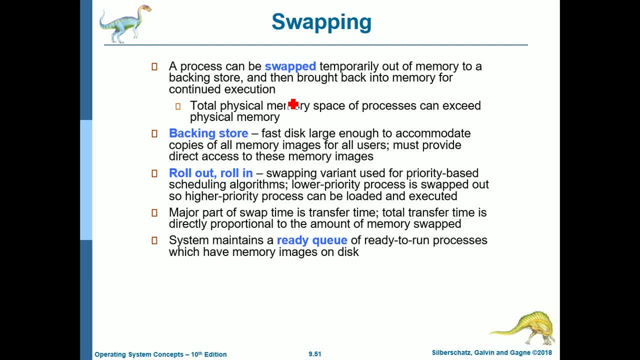 hard drive, so it's. a fast disk large enough to accommodate copies of all memory images for all users must provide direct access to these memory images. we have the roll out roll in, so this is also a swapping variant used for priority-based scheduling algorithms. lower priority process is swapped out, so higher priority process can be loaded. 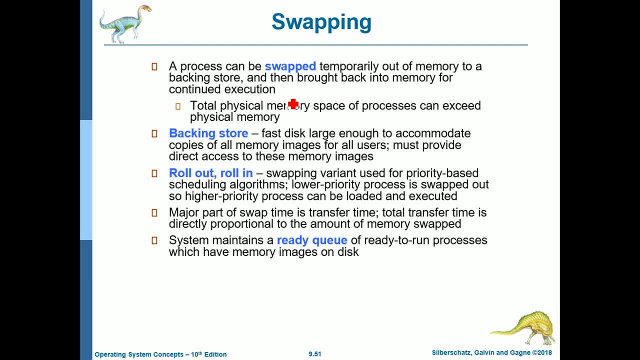 and executed. so that is why called the low priority process will be rolled out while the higher priority process will be rolled in. so that is the term of the swap, of the roll roll out, roll in, swapping variant. so major part of swap time is transfer time. total transfer time is directly. 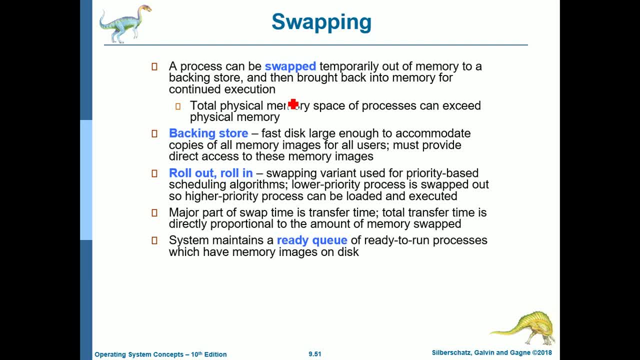 proportional to the amount of memory swap. of course, the amount of memory swap is proportional to the amount of memory swap, of course, if the physical memory space of the process is large, so the the transfer time is slower, just like, for example, in a real world scenario. for example, if you're 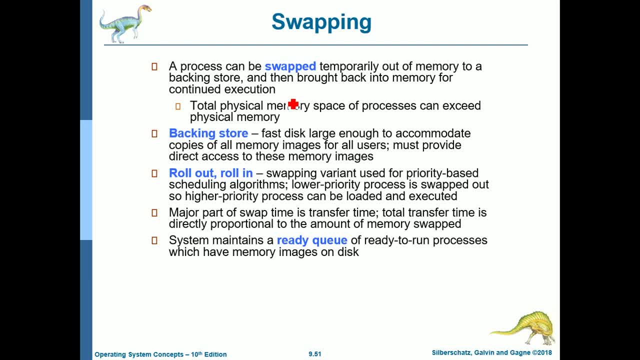 transferring one object from one location to another. if the object is light, you can transfer it faster because it's light. but if what? if you're going to transfers, for example, a refrigerator which is very heavy and you're going to transfer it to a refrigerator which is very heavy and you're going to 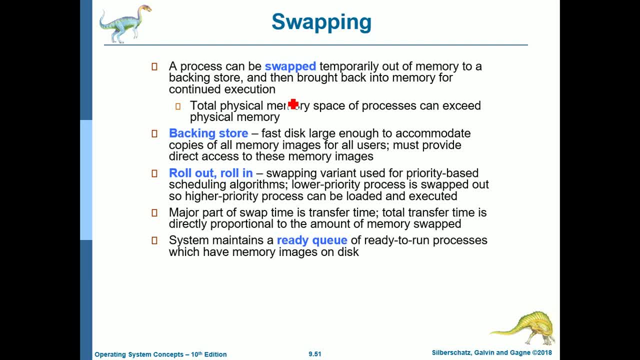 do it by hand or of course it will take time for you to transfer it from one location to another. so it's also with in in the computer system in main memory. so the total transfer time is always directly proportional to the amount of memory swap, and then system maintains a ready queue. 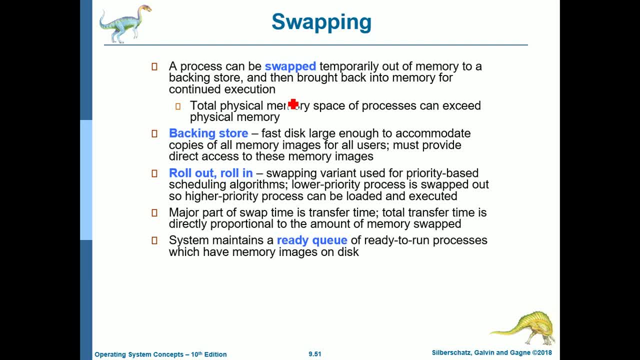 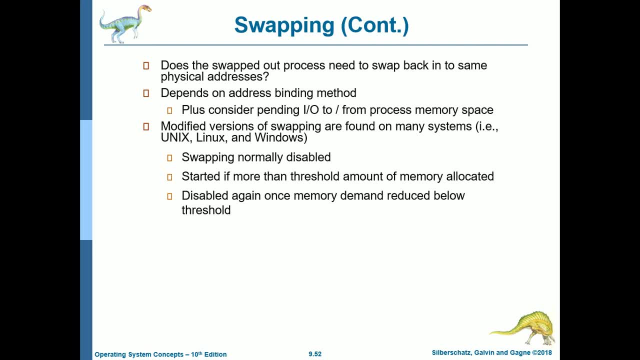 of ready to run processes which have memory images on disk. okay, so that's the swapped out. need to swap back in to the same physical addresses? okay? the answer to that question: it depends on the address binding method. so plus consider pending io to or from process memory space. 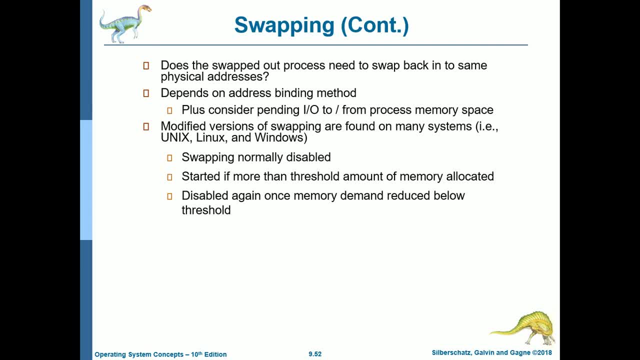 so modified versions of swapping are found in many systems such as unix, linux and windows. so swapping actually is normally disabled for the systems. it will only start if more than threshold amount of memory is allocated and then it will be disabled. If the memory space, the physical memory, is enough, then swapping is disabled. 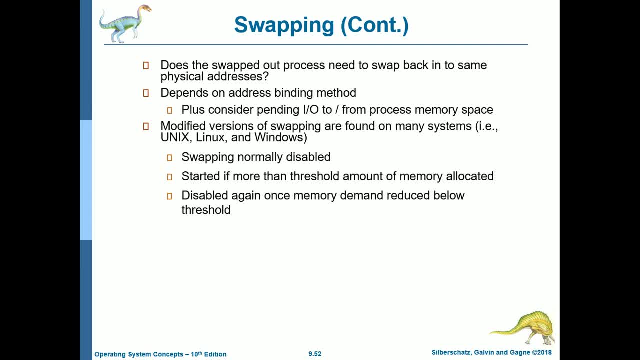 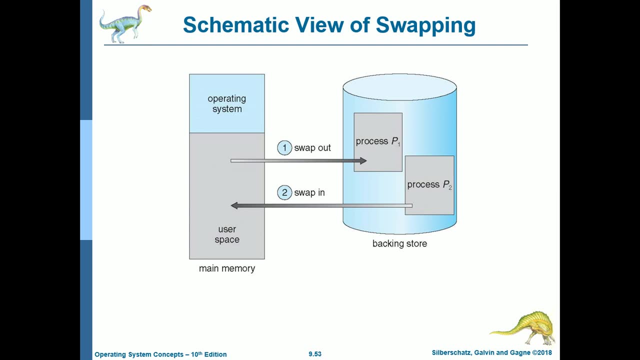 Yes, disabled. But if it exceeds the needed memory space, then it will be enabled. So it will be disabled again once memory demand reduced below threshold. So this is the schematic view of swapping. So again, this is our main memory, a fixed address for operating system, and then we have the user space. 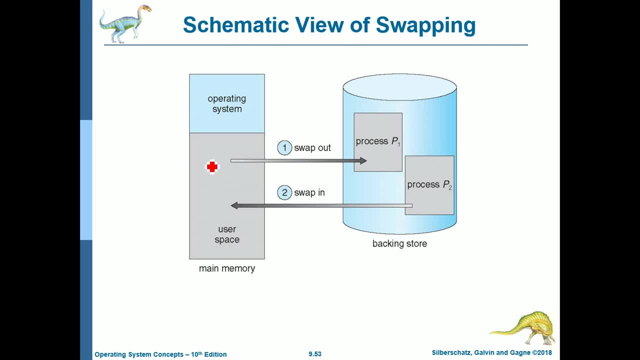 So, for example, process P1 is inside the main memory and process P2 is to be swapped in. So, for example- for a clear example, P1 is your R, You have opened the internet browser and then process P2- is you're going to type a Word document, for example. 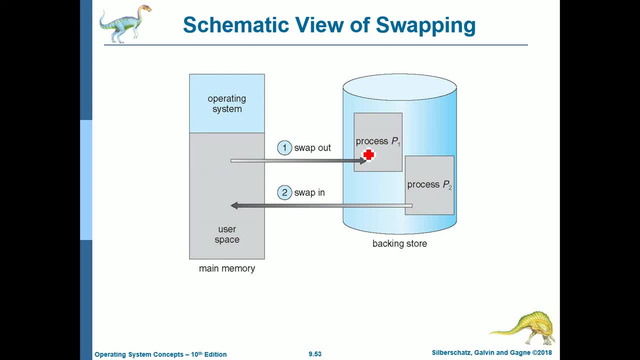 So while you're searching the internet, so process P1 is in memory. So then, after you've searched what you needed in the internet, then you decided to use the Word document. For example, you have a project that you are doing, you're researching for an article. 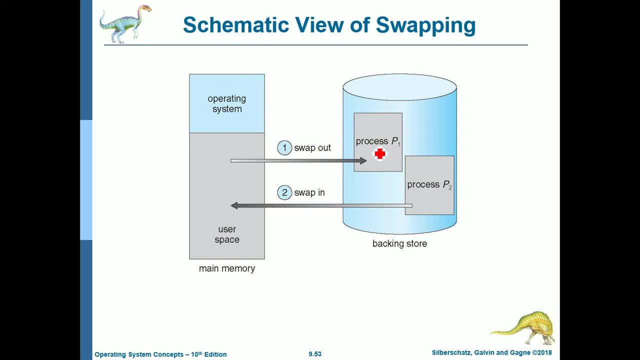 So from process P1,, in which you are doing your internet browsing, and then when you use your Word document, this is what happens. So process P1,, which is the internet browser, will be swapped out if the main memory space is not enough for the both of them. 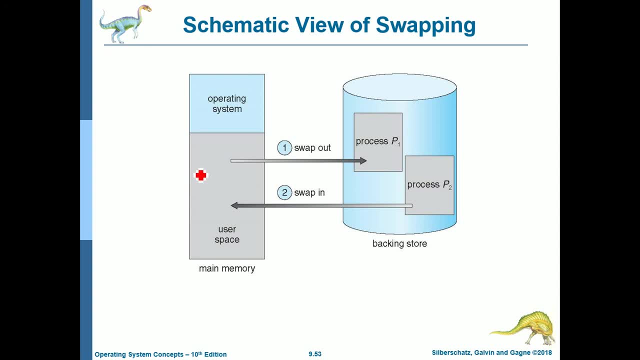 But of course, if it's enough, There is no swapping, that will happen, as indicated in the previous slide, that this is normally disabled. It will only be enabled if the space will not accommodate the process anymore. So again, let's go back with our example. 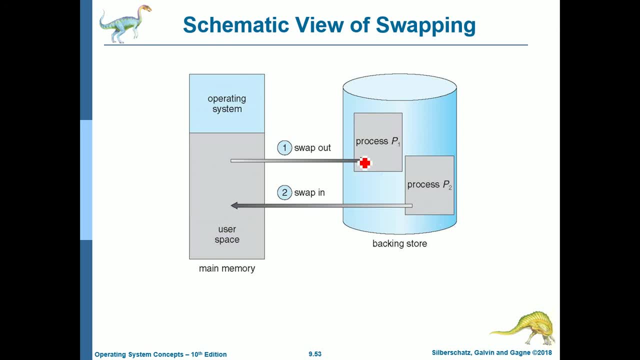 Once you're using your Word document. so since you're not using the internet browser for researching, so this will be swapped out. process P1.. And then your Word processor. since you're already typing or you're doing your project, so this will be swapped in. 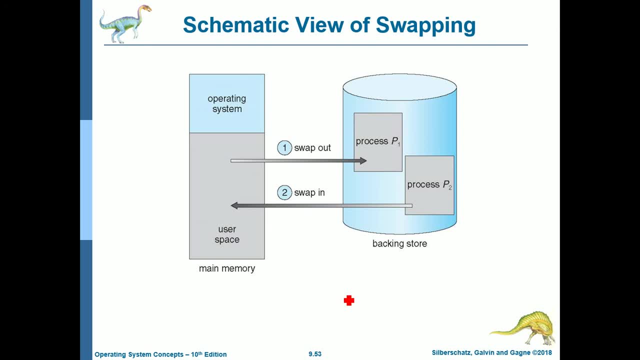 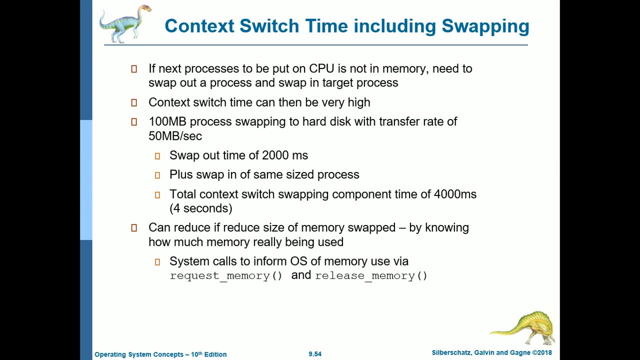 So that is the schematic view of swapping an example. Okay, next is we have the context switch time including swapping. So if next processes to be put on CPU is not in memory, you need to swap out a process and swap in target process. 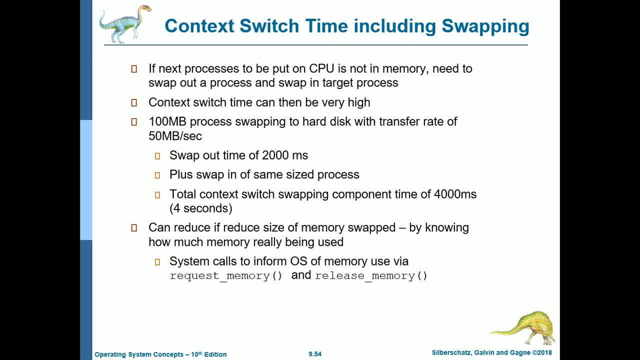 So this is the schematic view of swapping. So if next processes to be put on CPU is not in memory, need to swap out a process and swap in target process. So context switch time can then be very high. So we have 100 megabyte process swapping to hard disk with transfer rate of 50 megabytes per second. 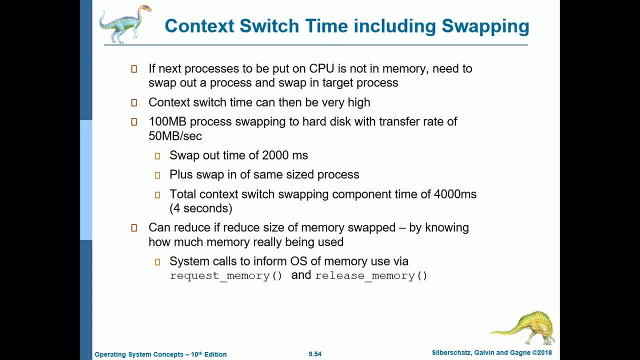 So swap out time is 2000 milliseconds, Okay. and then we have plus swap in of same size process. So total context switch swapping component of 4000 milliseconds- Okay- then can reduce size of memory swap by knowing how much memory really is being used. 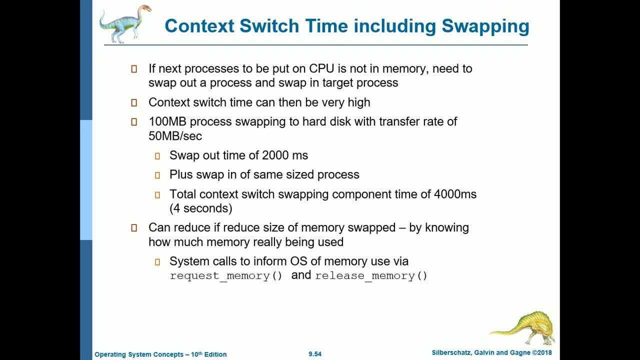 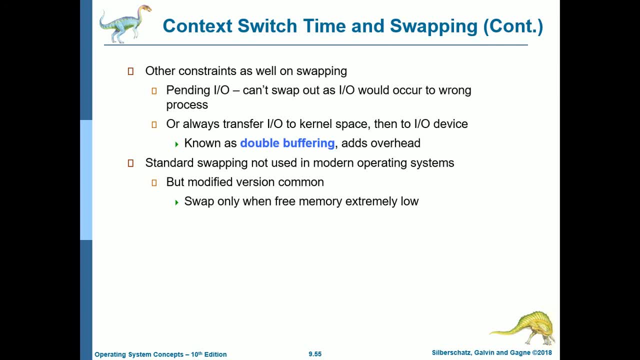 Okay, Okay, Okay, Okay. So pending input output can swap out as IO would occur to wrong process. So always transfer IO to kernel space, then to IO device, So known as double buffering. adds overhead. So double buffering is the copying of data twice, such as from a device to the kernel and then from the kernel to a process address space or the. process address space. So double buffering is the copying of data twice, such as from a device to the kernel and then from the kernel to a process address space or the process address space or the. So double buffering is the copying of data twice, such as from a device to the kernel and then from the kernel to a process address space or the. 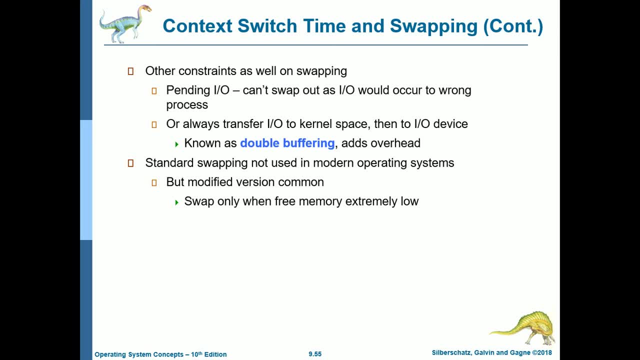 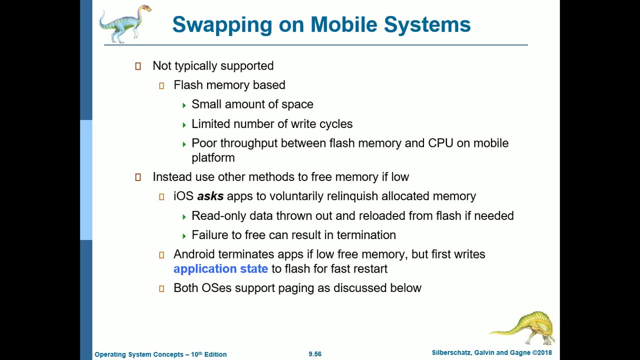 of two buffers to the couple producers and consumers. so standard swapping not used in modern operating system, but modified version common. so, as it is said, swap only when free memory extremely low. and then is there a swapping on mobile systems, in our smartphones or in our cell phones. so swapping is typically not supported. so because it is flash memory based and it has 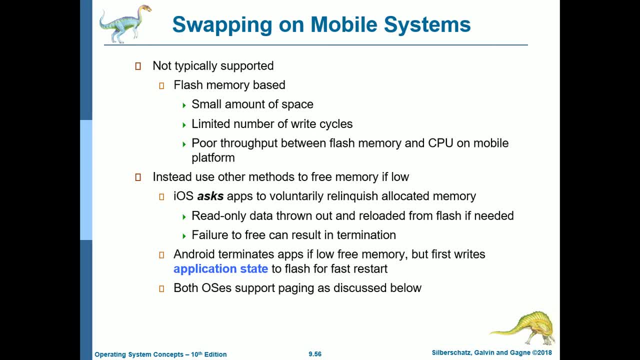 only a small amount of space, limited number of write cycles, so poor throughput between flash memory and cpu on mobile platform. so instead use other methods to free memory flow for ios. ios ask apps to voluntarily relinquish allocated memory. read only data thrown out and reloaded from flash if needed. failure to free can result in termination. so while android terminates apps, 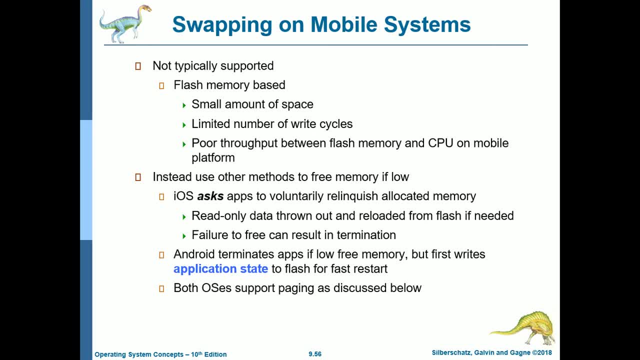 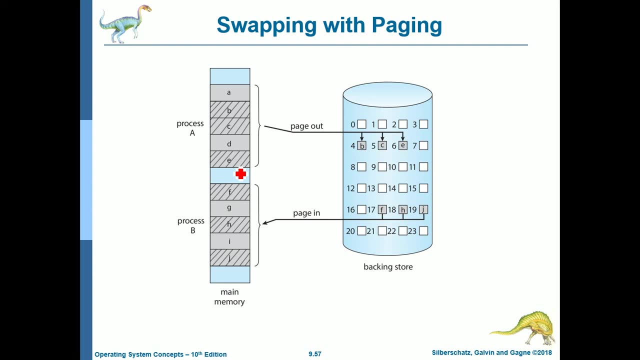 if low free memory but first writes application state to flash for fast restart. so both oss, ios and android supports paging as discussed, so we have the swapping with paging. so for example, process a has b, c and d page, so it's not really the process but the page. so this will be paged out. 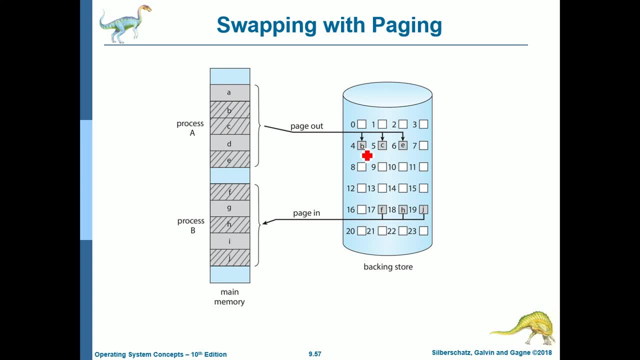 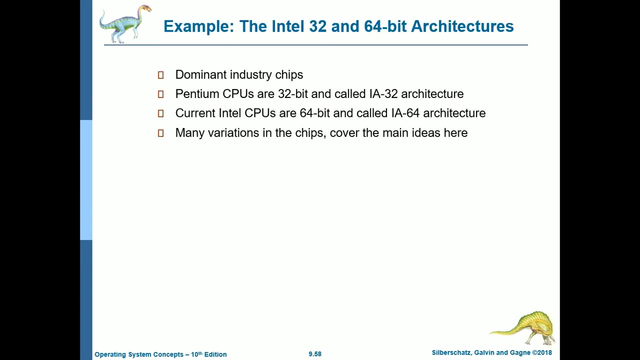 and it will be stored in uh backing store and then the corresponding, since this is three, that is needed by process b, so it will be paged in in the main memory. so next is we have, example, the intel 32 and 64-bit architectures. so these are the dominant. 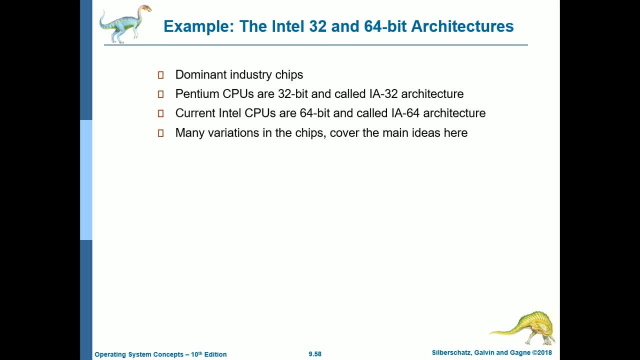 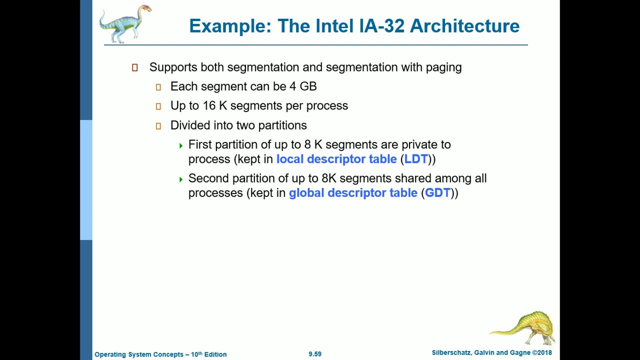 industry chips of intel and pension cpus are 32-bit and called ia32 architecture. so currently intel cpus are 64-bit and cold ia64 architecture. so many variations in the chips cover the main ideas here. so for the intel, ia32 architecture supports both segmentation and segmentation with. 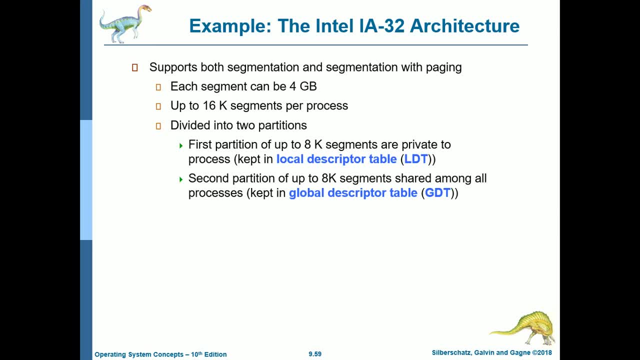 paging. each segment can be 4 gigabyte. up to 16 kilobyte segments per process and these are divided into two partitions. so first partition of up to eight kilobyte segments are private to process and it is kept in local descriptor table or the ldt. 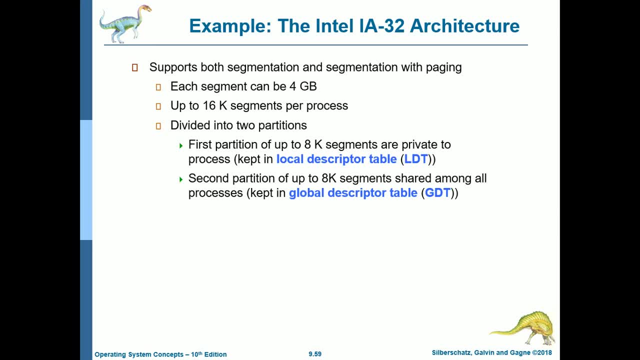 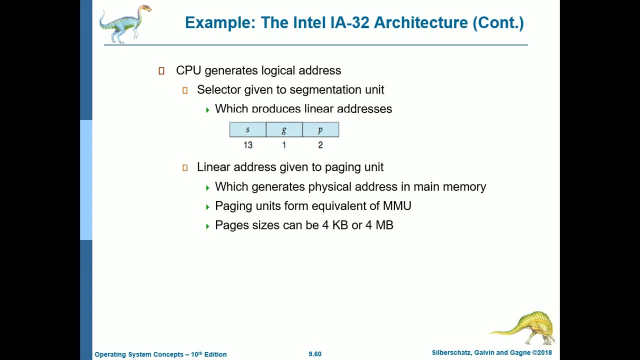 and then we also have the second partition: up to eight kilobyte segments shared among all processes. since this is shared, or rather all shared, these are kept in the global descriptor table, or the gdt. so cpu generates local, a logical address, rather so selector, given to segmentation unit, so which this 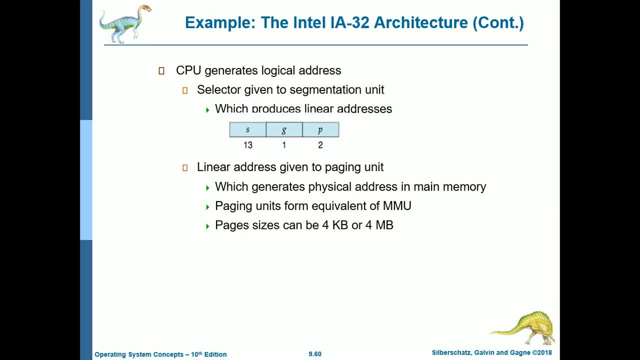 which produces linear addresses. so for here we have s, so s is segment number, so g, it's either a local, from the, the location of a local descriptor table, or a global descriptor table, and then p is for protection, so linear address given to paging unit which generates physical address in main. 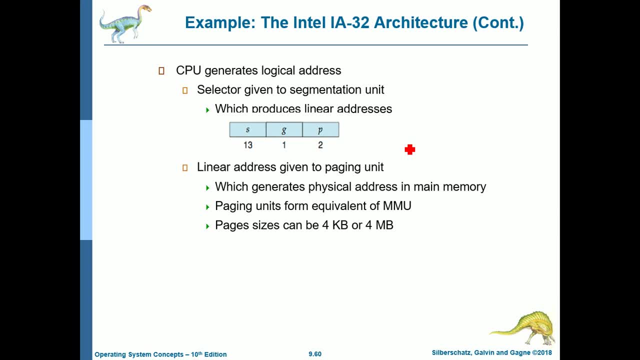 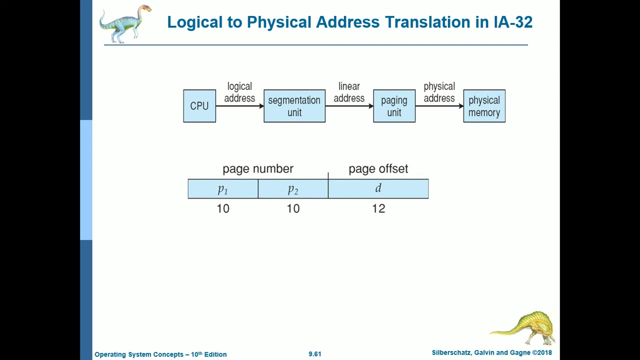 memory, so paging units or form equivalent of main memory management unit, and page sizes can be four kilobytes or four megabytes, so ia32. so the address is a 16-bit linear address. okay, next is we have logical to physical address translation in ia32. 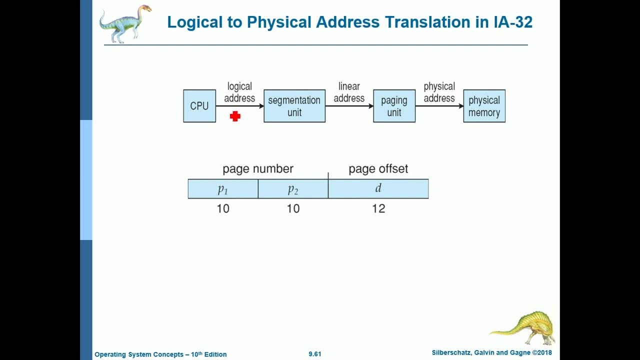 so for the cpu it will derive the logical address and then it will undergo process in the segmentation unit and then it will conceive a logical address after segmentation unit and then it will yapıyor the audit in the segmentation unit and would punching in the segmentation unit. so 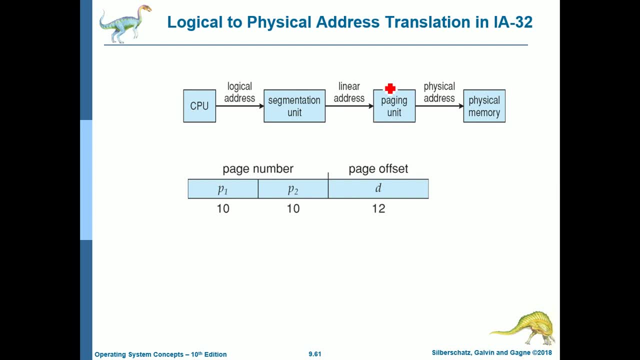 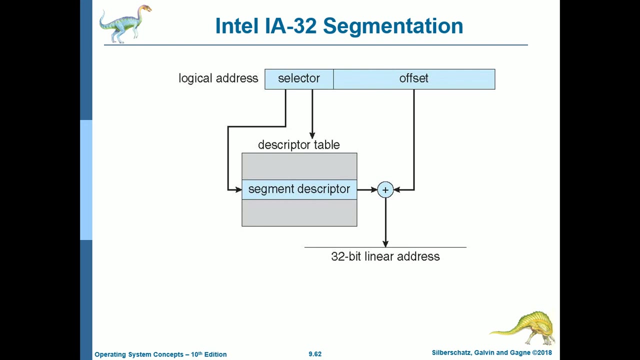 produce the linear address and then it will undergo under the paging unit and it will produce the physical address and it will be the corresponding address in the physical memory. okay, next is we have the intel i832 segmentation. so our logical address is composed of selector and offset. so this selector points to the description table and the actual location of 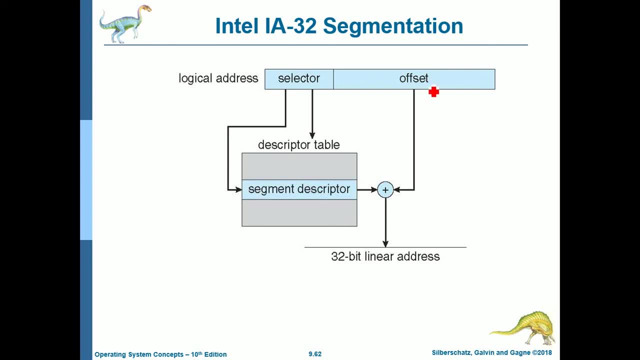 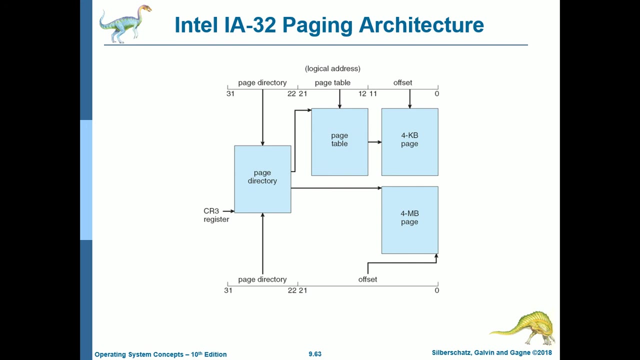 the segment descriptor, and then this will be combined into the offset, and then the offset is a 32-bit linear address. okay, there we have the intel ia32 paging architecture. so we have. so so we have the 10 higher order bits, references and entry in the outermost page table, which ia. 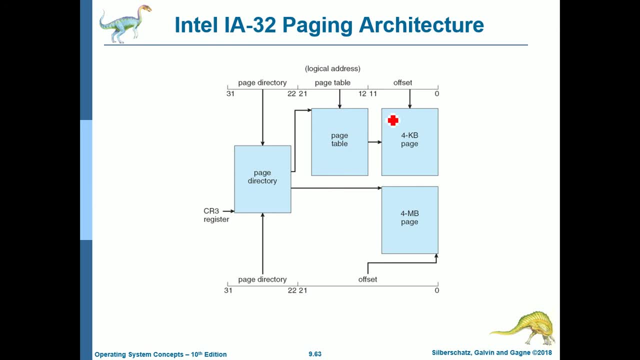 32 terms the page directory. so we have this one. so from 0 to 11, this is the offset. then from 12 to 21, it will uh points to the page table, and 22 to 31- this is the 10 high order bit- references uh, an entry in the outermost page table. so this is the. 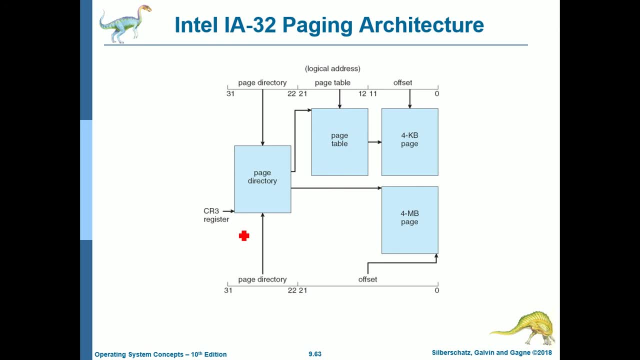 one and then our cr3 register points to the page directory for the current process, and then the page directory points to the inner page table. this is the inner page table, that is, that is what indexed by the contents of the innermost 10 bits in the linear address. so this is: 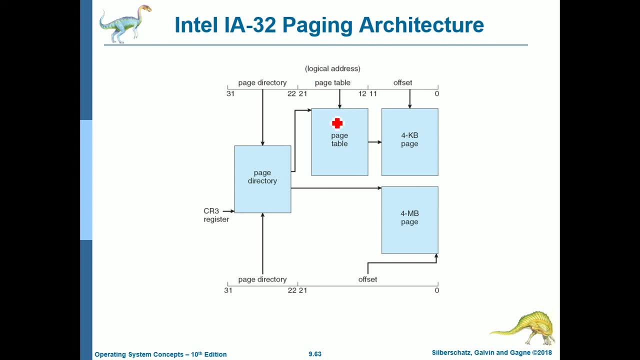 the 10 bits. okay, then finally the low order, bit 0 to 11, which is the offset, um. this refers, of course, to the four kilobyte page, pointed to the page table, and also, aside from the page directory, pointing to the page table, it also has also points to the 4mb page. okay, 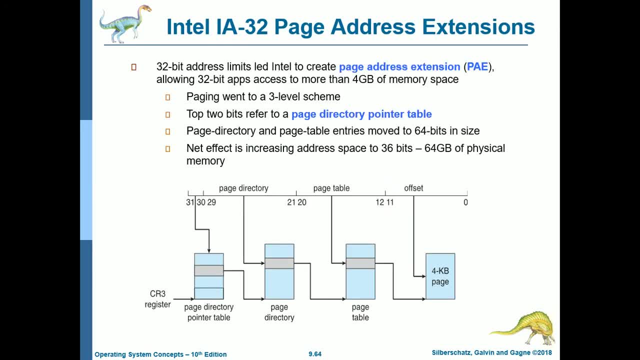 so next is we have the intel ia 32 page address extensions. so 32-bit address limits led intel to create the page address extension, or the pae. okay, allowing 32-bit apps access to more than 4 gigabyte of memory space, because for 32 bits it can only access 4 gigabyte of. 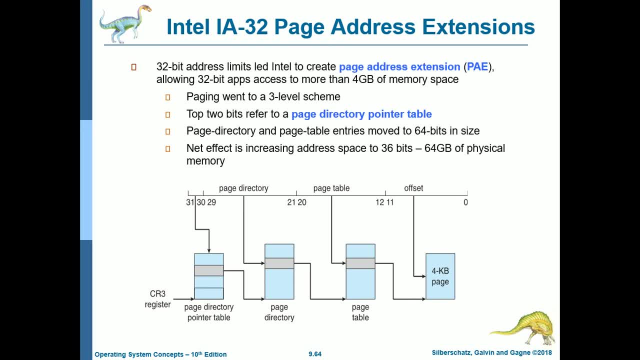 memory space. but because of page address extension it increases its limit that it can access more than 4 gig gigabyte of memory space. so paging went to a three-level scheme. so top two bits refer to a page address extension and it can only access 4 gigabyte of memory space. so paging went to a 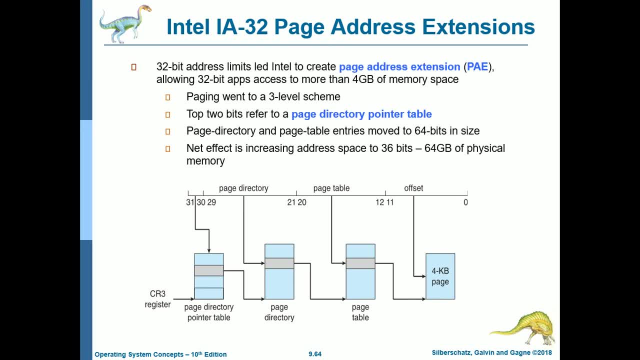 page directory pointer table and then page directory and page table entries move to 64 bits in size and the net effect is increasing other space to 36 bits as to 64 gigabits of physical memory. so from 32 it become 36 and then it can access an additional or a bigger size which 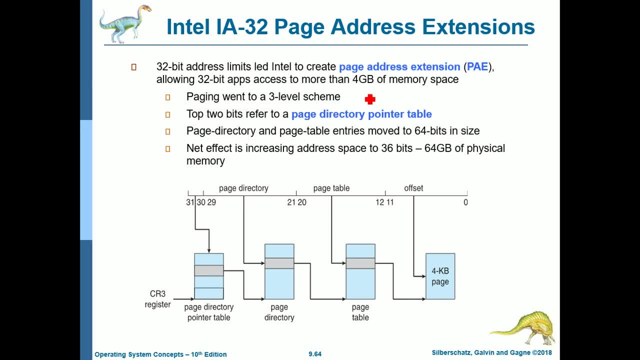 is 64 bits of physical memory compared to 4 gigabits- gigabytes rather- of memory space. so for again it's a 32 bits. so 0 to 11 is the offset, 12 to 20 is the page table and 21 to 30 is the 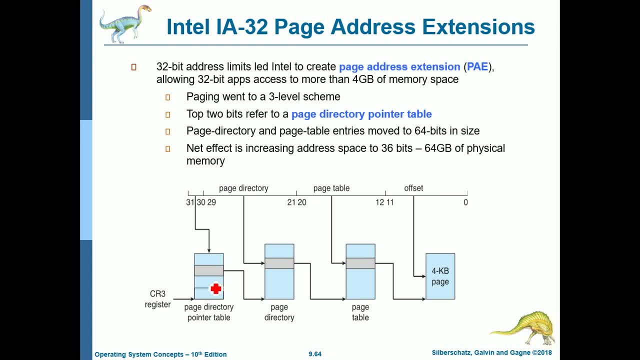 page directory and then we have one byte here for the page directory pointer table. so this also illustrates a pae system with four kilobyte pages. so also pae support supports two megabyte pages. okay, so again we have the cr3 register. points to the page directory table and then this points to the 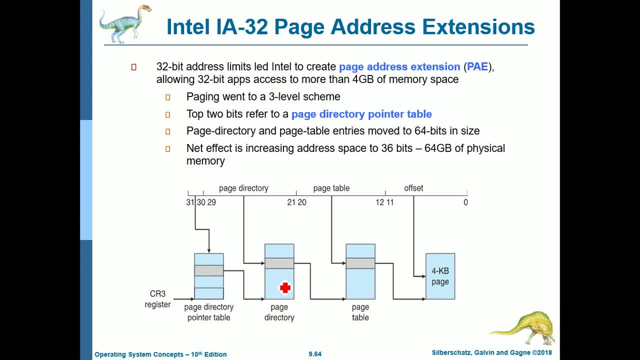 page directory and then this address is for the page directory, and then page directory points to the page table. so this one, this address, this bits, is for the page table and of course we have a four kilobyte page combining for the offset and the values of the. 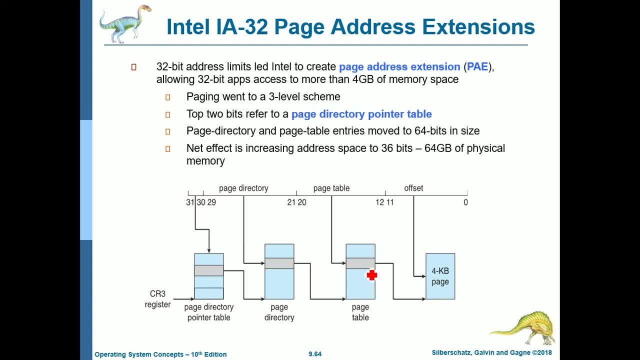 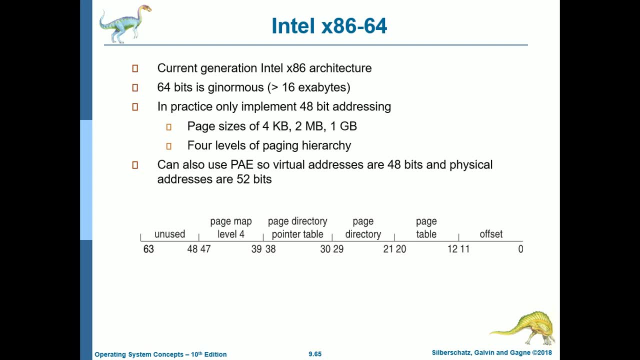 page directory and the values in the page table. okay, next is we have the intel x86 64. so current generation intel x86 architecture, so 64 bits, is greater than 16 exabytes. so in practice only implement 48 bit adjusting so page sizes can be of four kilobytes, two megabytes and one gigabyte because it's two bits. 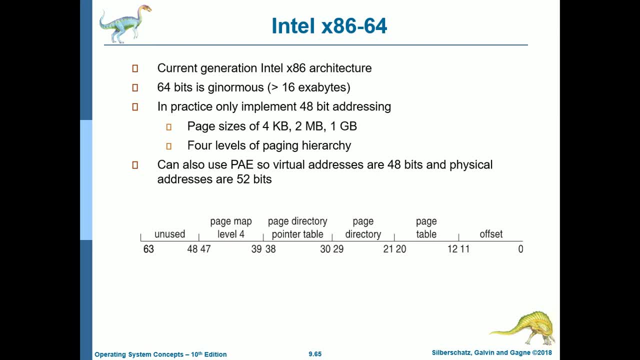 and then it has a four, four levels of paging hierarchy, can also use pae. so virtual addresses are 48 bits and physical addresses are 52 bits. so again, this is the composition of its 64 bit address. so we have offset for 0 to 11. 12 to 20 bits is the page table. 21 to 29 is the page. 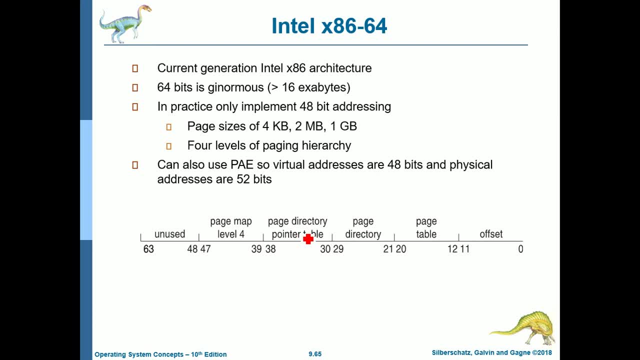 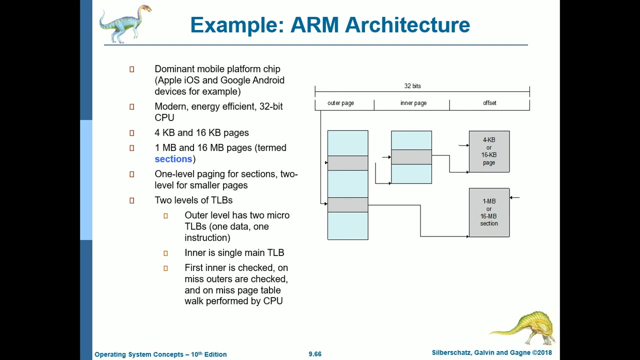 directory 30 to 38 is the page directory pointer table and 39 to 47 is we have the page map level 4 and of course it is said that in practice only implements 48 bit addressing, so 48 to 63 is unused, okay. another example is we have the arm architecture, so dominant mobile platform chip. 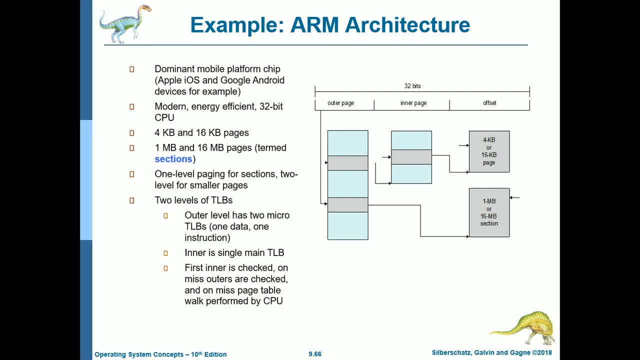 which is used by apple, ios and google android devices, for example. it is modern, energy efficient CPU. it uses 4 kilobyte and 16 kilobyte pages, and then we also have 1 megabyte and 16 megabyte pages for sections. so one level paging for sections, two level for smaller pages. so it has two levels of 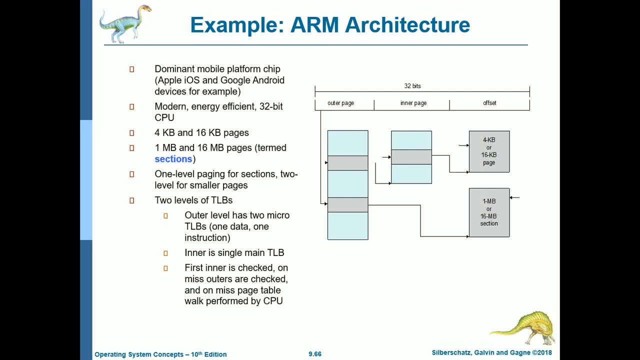 tlbs. so outer level has two micro tlbs, one data and one instruction, and then inner is a single main tlb and then first inner is checked and then the other inner is checked, and then the other inner is checked on miss outers are checked and on miss on page table walk performed by cpu. so it's a 32 bit.